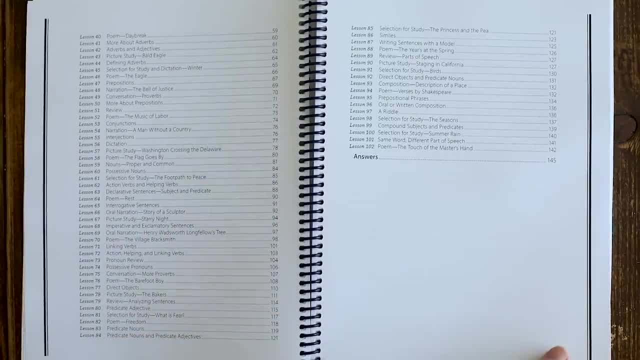 a summary, a paragraph summary, about it. They do memorization, There's poetry, there's grammar, there's picture studies. there's all sorts of different things involved. It even goes into some composition as well, And so it's just a very gentle light on language arts curriculum that you 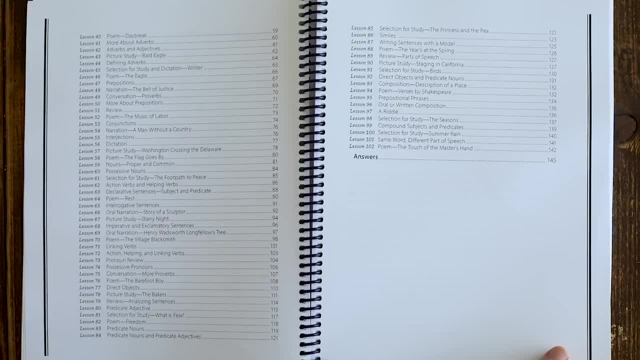 can use alongside really anything else that you are doing, And I love, love, love the approach of this. So let's take a look inside some of the days So you can see how they're incorporated into their. So let's take a look inside some of the days so you can see how they're incorporated into their. 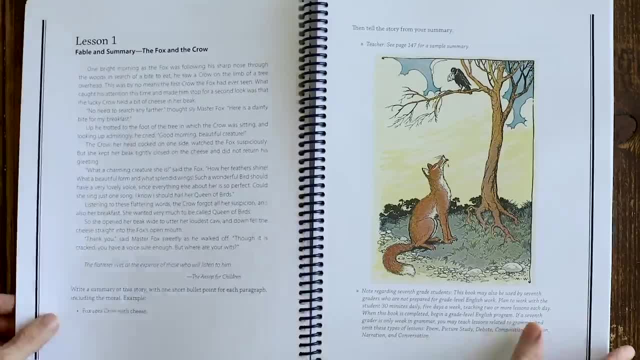 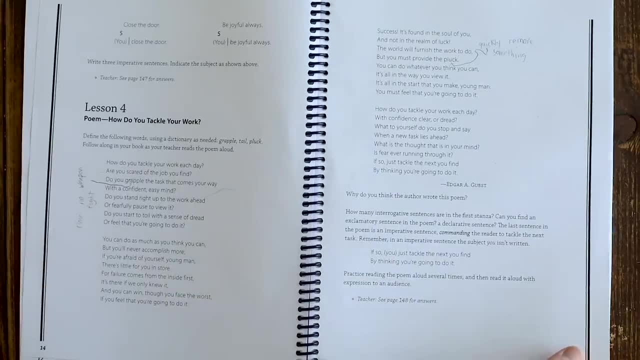 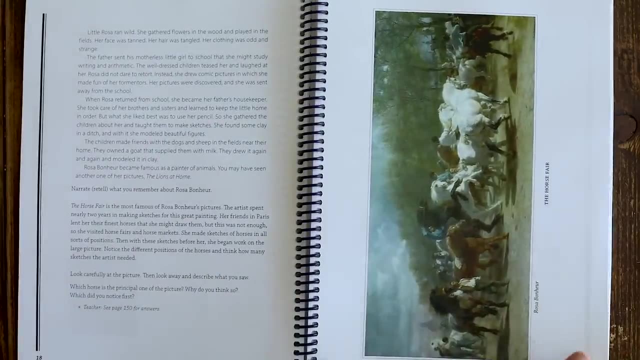 you can see how it is laid out. So they're doing reading aloud, There's poetry, picture studies. I love the layout of this. I love that the lessons are relatively short. They're easy to do, They're not too overwhelming And, like I said, this is the grade six level. So I think that for this level, 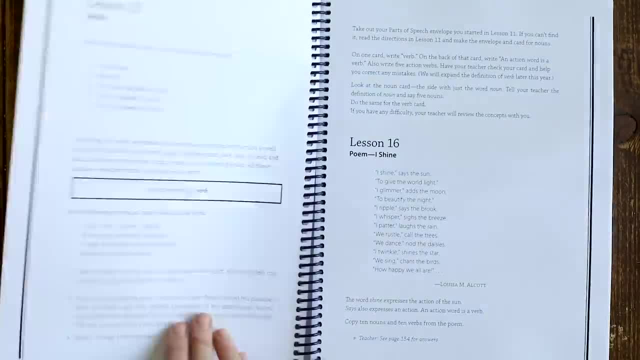 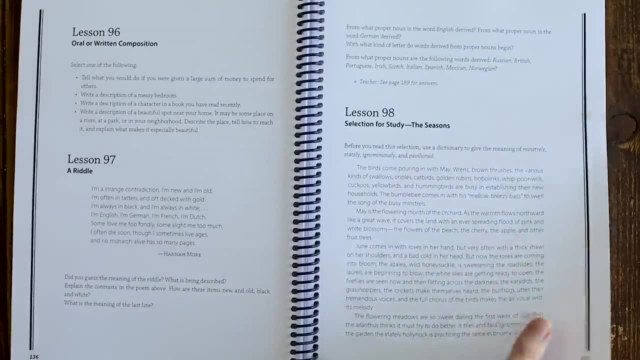 it is definitely not too much And it's just that reinforcement that they would be doing on a. I personally think language lessons for today is phenomenal And it's relatively inexpensive. If you go over to their site and click on language arts, you'll see them all listed there. 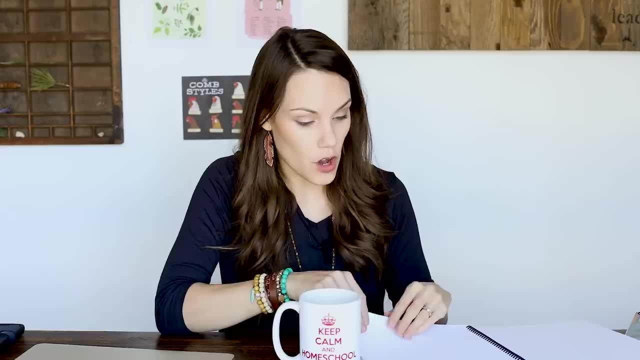 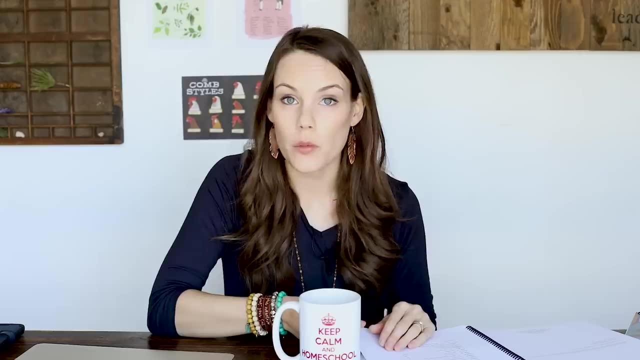 Now let's take a look at writing skills. for today We're going to look inside the table of contents. This is the level C I'm showing you, And this is actually an adaptation of writing strands. You may be more familiar with writing strands. There is quite a bit of it out there and some different. 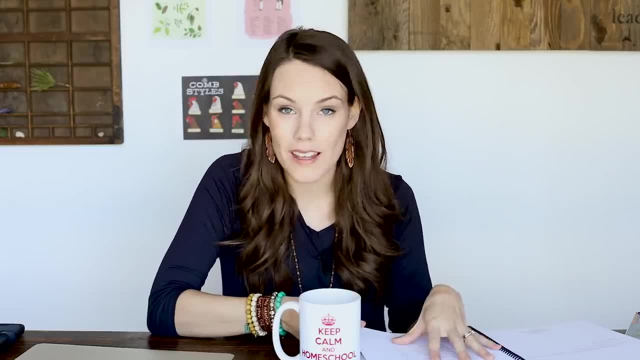 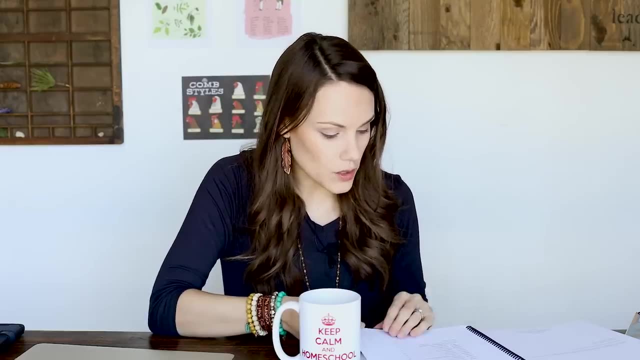 companies have also kind of put their spin on it. So My Father's World also has done the same thing. They want to put their spin on writing strands. So that is what this is, And so you'll see the different units that are included, And this is giving them really instructional how to write. 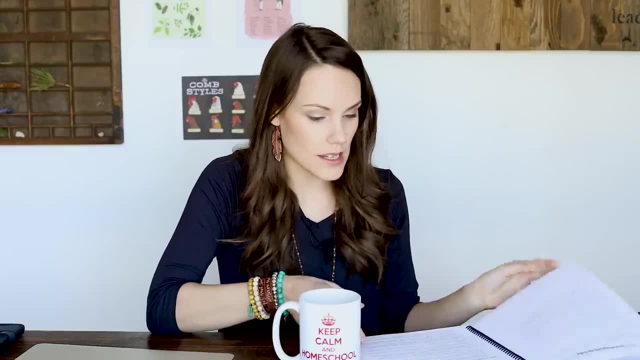 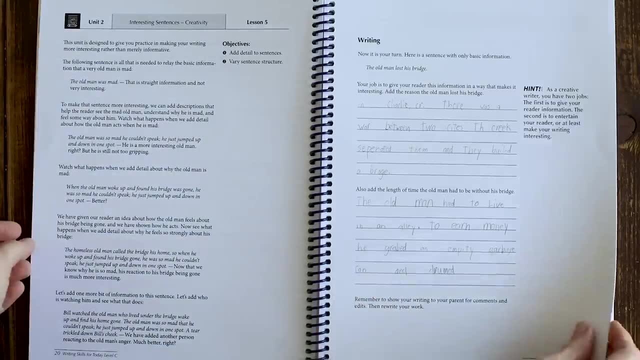 a letter how to write more interesting sentences And it kind of walks them through the process. So this is just writing And this will give you an idea. Let's take a look through some of the pages. You can see my son was trying this out. 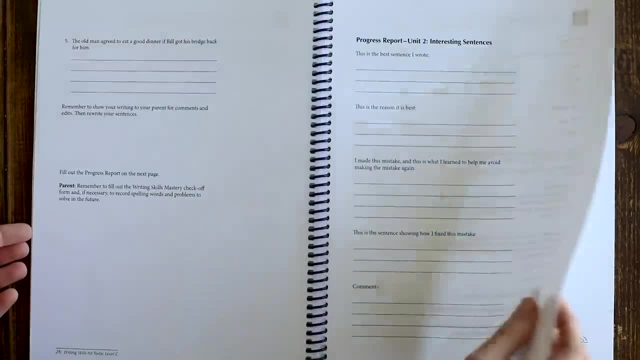 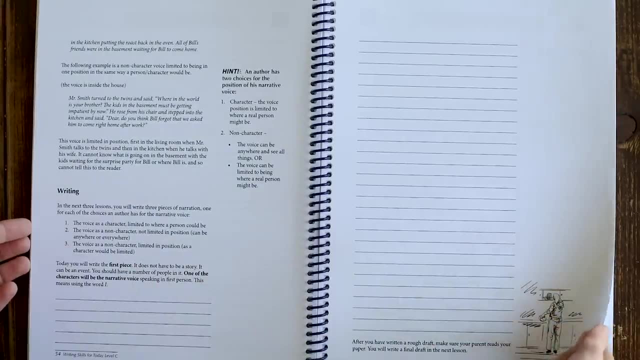 Okay, And again, this is not too overwhelming, And inside the Rome to Reformation, inside the actual schedule. they're not necessarily doing their writing every day either, because you have to remember, they're also doing writing inside the Rome to Reformation theme And there's some. 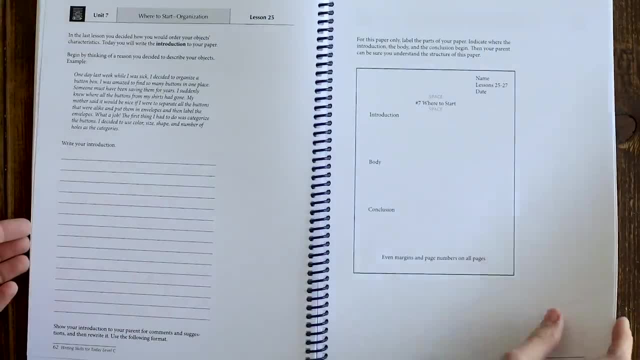 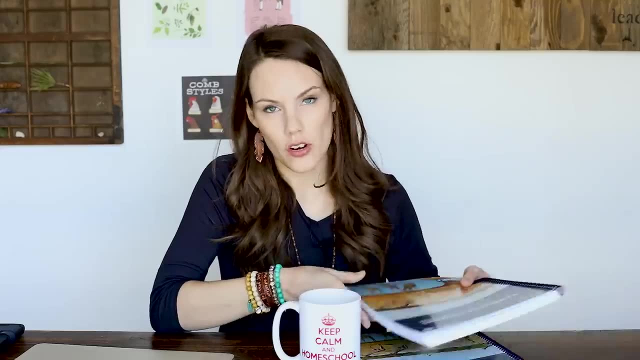 writing in language lessons for today. So it's- it is included in everything that they do. It is not just limited to these books that you're going to see listed underneath their language arts- The other resource you're going to see listed under language arts inside that elementary. 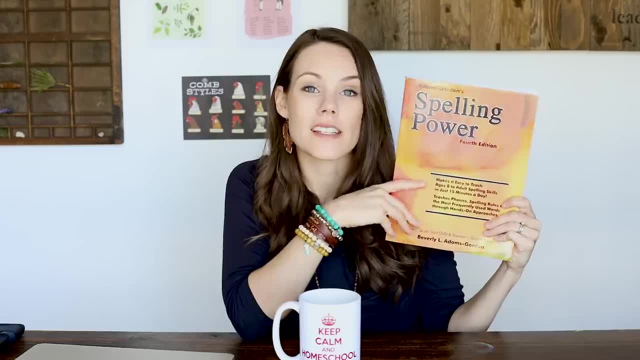 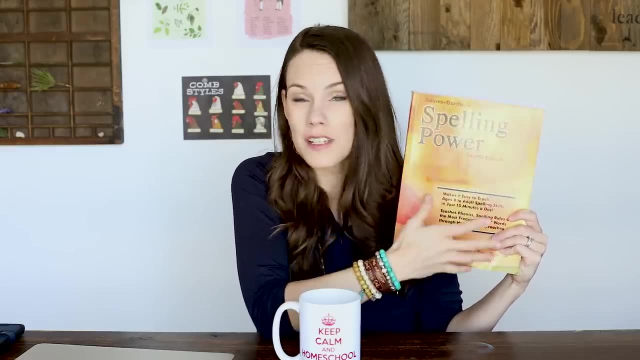 category is spelling Power. Spelling power is their recommended resource and it's included inside their Rome to Reformation schedule as well of just just 15 minutes a day spelling lesson. So this is the other resource you're going to see. We can take a peek at the table of contents of this one as well. 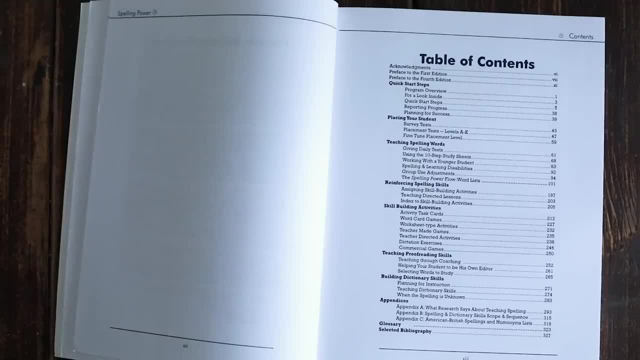 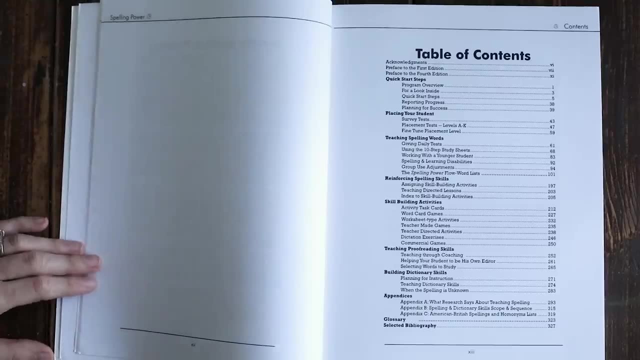 So you'll see that it tells you how to place your student, how you're going to teach it, how you're going to reinforce it. There's different skill building activities and proofreading and dictionary skills and all of the different tools that you're going to need, and 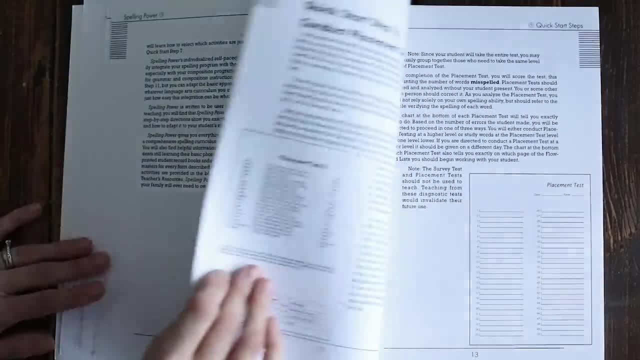 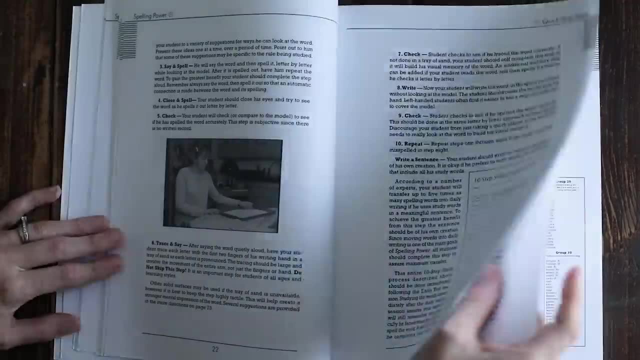 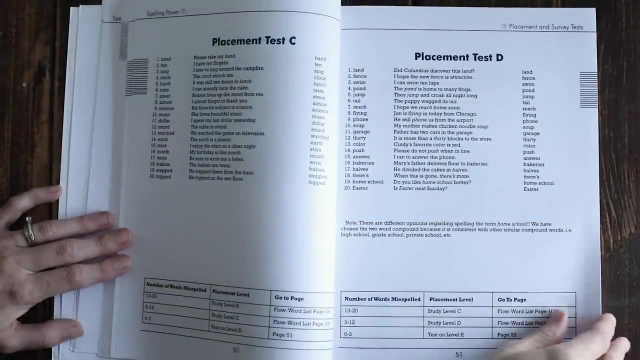 how you're going to create activities are built within this. So if I just do a quick kind of flip through, give you an idea, we can can see kind of kind of what it is. It is definitely written to the adults And so you would have to kind of read this and understand what the approach is. 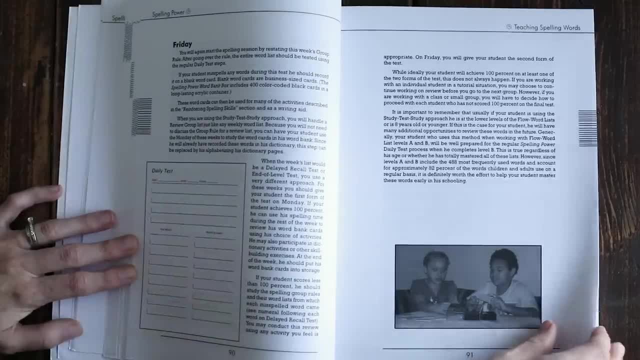 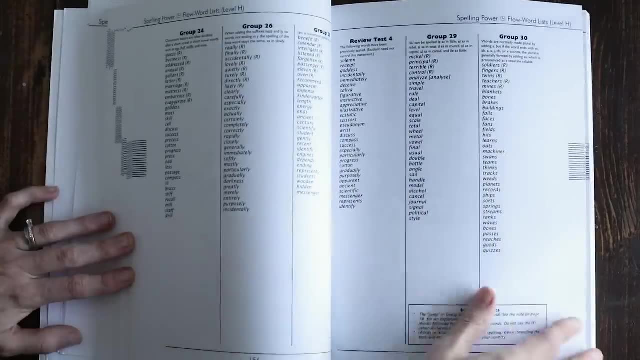 how you're going to do it, where your child would fit within this and then teach from that. So it's a little bit more teacher intensive, but it looks like a great way of teaching spelling. So this is the resource for that And, uh, that gives you an idea of how they do spelling within their program. 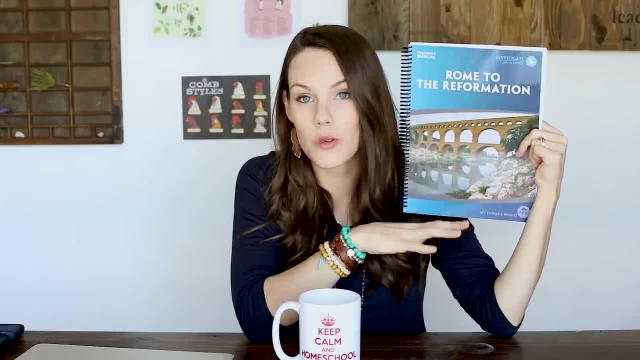 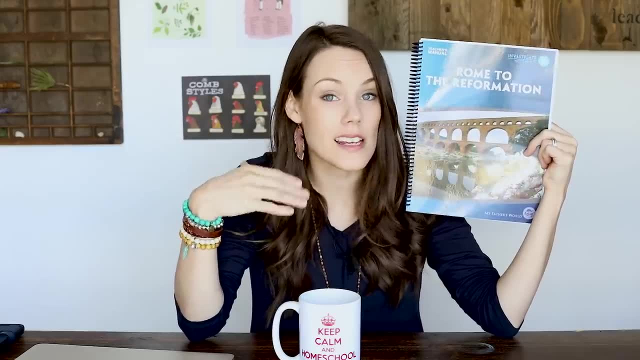 So the last thing I want to show you is Rome to Reformation, and I'm actually going to do a close up. I want to show you all the different books that are included in one of these kind of history themes. Now, remember, this isn't just history. This is history. It's art, it's music and 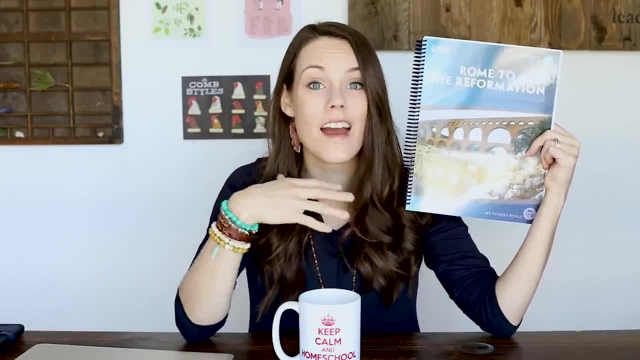 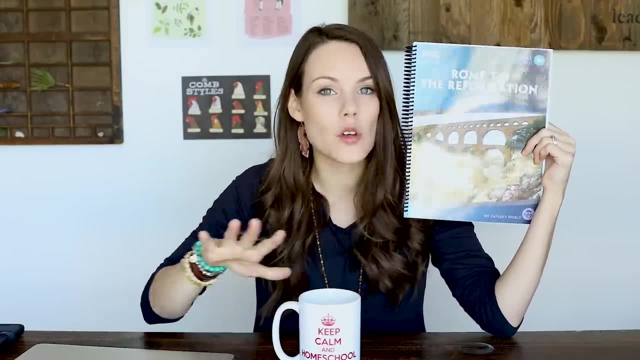 composers. It is your read alouds and literature and everything. It includes your science, It includes your Bible. It is such a comprehensive program So I'm going to show you all of those books And why it is priced, the way that it is priced and also how they incorporate language arts right. 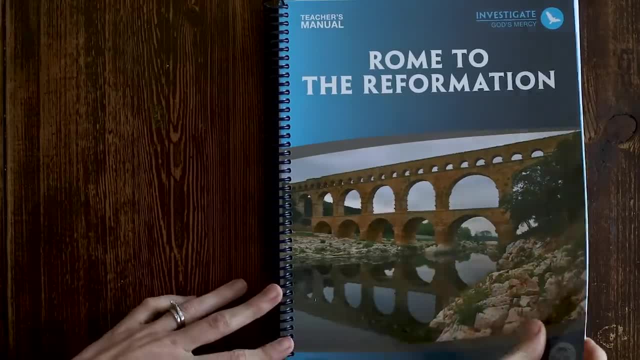 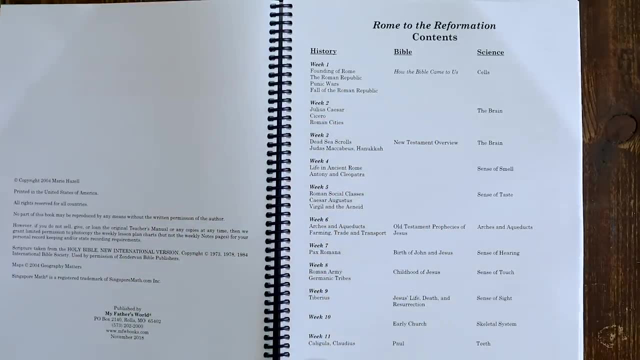 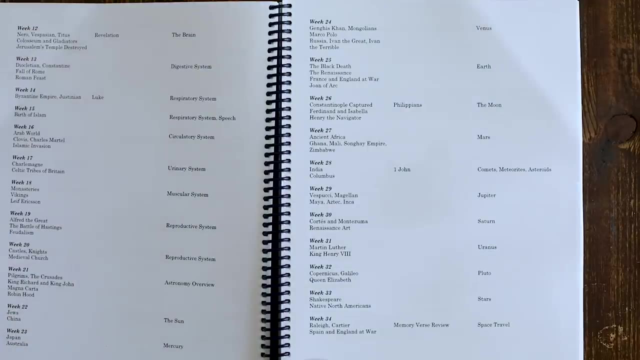 inside of their themes. So inside of this you can see that for science they are going to be doing the human body as well as space. for this year This is adaptable for kids from grades two- if they're doing it with older siblings- all the way up to about grade eight. And I want to take 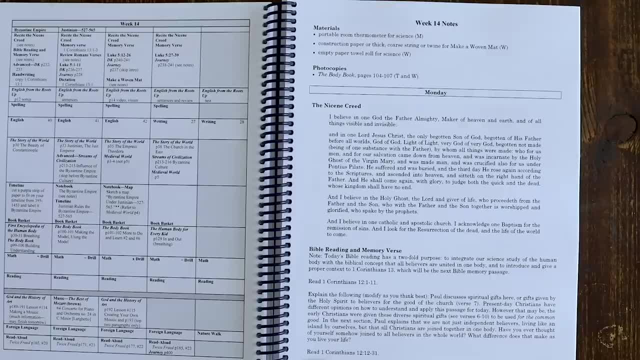 you to a sample week. So we're going to go to week 14.. So here on the left you can see this is our schedule and it is laid out with four days. It has an adaptable fifth day You can add in there if you want to. It uses English from the roots up Again. all of these things are totally 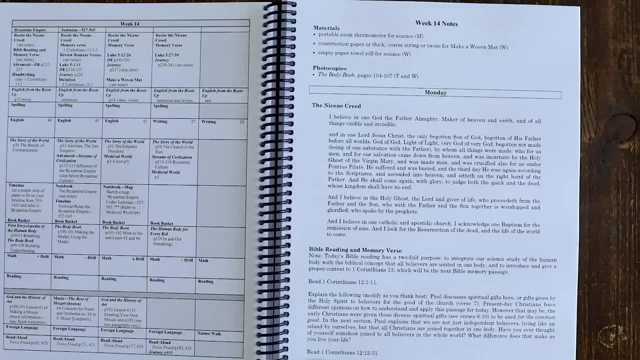 optional for you of how much you want to include and how much you don't want to include. But that would kind of be some of your language arts as well. It is Latin that they are teaching you some of the roots and Latin words, So that is an additional resource you can use for spelling It. 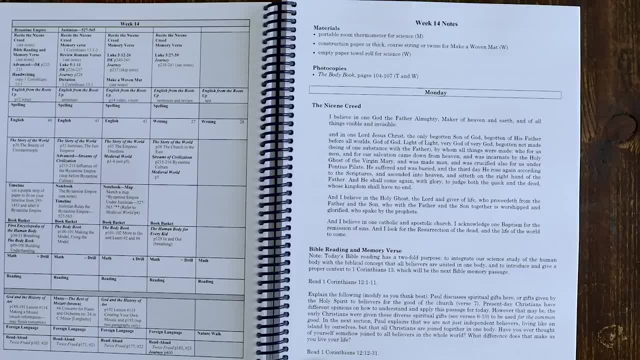 just gives you spelling, And if you were using the spelling resource then it would tell you what you need to do for that And you can see it separates The English- that would be your language. lessons and writing days are there as well, So it tells. 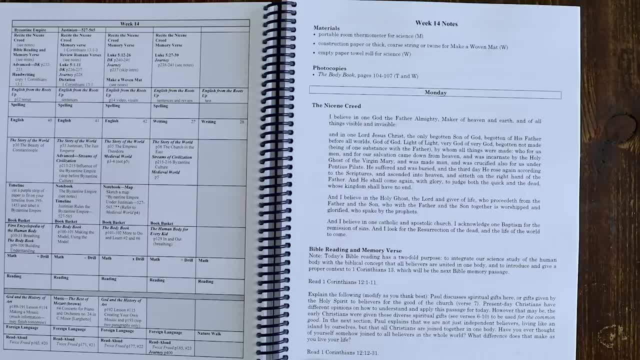 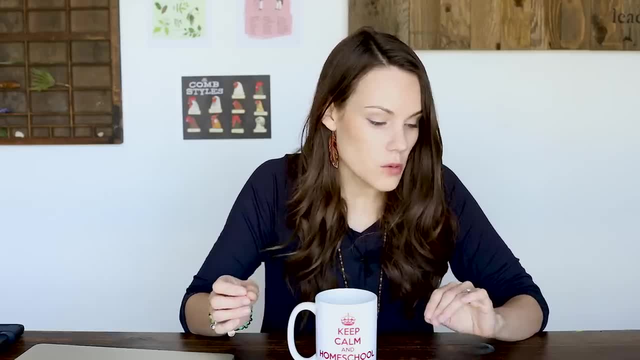 you everything you need to do, what you need to do, what you need to read. There is tons of read alouds included with the package. You're going to be reading aloud to your kids, You're going to be doing art, You're going to be doing science. Everything is listed here for you to do All. 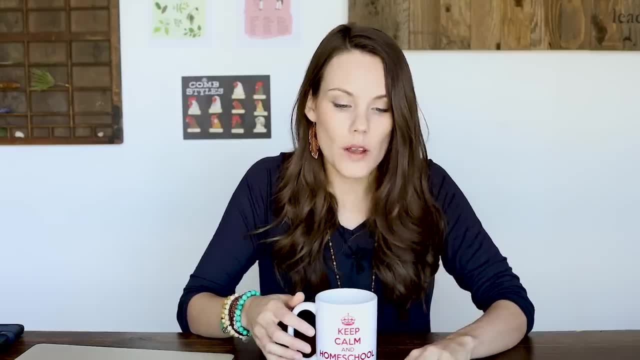 you need to add is math and an independent reader for your child. So if we look at the notes to the teacher you're going to see, it tells you what you need, the photocopies and each day it gives you as a teacher. 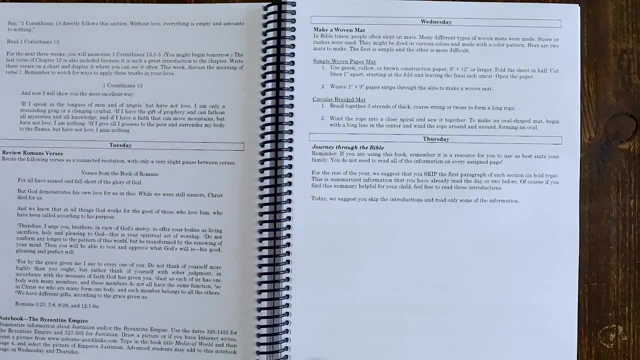 how you're going to teach this. So, specifically for the Bible, that's really important because it's telling you what you need to teach, what memory verses you need to do, et cetera. It's got lots of good discussion questions built into there as well. Um, it tells you each day is kind of 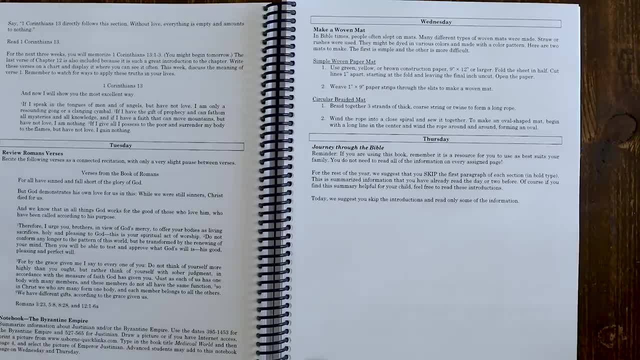 broken up for you So you can see it's got different verses you're going to be studying and it incorporates notebooking all throughout. So the notebooking is where you're going to start to see some of those language arts built right within. not only is it very project based, not only is 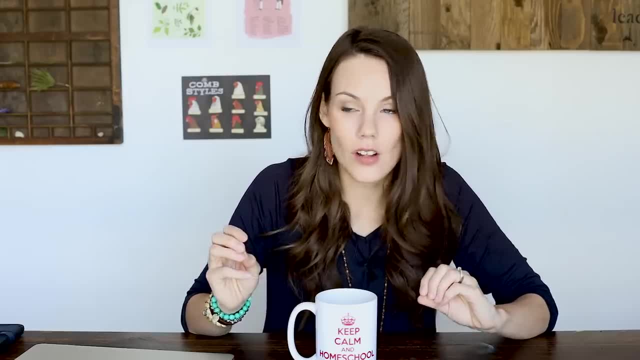 it very um. you know they're going to be doing lots of reading and lots of discussion and lots of oral narration and memorization, but on top of all of that they also do notebooking, and that's where you're going to. 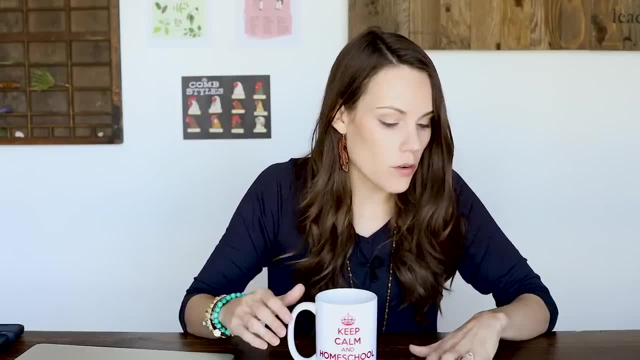 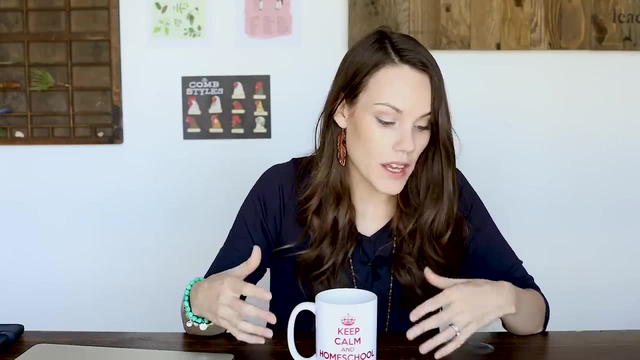 start to see the language arts incorporated into these themes. So, for example, it will tell them: you're going to read this and you're going to write this about it here. They're going to summarize the information about what they are reading in their books. So they're going to read. 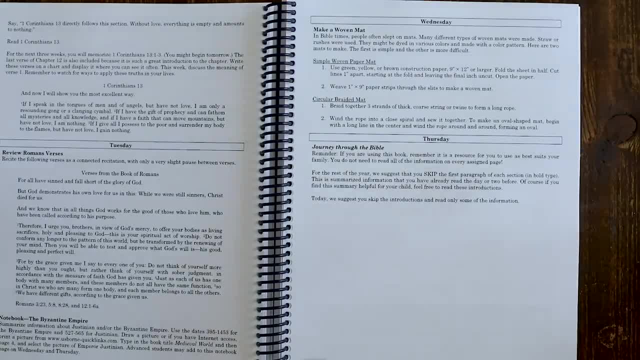 in the book, draw a picture, and they are going to write about it and add it to their notebook, So that gives you an idea of how language arts is incorporated right in. on Wednesday, you can see that they are going to be making a woven mat, which is just how you can get. 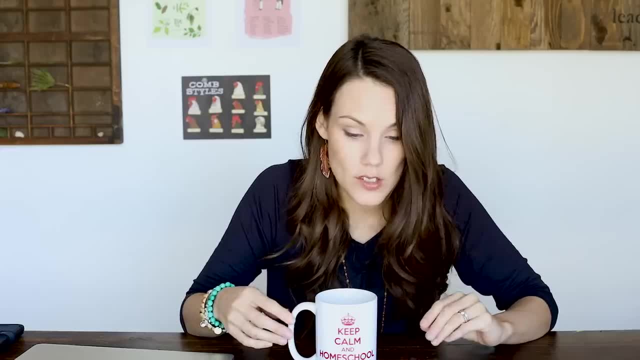 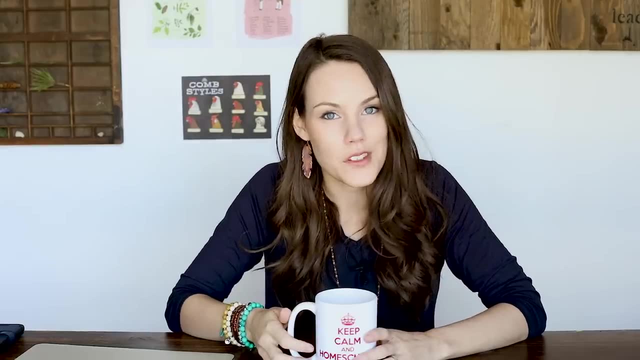 an idea of how kinesthetic and hands-on it is, And there's lots of projects throughout as well, And then it also has, you know, lots and lots of Bible included in there. So let's take a look at some of the different books that are included inside the Rome to Reformation So you can see. 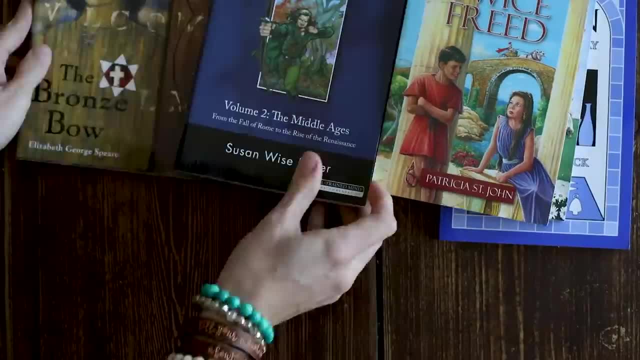 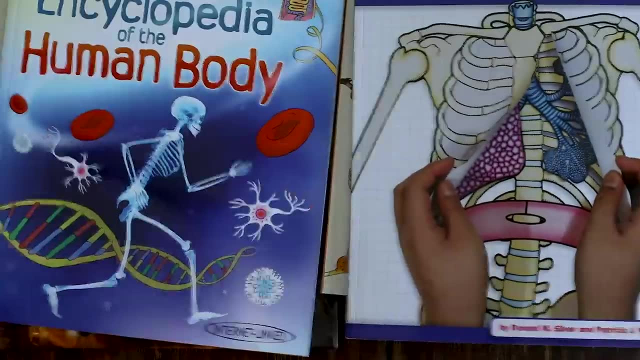 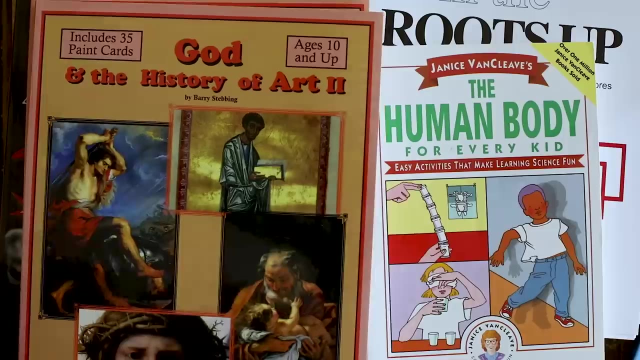 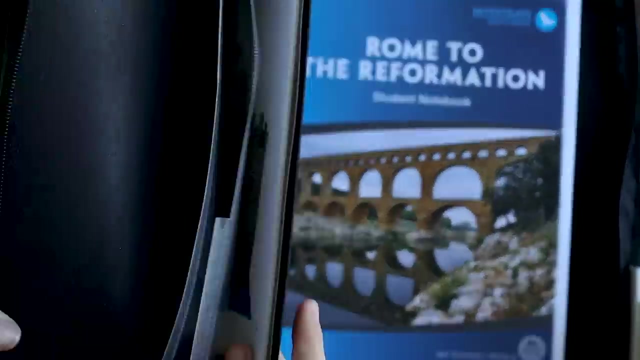 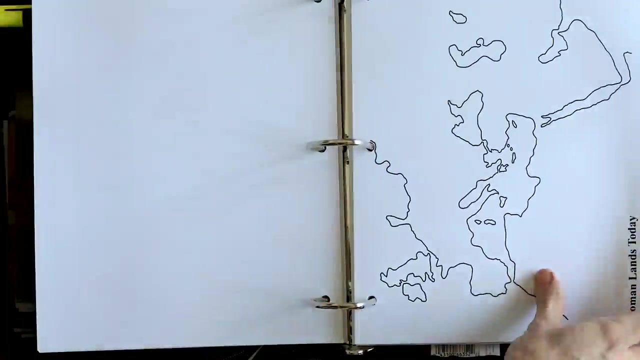 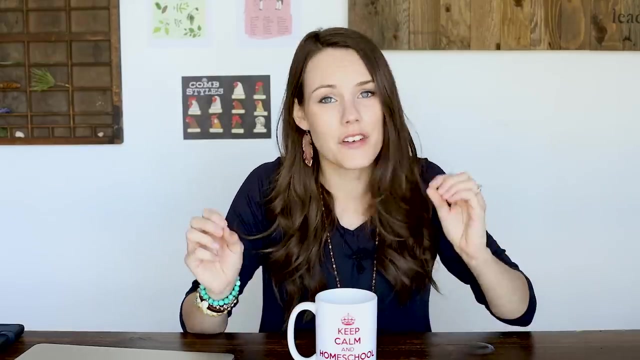 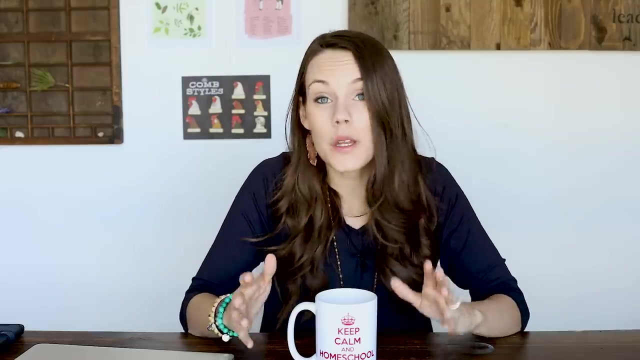 why it is so comprehensive. All right, So that's My Father's World. obviously a very quick little snapshot to give you an of how it works, how it is taught and what it looks like inside. but what I really want to talk to you about is who this is going to work well for and who 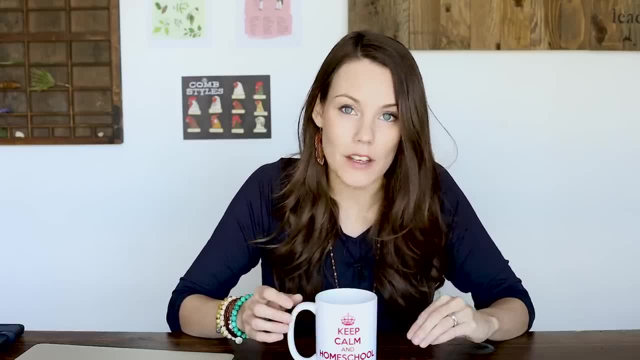 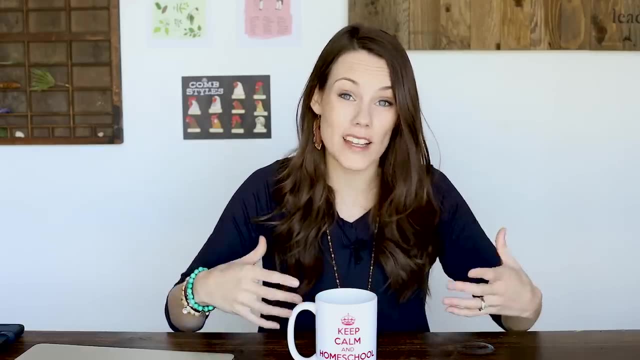 it isn't going to work well, for this is going to be a fantastic program. if you are looking for something you can teach with multiple kids, it's gonna work really well. if you want something that's more Charlotte Mason inspired, a little bit more gentle and less focused on heavy workbook, you know reinforcement. 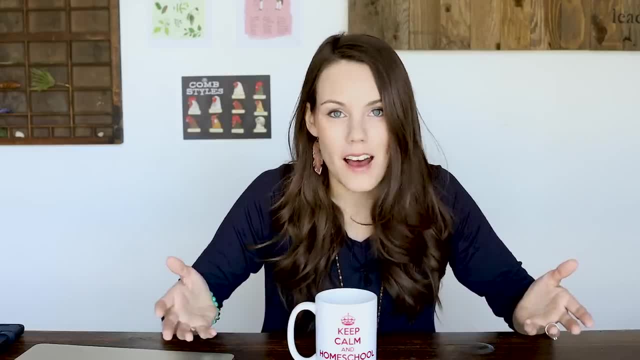 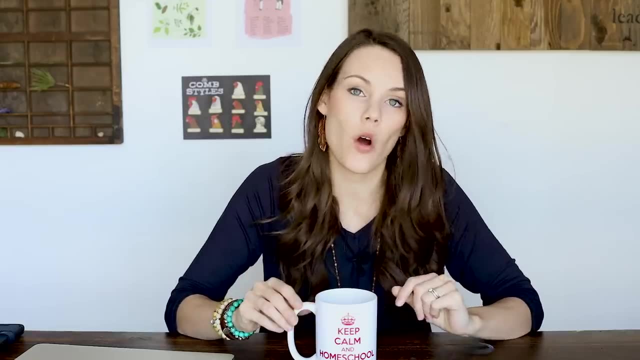 and drill based learning. it's gonna work well for all different learning styles because it has hands-on, because the auditory kids are gonna get to hear it, because your visual kids are gonna get to see it. so it works well for all learning styles and it works really well for blending your kids, which can save 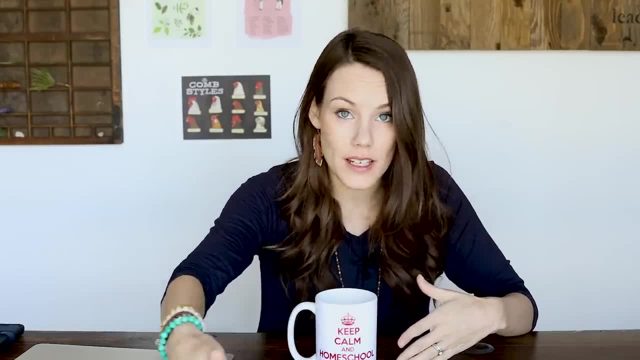 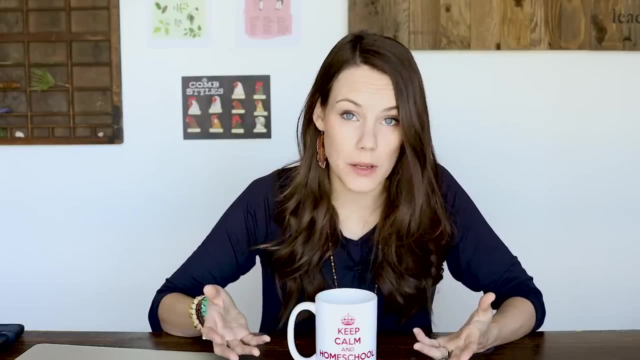 you time instead of having to teach one-on-one for each of your kids for each of their subjects? who this isn't gonna work well for is anyone who's looking for secular curriculum. obviously this is very Christian based. if you're looking for a secular, you're gonna want to skip forward, because I've got some 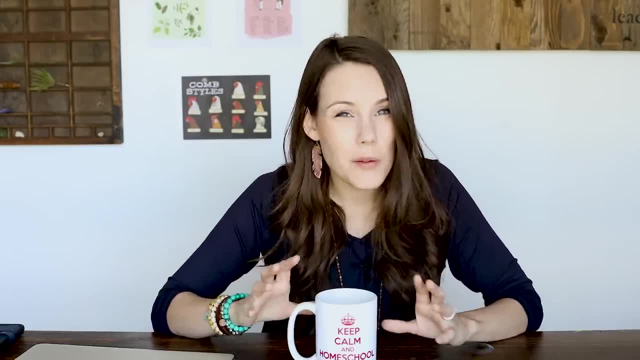 different options for you there as well. it is going to not probably work for you if you are on a very strict budget and can't afford this kind of price tag. okay, so I'm going to show you how to teach one-on-one for each of your kids. 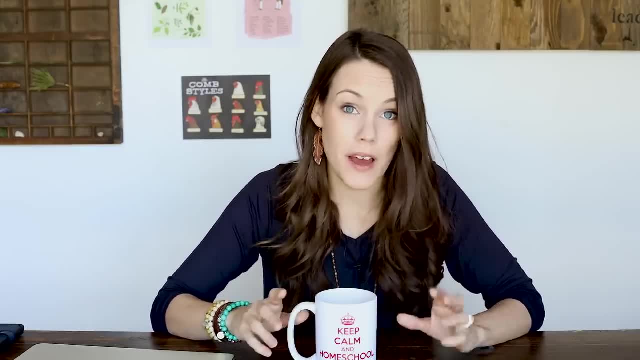 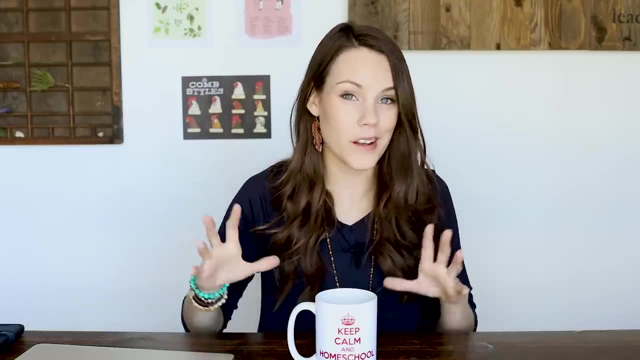 the language lessons and writing skills for today are very affordable on their site, by the way. if you want to just add that to whatever you're doing, they're like $19. but if you want to do this whole curriculum and the way that it teaches all your subjects together, that Rome to Reformation package is about. 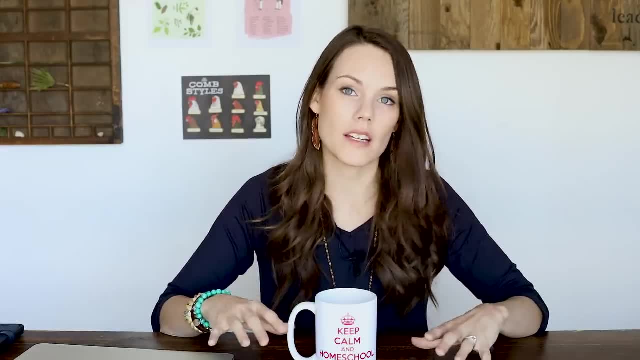 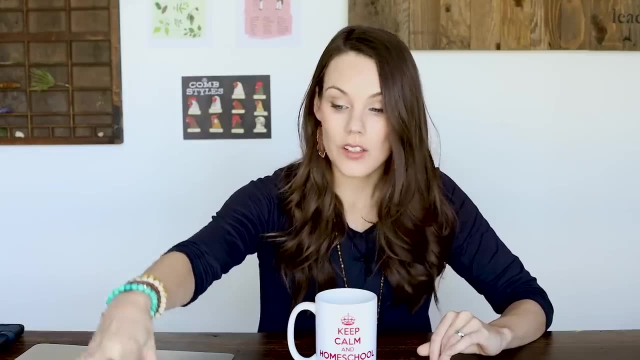 $440. but keep in mind- is really important to keep in mind- that when you price out music study resources and art resources and you know science resources for each of your kids and Bible resources for each of your kids and history resources for each of your kids and history resources for each of your 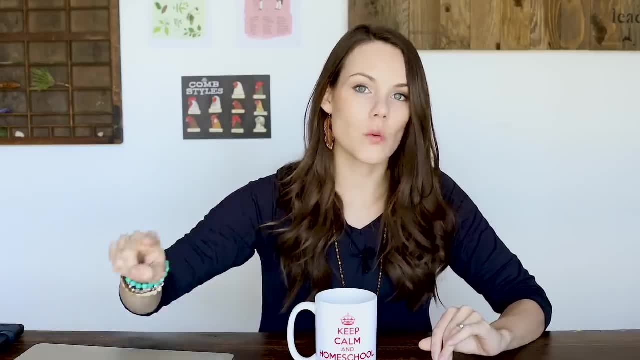 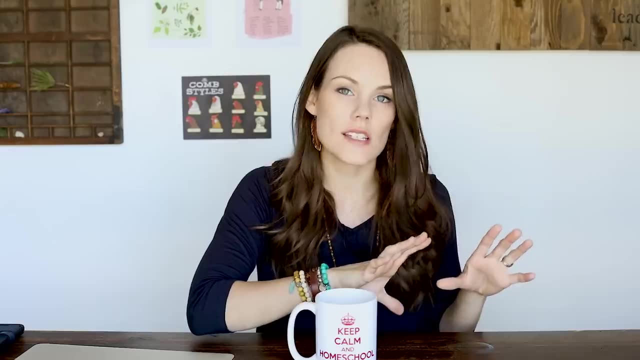 for each of your kids and language arts resources for each of your kids. it usually works out to a whole lot more than that, So that price tag seems big overall. with any of these all-in-one curriculums I'm going to be showing you, you're going to see that. You're going to see that sticker shock. 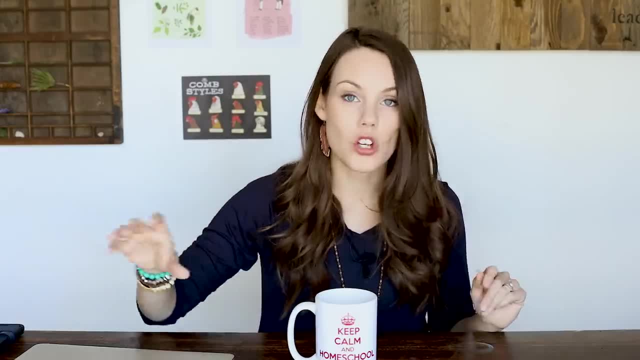 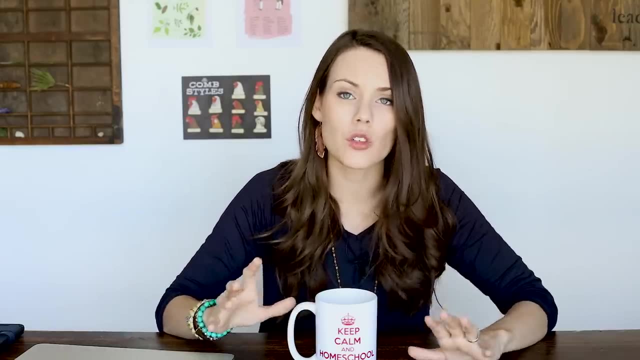 but keep in mind that it is taking away the need for you to go and buy this times five or however many kids you have. So it's just lots to think about when you're looking at this curriculum. but if you do have a very limited budget, then definitely budget's going to play into that, for 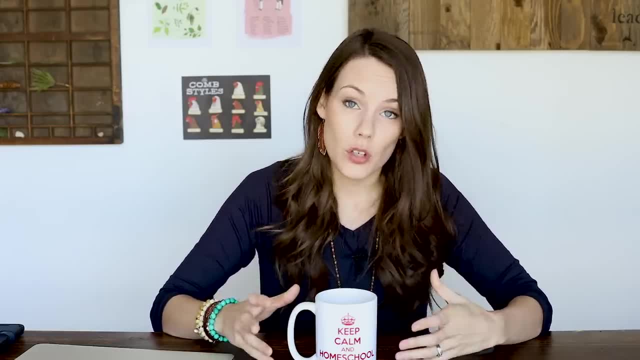 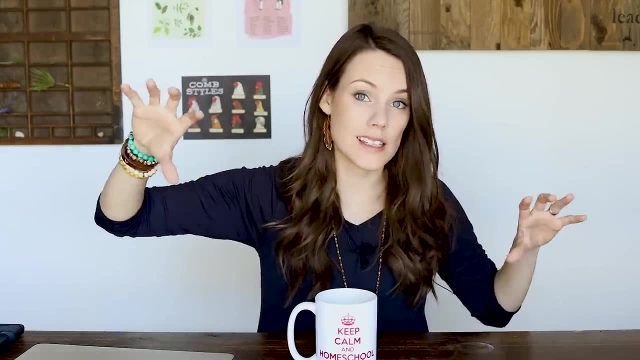 you as well. The last thing that I think would maybe be a detriment for you, depending on your situation, is if you have a very intense, busy life or, like I said, are dealing with kids that are very um, very different age groups, If you've got five-year-olds that you're trying to do. 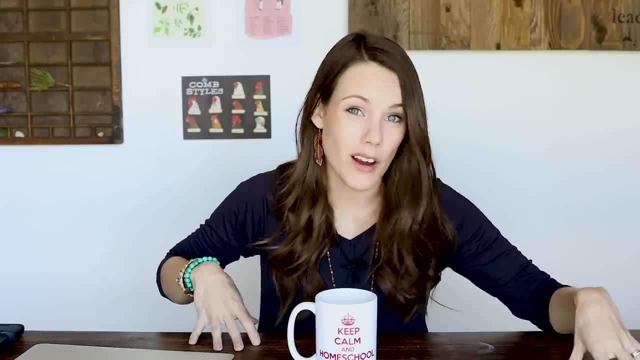 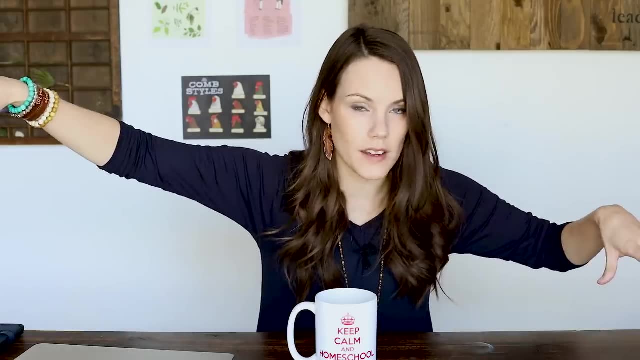 kindergarten and phonics and, and you know, learning how to read and write, at the same time as you've got high schoolers, at the same time as you've got middle schoolers, and you're trying to blend this in with some kids, but still do stuff with the other end of the spectrum. it's going to 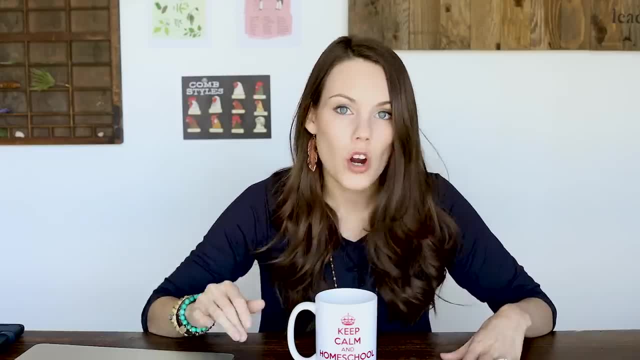 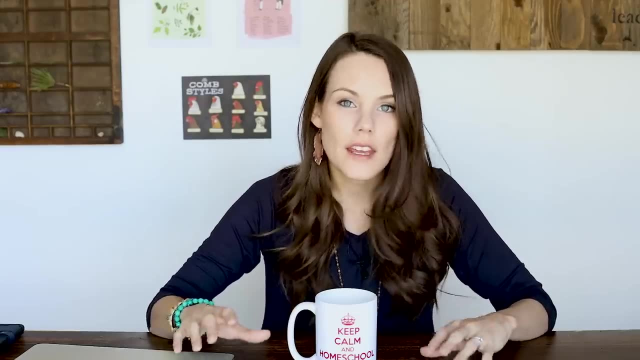 be probably too much. If you have a job and you work almost full-time and you need something that you can just start them on and they can do and you just get school done. those are the situations that I think that my father's world would not work as well for, because it is more parent-led, it is teacher. 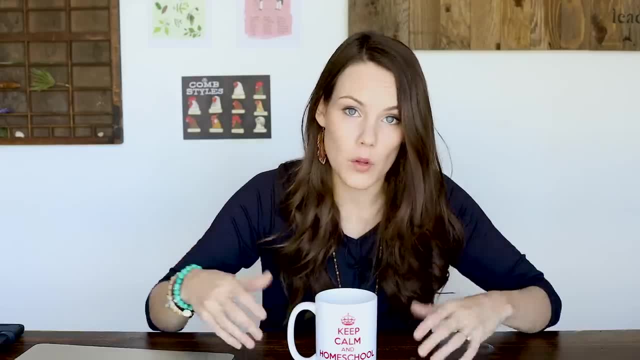 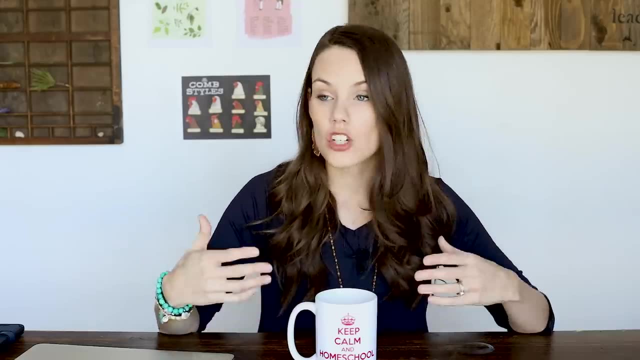 intensive in the fact that you have to be the one teaching, you have to be the one reading, So it is not too time intensive. You can see, the days are actually very, very gentle. It's it's just reading and discussion and it's not too much built into it. And, of course, 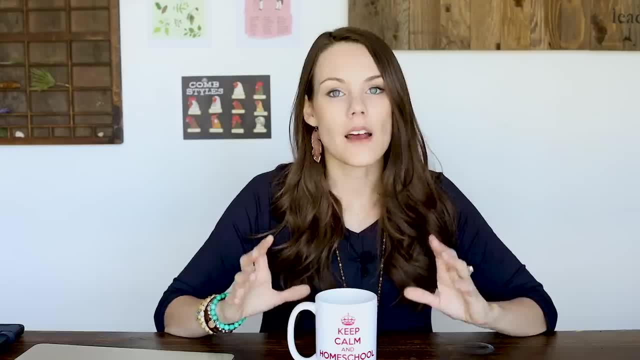 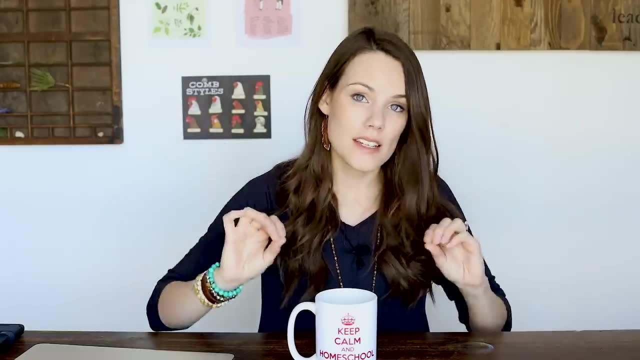 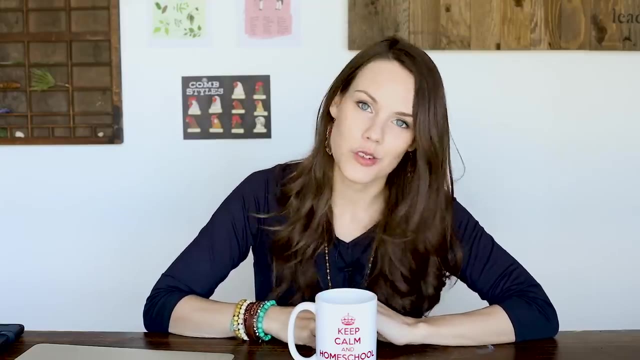 all those activities are optional, but it is something that you, as a teacher, will have to lead. If you do not have the time for that, or your family dynamics do not work for that, then this may be something to consider when you're looking at my father's world. So let's move on to some of the other programs that I have to show you. 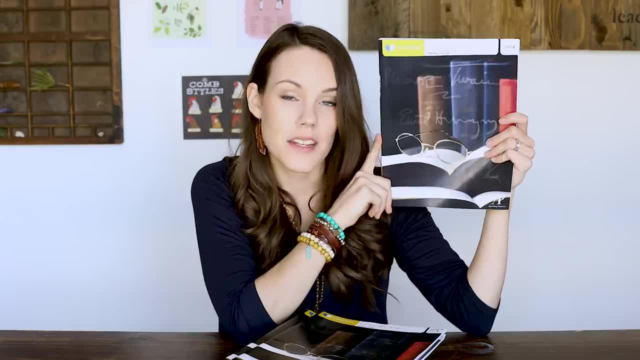 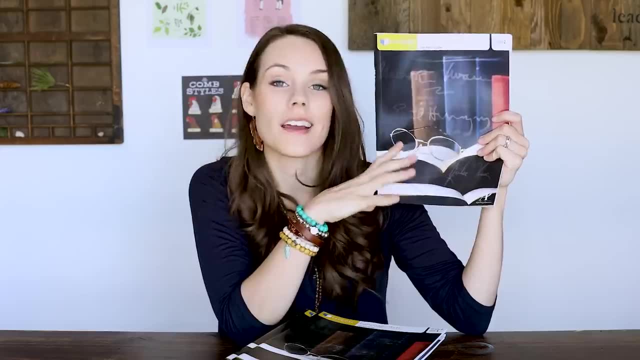 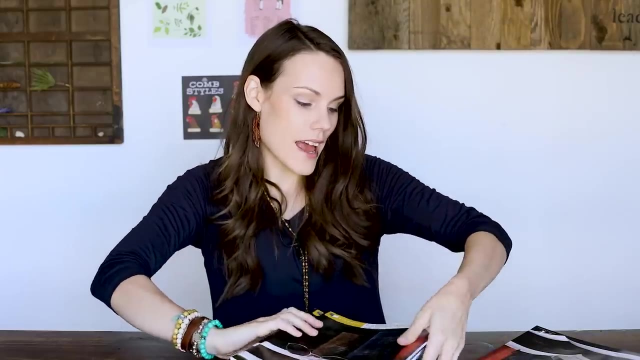 today. The next program I want to show you is LifePack by Alpha Omega Publishing. Now, LifePack you are going to get for each subject, so language arts, for Bible, for science, for socials. you're going to get a teacher's guide as well as 10 different unit booklets. So they 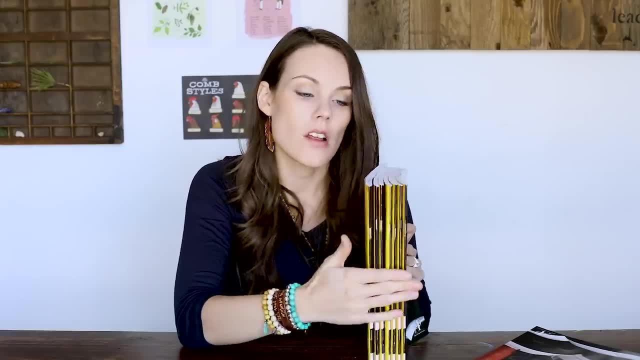 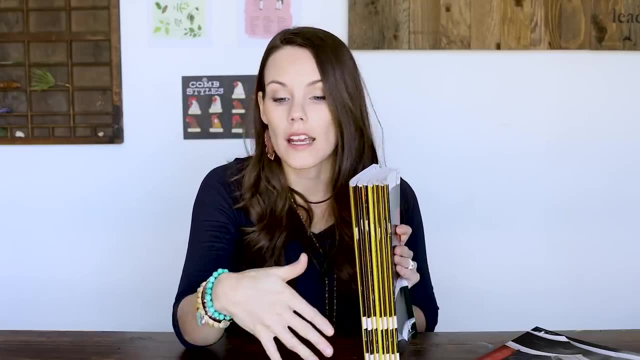 would do essentially one booklet per month per subject. A lot of parents love this because they can just open and go. This is definitely pretty much the opposite of my father's world, where my father's world is very Charlotte, Mason and exploratory and incorporates all those amazing 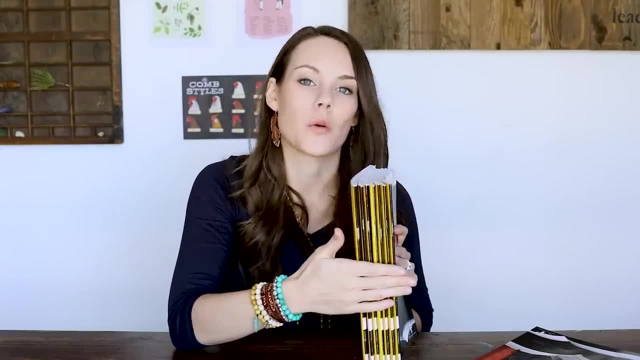 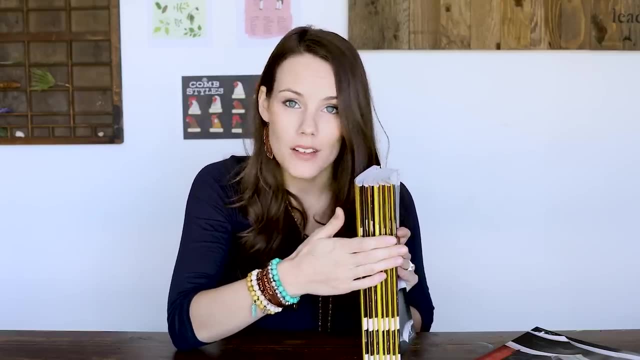 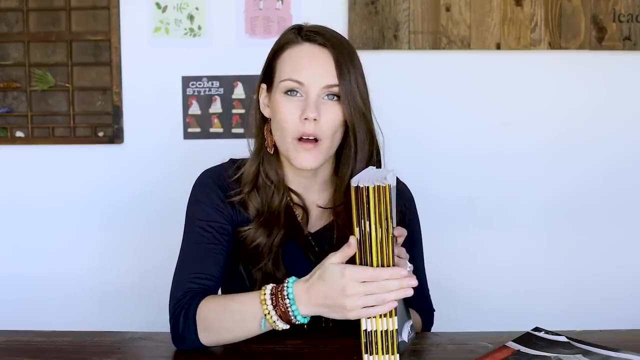 things. This is traditional, traditional schoolwork, where it is bookwork open, go read, write, do what it says, follow the instructions. This is also very, very independent, where my father's world and some of the other curriculums I'm going to be showing you today are more teacher led and directed. So this is one that 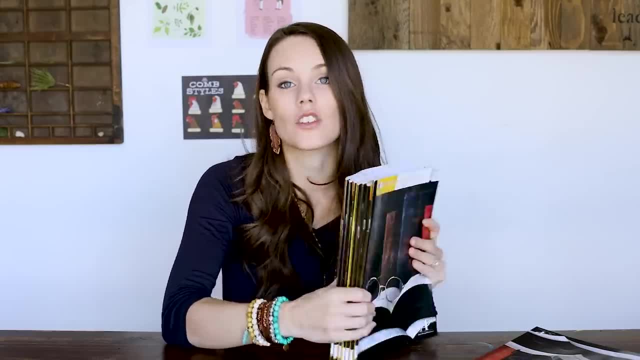 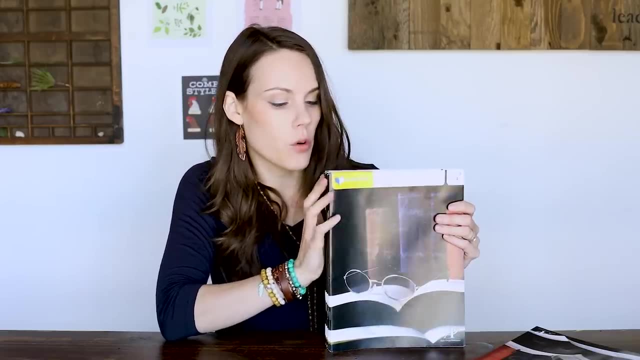 you're just going to kind of get them started. Once they're familiar with the way this works, they can do them on their own. So I want to show you inside these, give you a glimpse. I'm missing a few. I have unit four through 10, I believe of this, as well as the teacher guide, but I want to 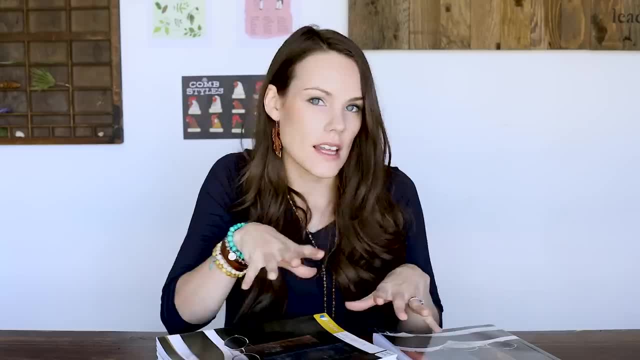 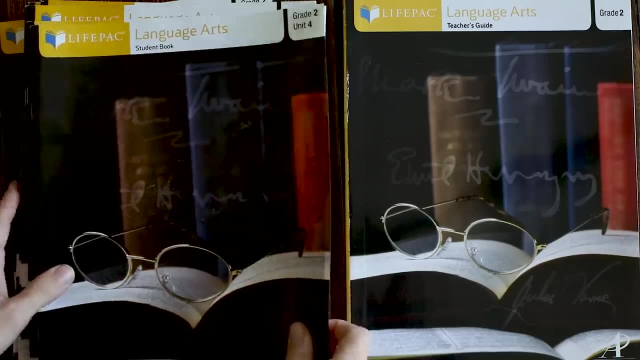 show you how it is laid out so you can see what this looks like inside. So let's take a look at the table of contents inside. We're going to look. this is unit four, So I'm not gonna show you inside all of them. I'm trying to keep this as short as possible. 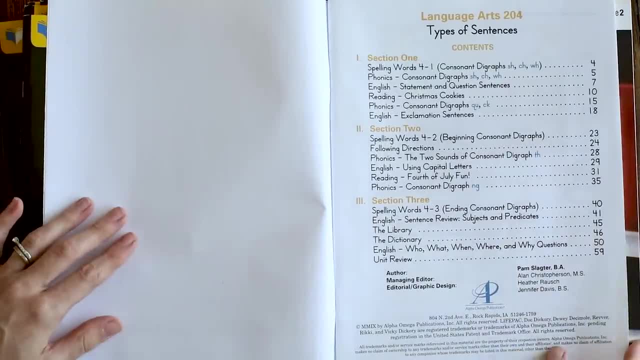 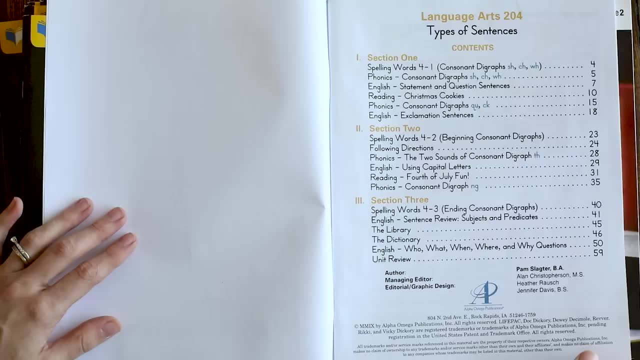 which is going to be a challenge. So here you can see that inside one of the kids booklets they have their different sections they're working on. There's unit review built in and they're just kind of working through and following directions of what this booklet says. that. 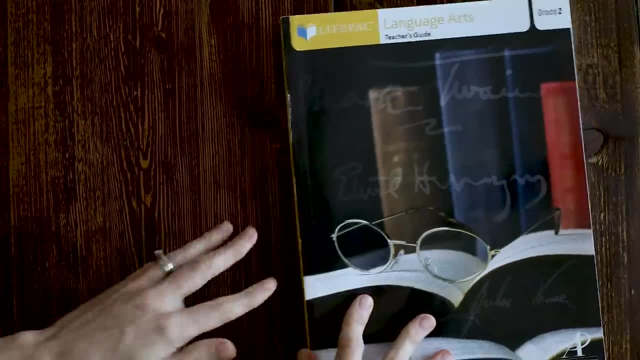 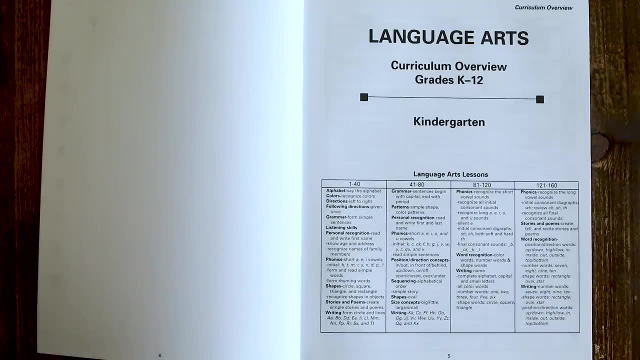 they need to do The table of contents inside the teacher's guide. If we go to the curriculum overview, that shows you for each grade. So we can look here at grade two where you can see all the other ones, what is going to be covered in their language arts for each grade, in each unit. 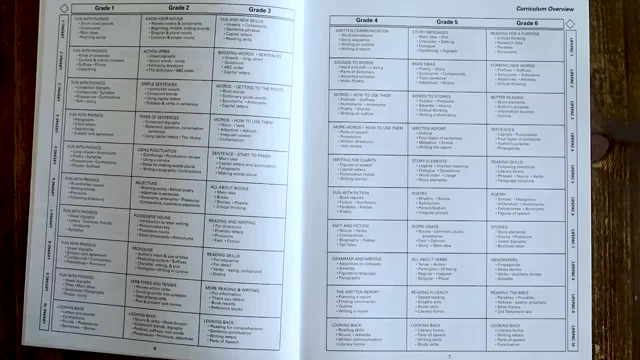 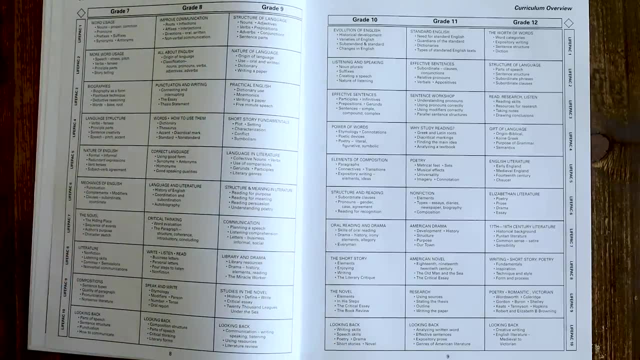 So if you are considering this, you're going to want to take a screenshot of this so you can see and go and see what it would look like for your child. So it goes all the way to grade 12 and these are all the different things that are covered. 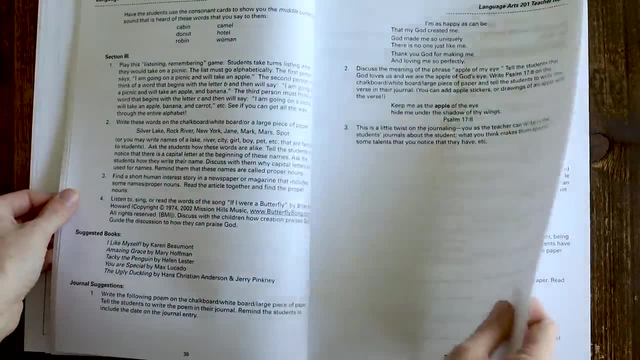 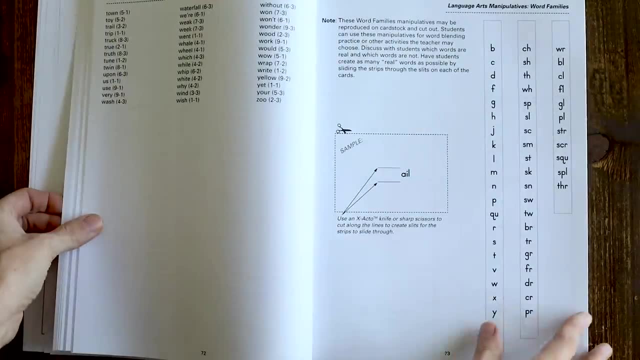 So if we skip forward, it's got grade two grading- how to grade their lessons. There's a weekly lesson planner and then it goes into the teacher notes So it actually will tell you you know what you need to be doing. 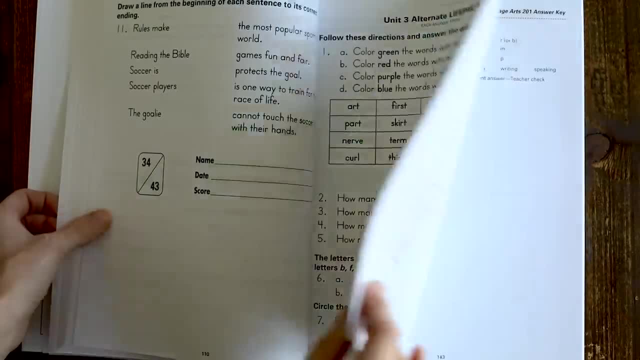 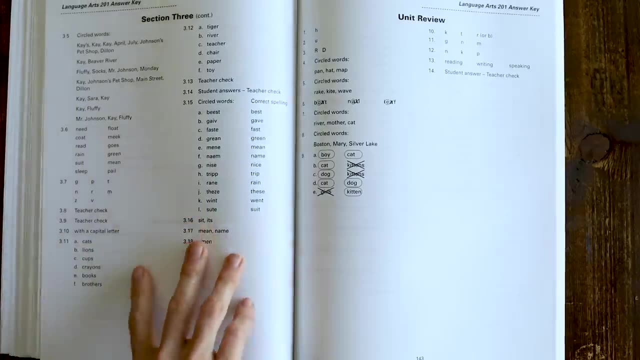 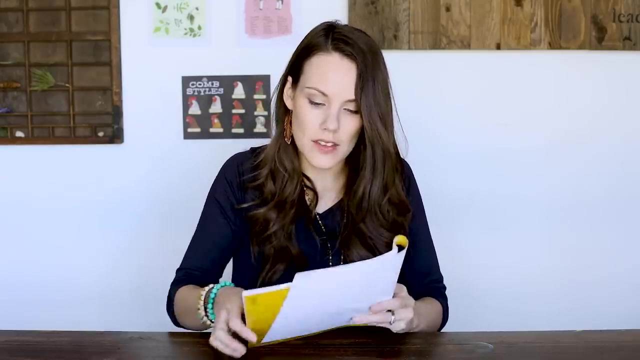 There's alternate tests that are in here as well, And there's spelling tests that are in here, and it gives you different materials that you need. It gives you an answer key. So all of that is right here inside of your teacher book Now inside the unit, just so you have an idea of how it's laid out. Remember, this is the grade two. 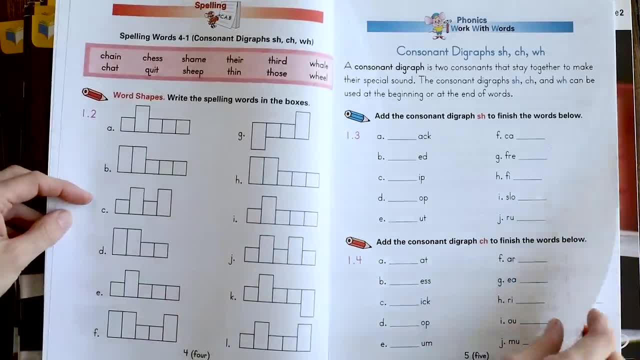 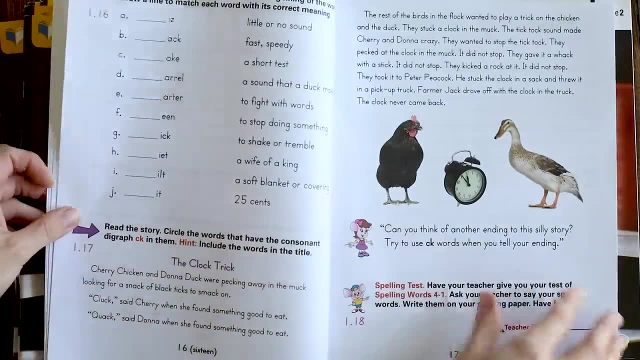 Obviously, it's going to get more in depth. It's very bright. It reminds me a lot of a Becca, which I'm going to be showing you as well. but it's very simple, workbook style. Fill in the blank. write the correct word, circle what you need to circle. 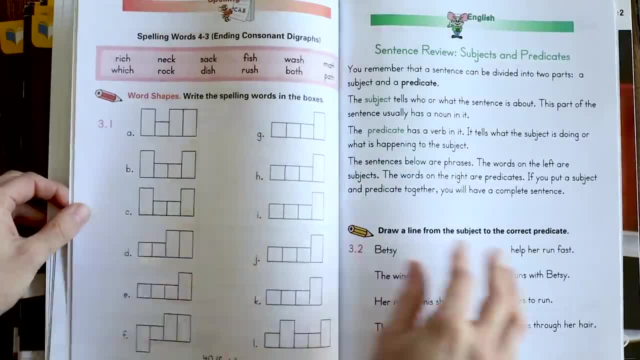 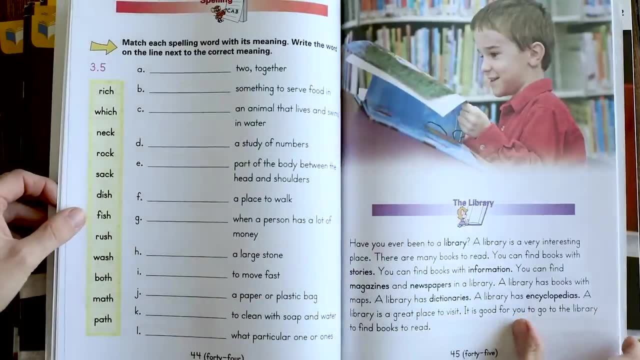 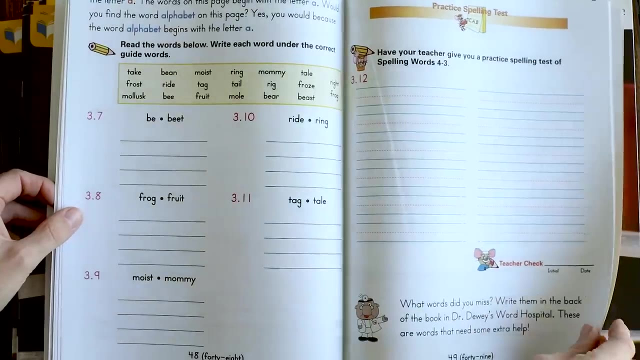 It's definitely very traditional in its approach, So this does work well for families that are needing something that is laid out in a way like this that they can just give them their workbooks and have them go. It also works well because you just have this one unit book for language. 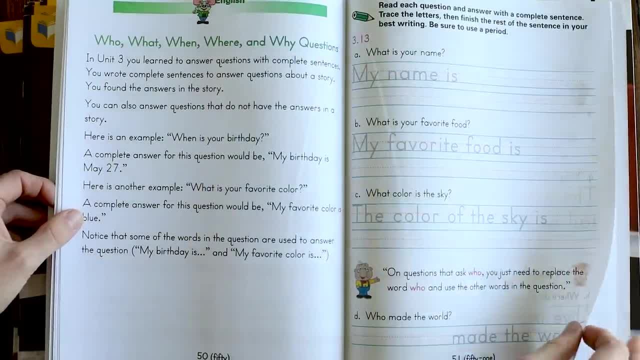 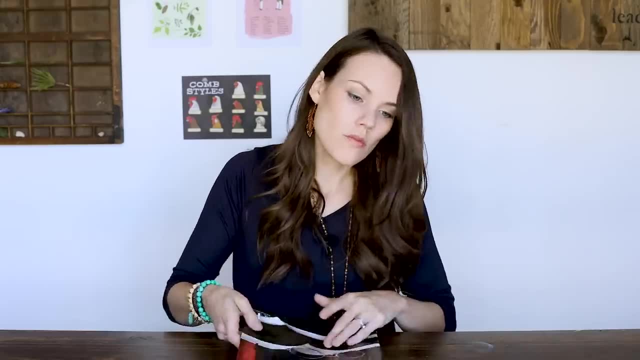 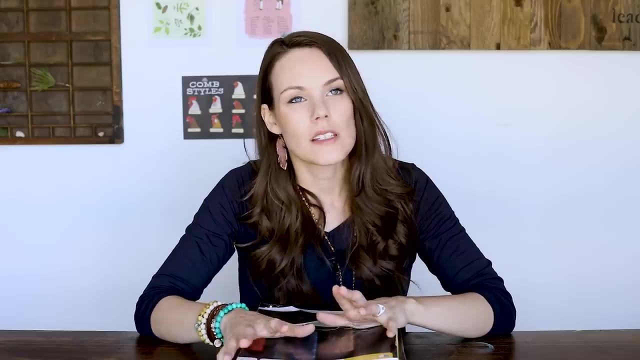 arts that you can take with you. It's not like you have to bring five different you know language arts books with you and read alouds and resources, And then you'll see the unit test is built in there as well. So that is LifePack by Alpha Omega. It is not cheap, depending on how many kids you have. 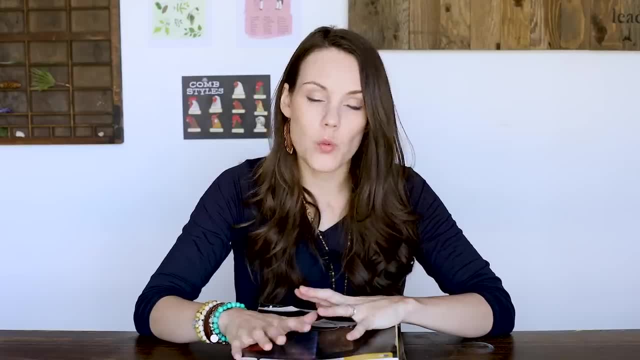 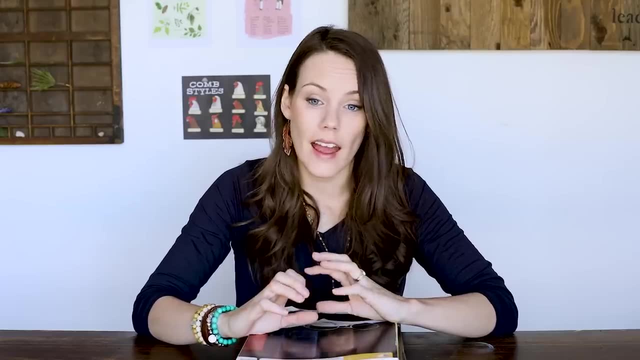 but it's definitely new. So that is LifePack by Alpha Omega. It is not cheap depending on how many kids you have, but it's definitely new, Not crazy crazy expensive either. It works well for kids that are more visual. It works well for parents that need something that is more child directed and led and is open and go. 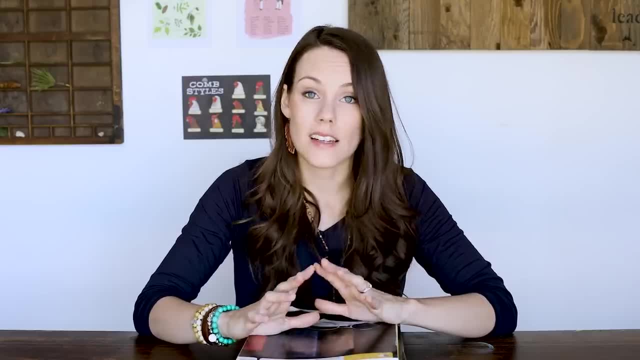 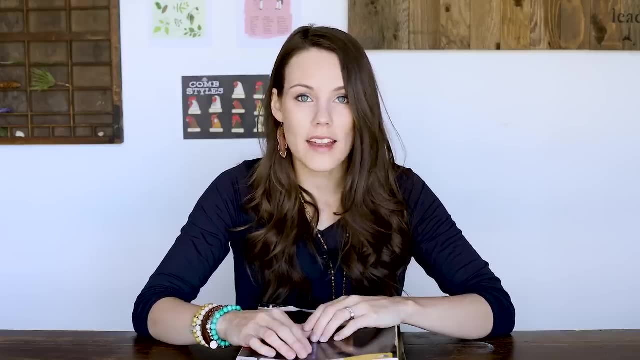 and independent from them. So if that is you, then this is going to work well for you. It is also Christian. It is not going to work well if you are secular And if you are looking for anything that is just the joy and love of learning and exploring the. 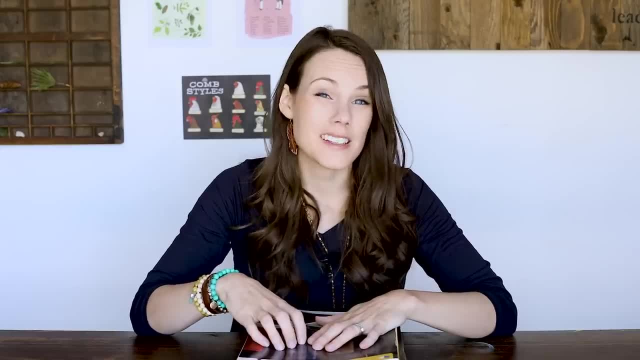 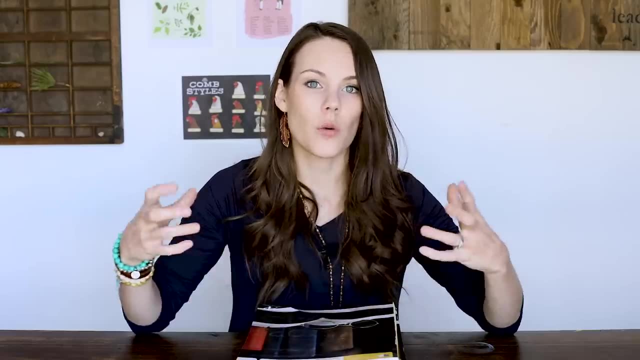 world around you or Charlotte Mason inspired. I would recommend finding something else than this, Because this is very, very traditional. It's going to get the job done, but it's not going to get it done in a way that is going to you know. 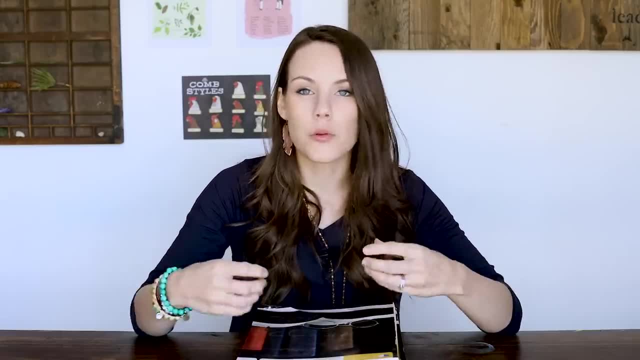 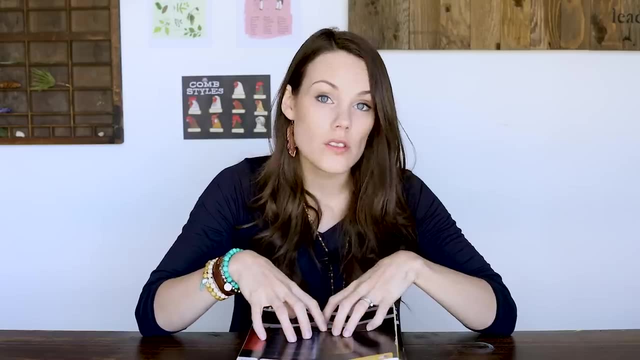 be out of the box and going to really explore good literature and all those different things. That's not included in this program. So, depending on your goals as a family, I would look at that first. What is your goal? Do you need something just to get it done? 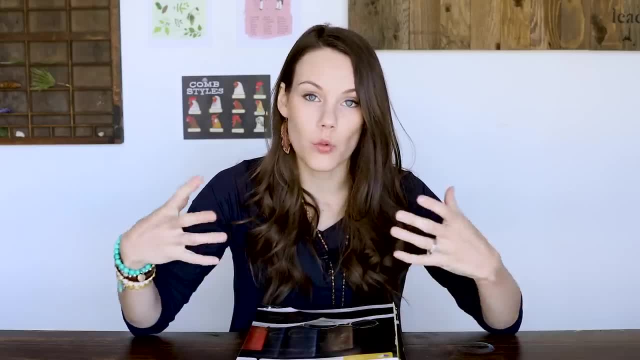 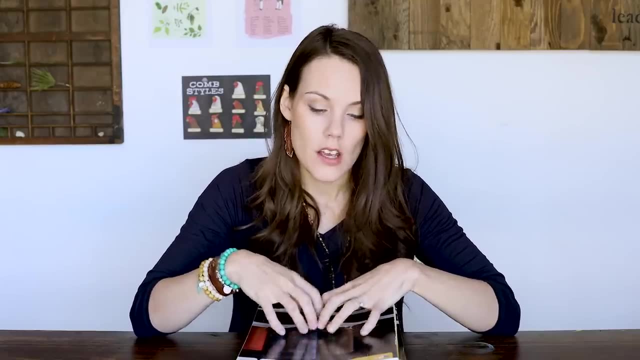 Or are you looking for something that's going to really inspire that level of learning or give that rich Charlotte Mason or unschooling or unit study approach, Because this probably won't be a good fit in that case. So take a look at it. 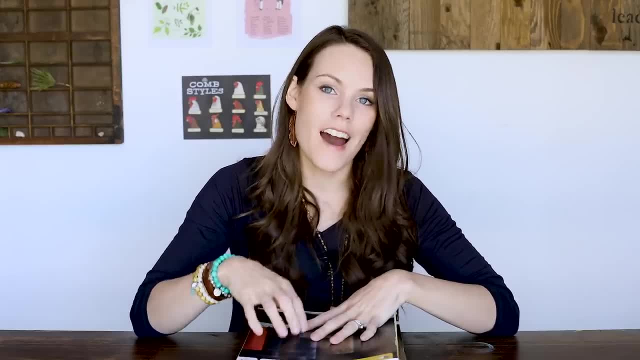 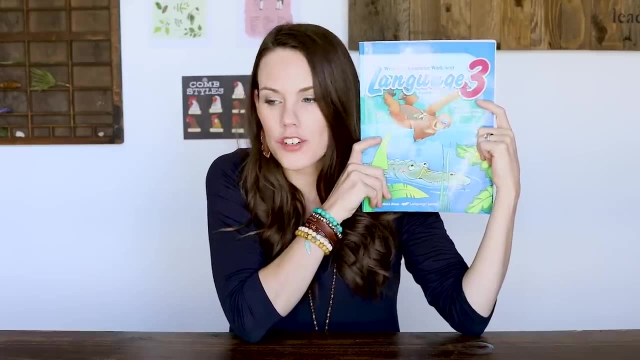 You can go to their website and learn a lot more and check out more samples, But that is a life pack, All right. Now we have a Becca, which you're going to see some similarities between Alpha Omega as well as the Becca. 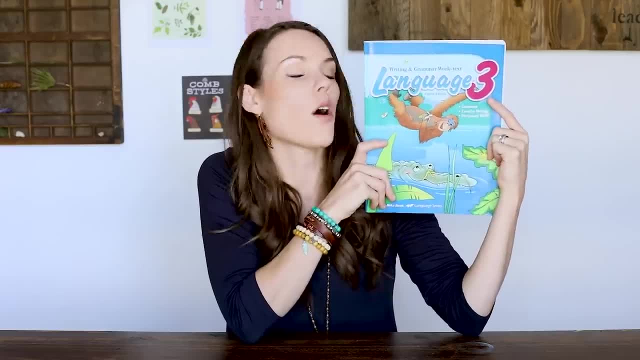 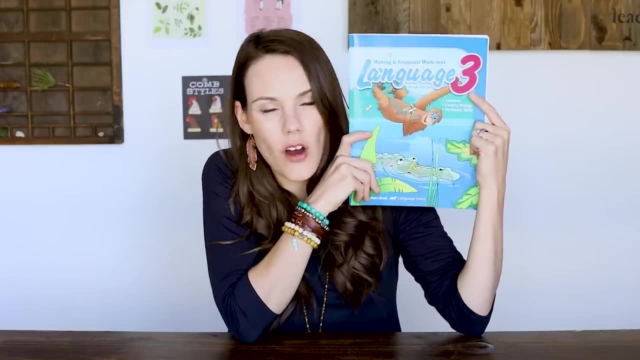 This is also Christian based. Okay, All of their stuff is Christian based. It's not as infused throughout their program, though I have heard of secular homeschoolers using it and not, you know, finding that it's. it's too. 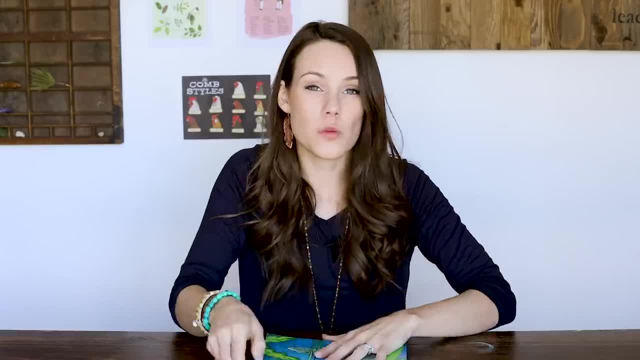 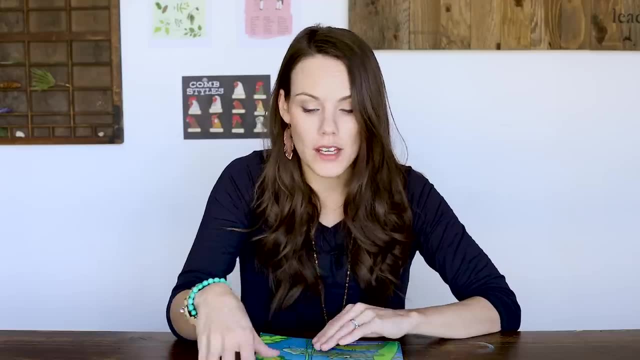 in your face. So that's something to keep in mind. There are teachers resources to go along with this for the younger grades. I never thought it was necessary for the older grades. It can become a little bit easier for you for your marking and stuff like that. 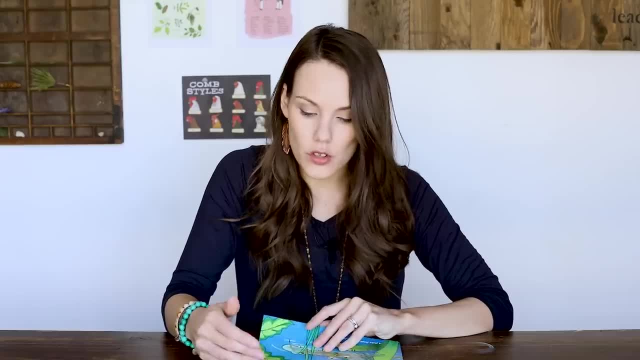 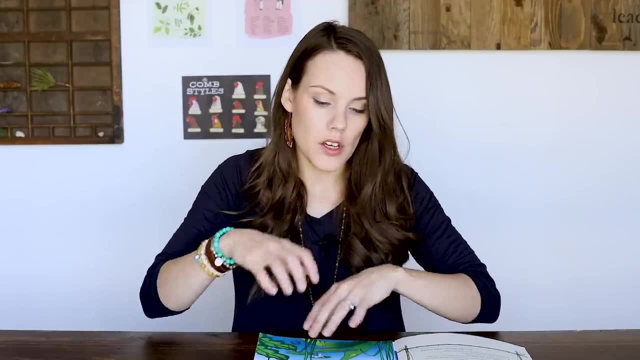 But this is the language three. So this is your grammar, creative writing and your dictionary skills. There's also spelling books and different things. So this isn't everything for language arts. There's their one on one. kind of books are a lot more affordable. 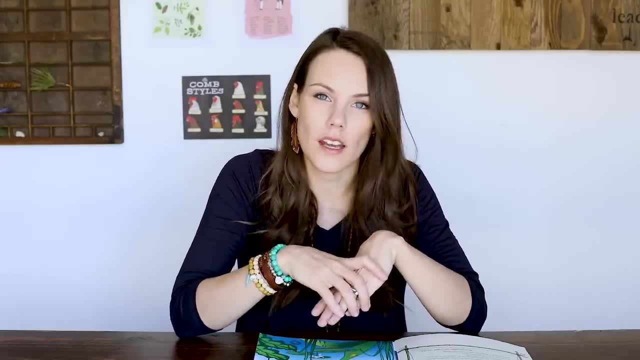 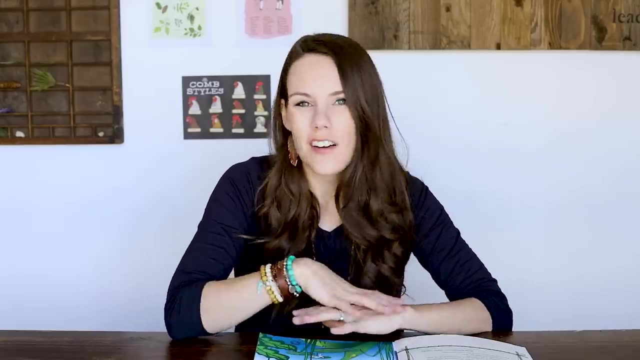 but generally you would want to get the package set so that you could get you know all of your different things: your spelling and your teacher's guides and your handwriting and all of that as well. So this is just going to give you an idea of a Becca in general. 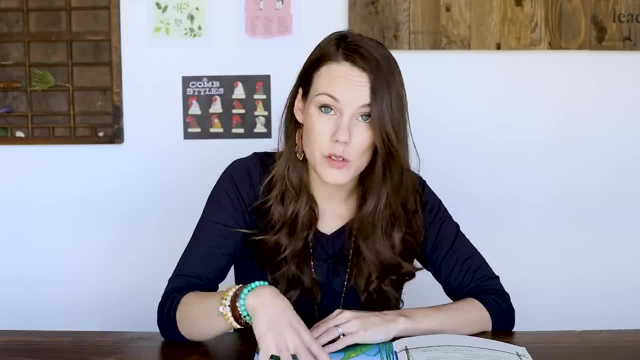 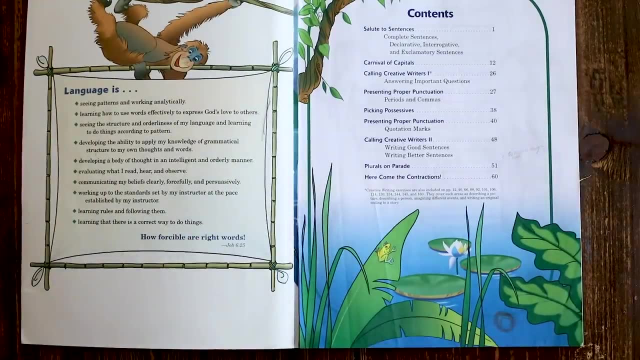 I'm not necessarily showing you everything, because they did not send this to me. This was the one that I had purchased, So this is the table of contents. We'll take a look inside again. Keep in mind, this is a hundred percent going to work well for families that are looking for something that's very 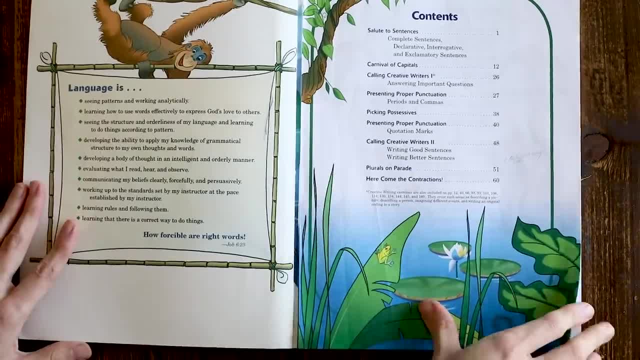 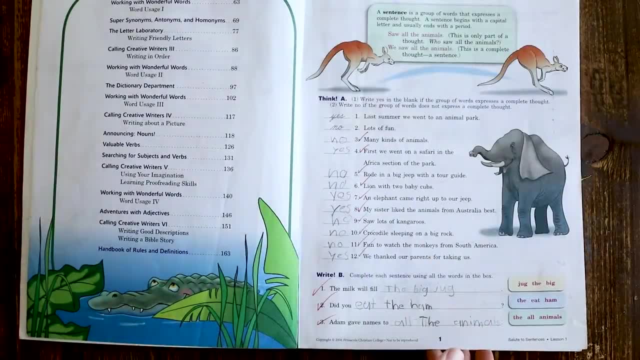 very independent Their kids can do on their own. You're not looking for anything, Charlotte Mason, unit study or or unschooling or any of that. You're not looking for any anything that's going to require a whole lot of you. 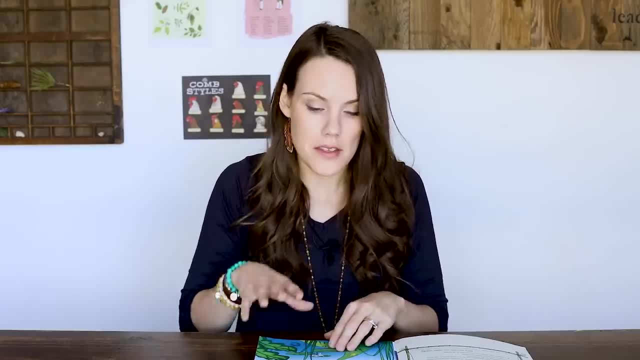 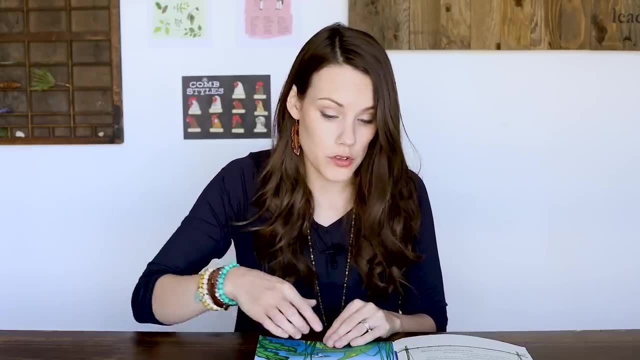 You're looking for something that your kids can just do and get her done, Then this is going to be a really good fit. It's also really bright and colorful and it works well for visual learners- often that do well with book work. So the table of contents. 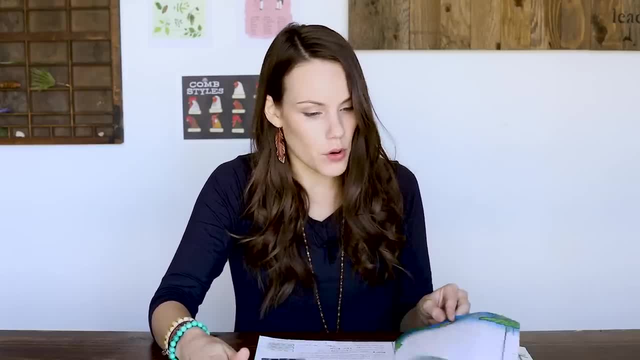 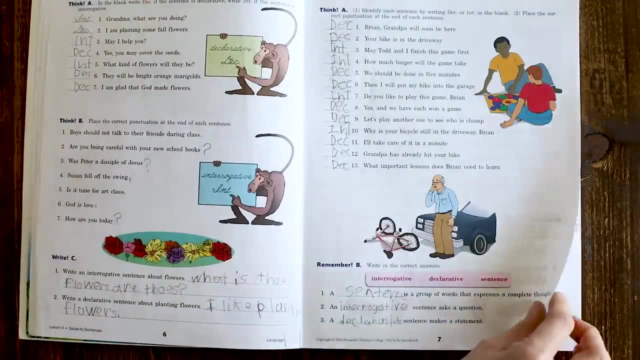 you can see some of the different things that are covered in the program, and then we'll just do a little flip through of the book as well, So you can see how it's laid out. A Becca is definitely a little bit ahead and advanced. 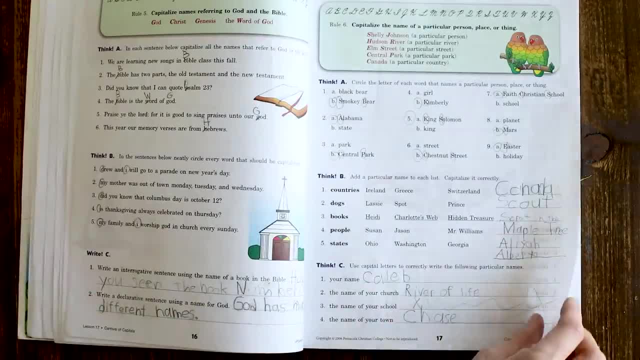 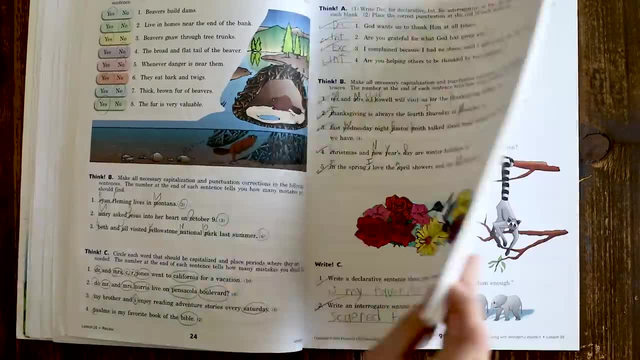 So I would recommend checking samples before you are purchasing, because, um, because you may find that you need to do a year down, If you're jumping into this somewhere in the middle, if you're starting in kindergarten again, even in kindergarten, 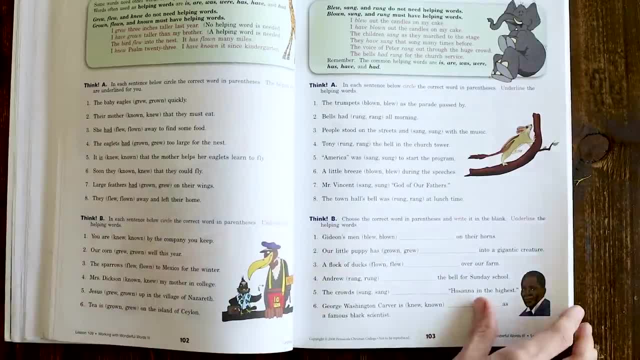 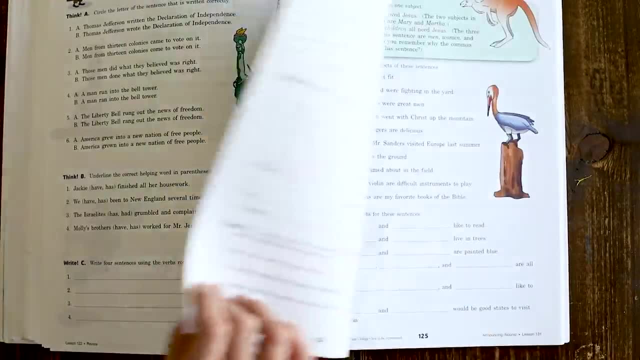 I have found that for a lot of families they can't start at that K five. when their kids are five, they need to start at that K four. So it's going to depend on um where your child is at, So keep that in mind. 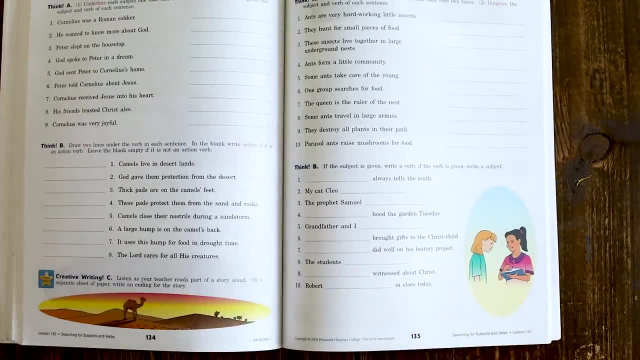 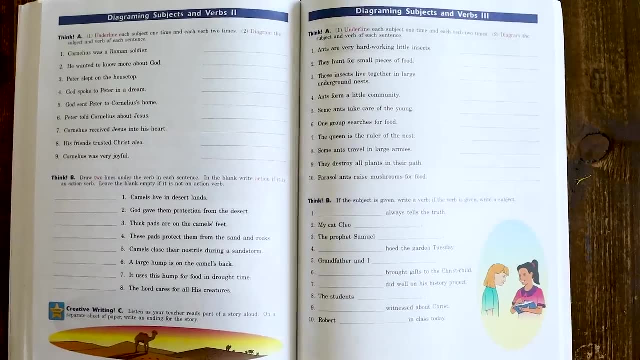 um, when you're considering this, because it is pretty intensive and their older grades go really in depth into grammar, So they're going to do like a couple of pages of this a day. Sometimes it's only one page a day, depending on the level or the age. 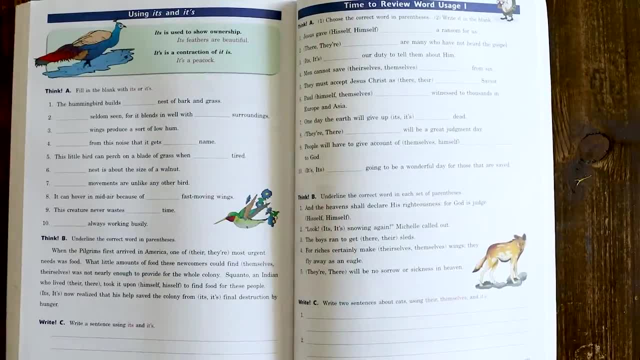 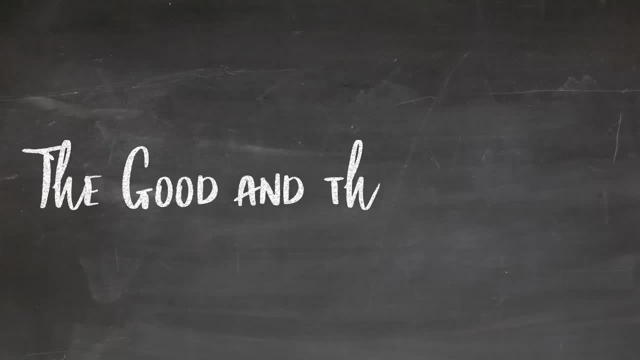 Um, but that gives you an idea of the way a Becca is laid out, So I wanted to make sure to include that one for you guys, so you could see what it looks like inside. The next one I'm going to show you is the good and the beautiful. 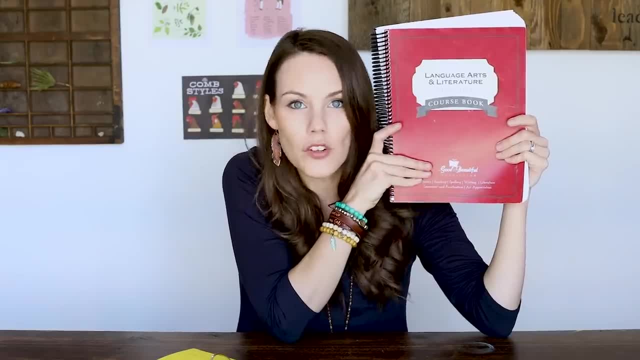 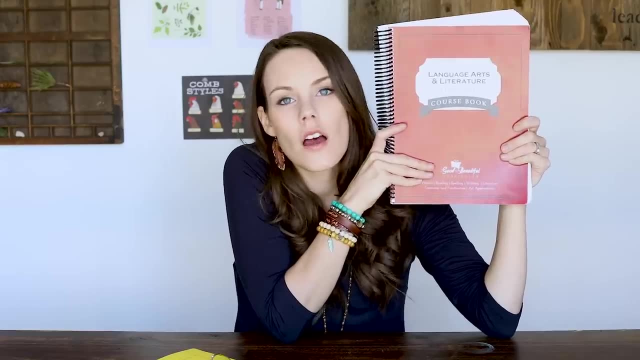 so this is one- you'll probably have seen a lot of my own posts about it and those are a lot more personal- of why we're not using this. so you can check that out. I'll make sure to link it above: Um. 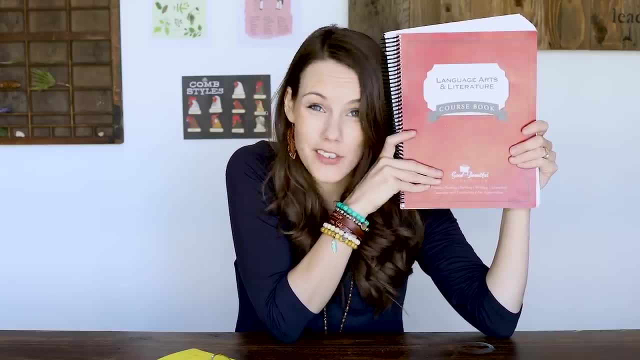 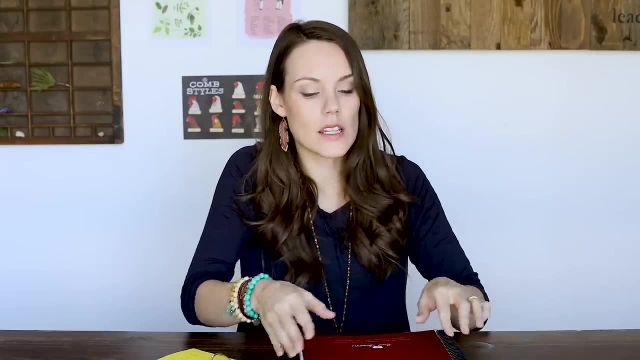 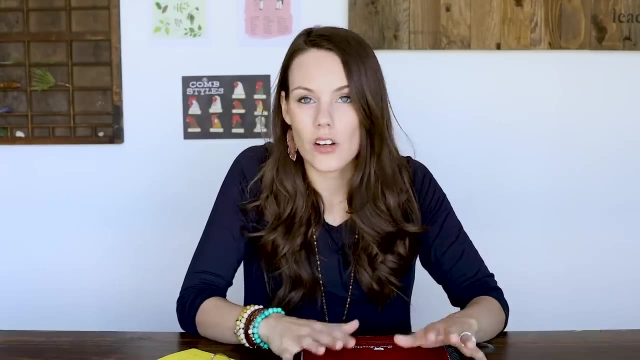 but I am going to show you inside of it anyways, and you guys can make your own decisions, And I wanted to make sure I included it as a comparison. So this is the um is. this is um written by somebody who is lds, so it is not necessarily christian. it incorporates: 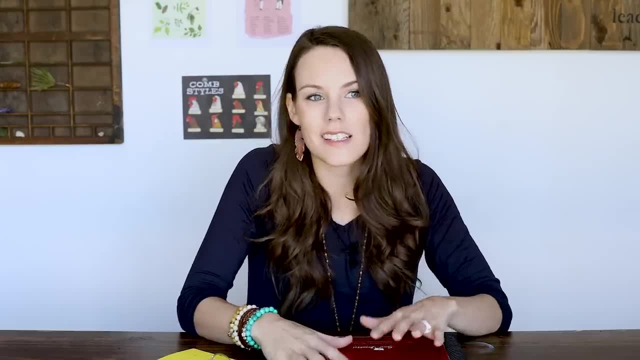 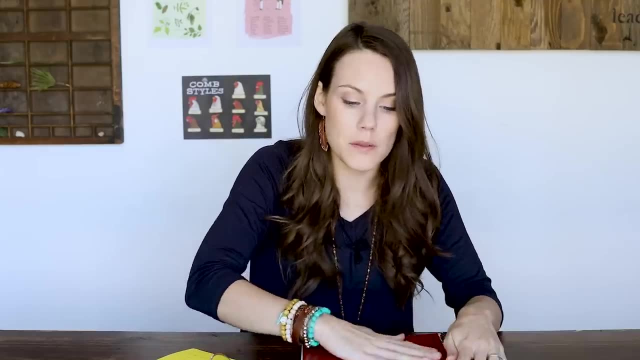 lots of christian values, but that's just something to keep in mind when you're looking at this. it's not secular. for sure you're not going to want to use this. if you are a secular family, it it has god all throughout it. so just keep that in mind, depending on if you're looking for christians. 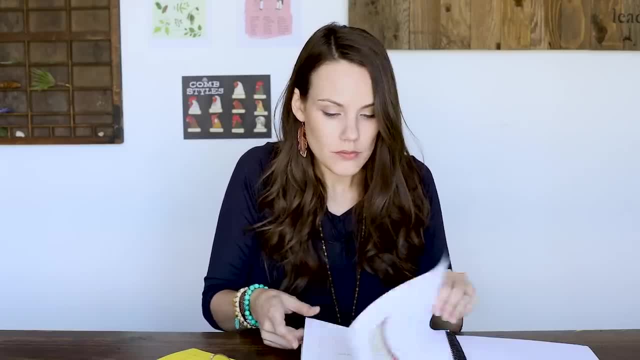 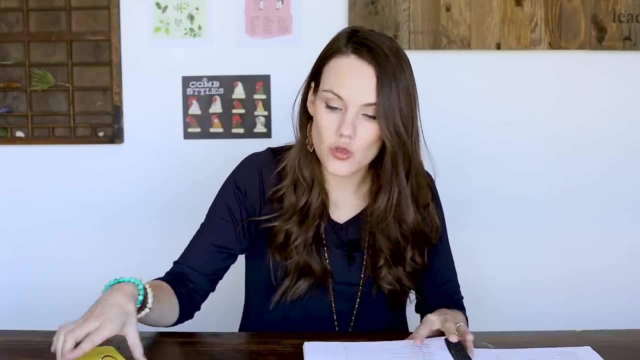 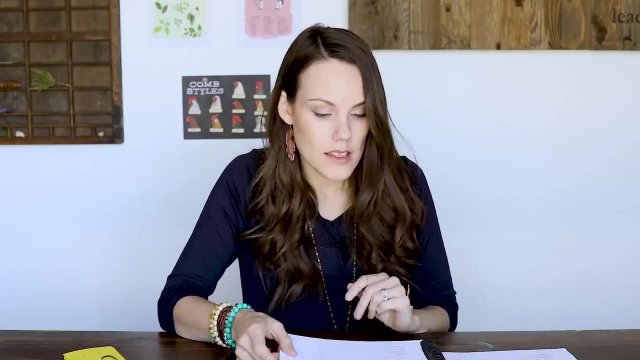 or secular. so when we look inside, this is probably more focused on, like classical slash, traditional model of education. so if we look, i'm going to show you the table of contents here so you can see the way it's laid out. this comes with a reader and it comes with some flash cards. 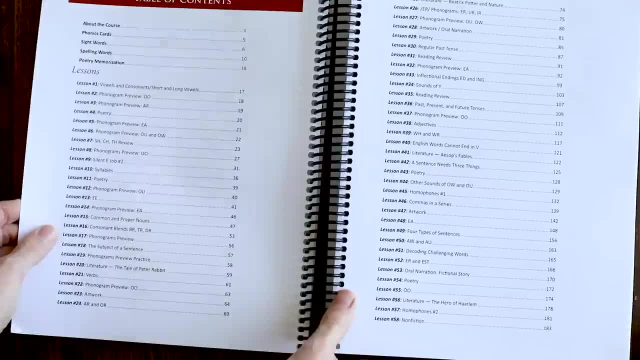 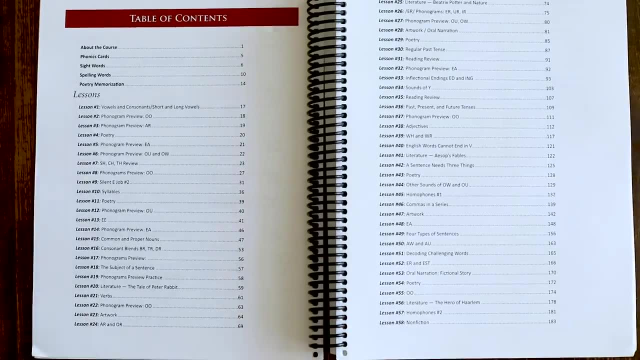 as well they're going to be working through and there also is, just like a teacher, a little hand book, but not necessarily a teacher's guide. you're going to need additional resources for a lot of their, their things, whether it's readers, you're going to need to go and buy. 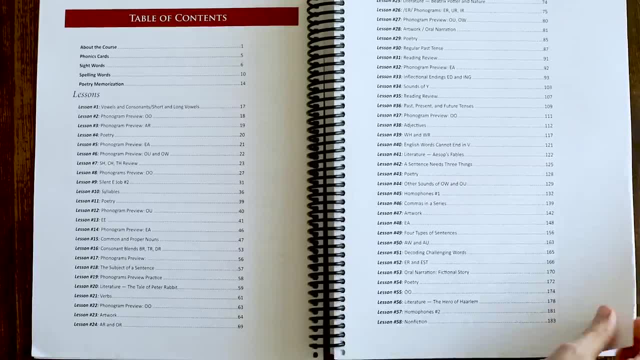 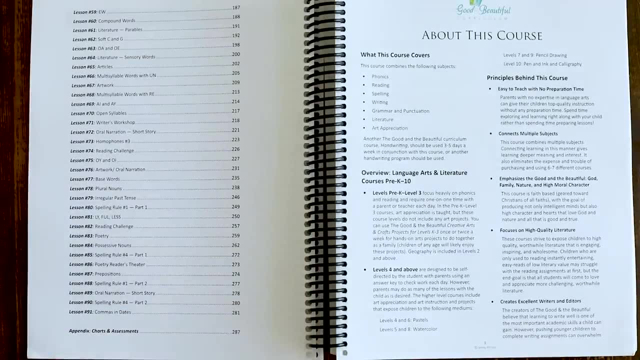 um, there's some. there's some art supplies and stuff like that, because it does have some art in there, especially as the kids get older. so if we move forward, i'll give you kind of a flip through of it. there's spelling lists, there's reading words they're going to be reading through. 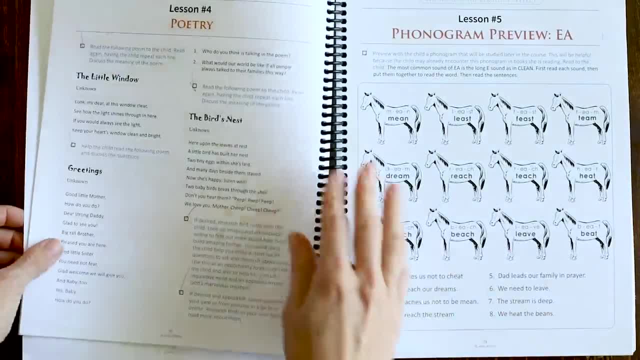 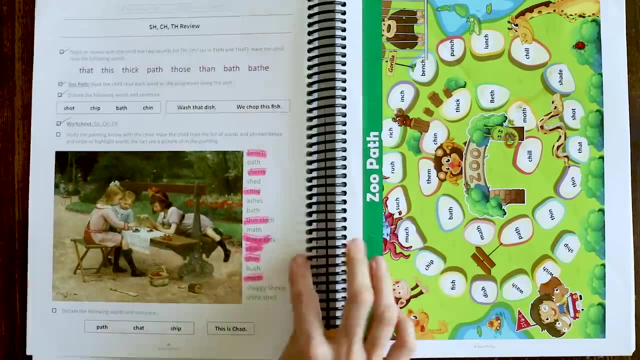 um, that's all kind of at the front here, and then their lessons are laid out. now, this is the level one, but it's going to be a little bit more complicated because it's going to be a little. it's laid out, it's got poetry, um, and it's got. you know, it's very in-depth, very in-depth with. 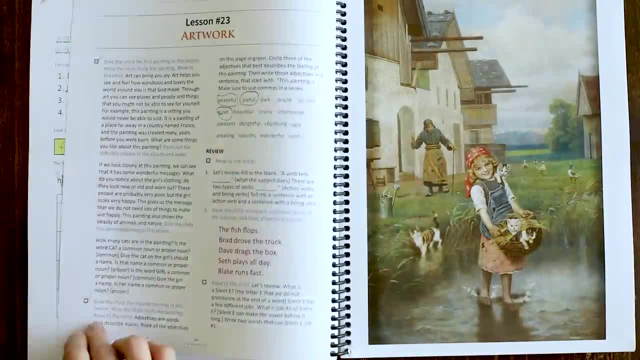 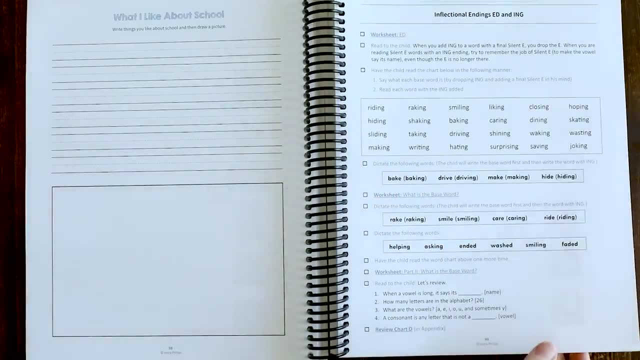 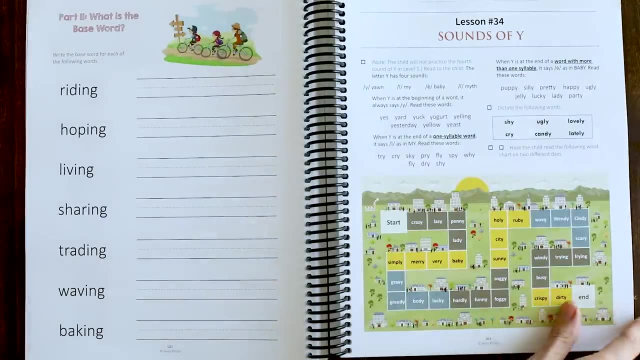 your grammar. it's got picture studies, but it is still laid out more as something that is traditional slash kind of classical. it is not necessarily um, as as project-based, it's not necessarily including, you know, the music studies and all of those other things as well. so, depending, 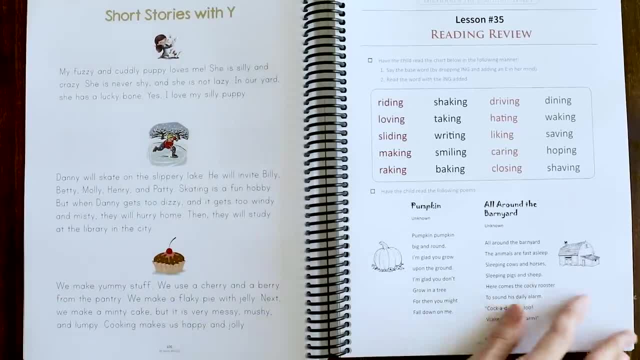 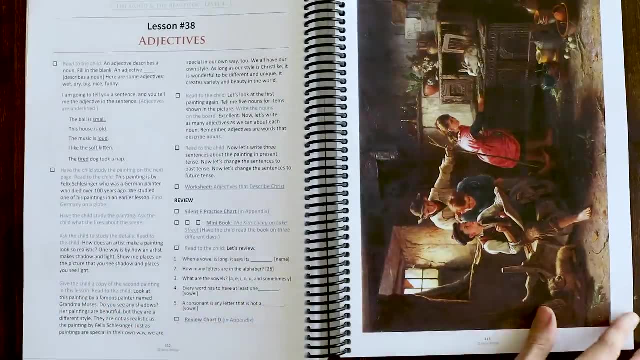 on your homeschool style. those are just things to keep in mind. so that is the course book. the other thing to keep in mind is that it is teacher-led in all of the like level three down. so depending on the age of your child, it's teacher-led. 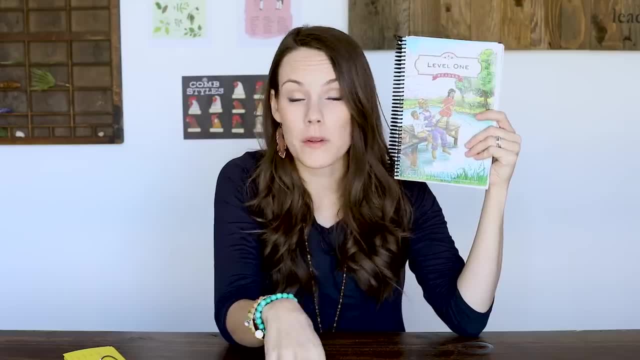 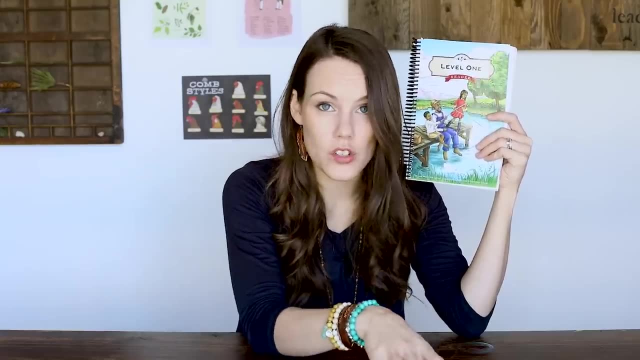 also you are going to be. it recommends doing it for 45 minutes to an hour for their language arts. they're supposed to do five minutes of their flash cards. you're supposed to do five minutes of their sight words. you're supposed to do five minutes of their spelling words. they're supposed. 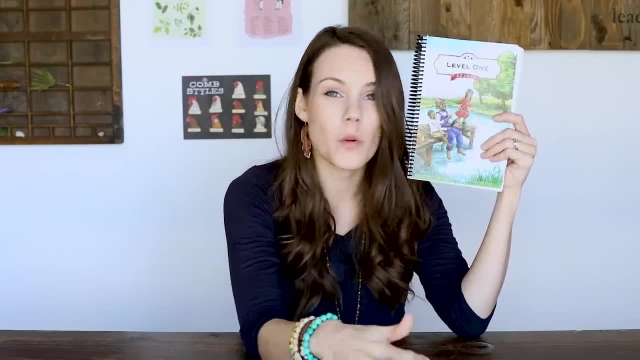 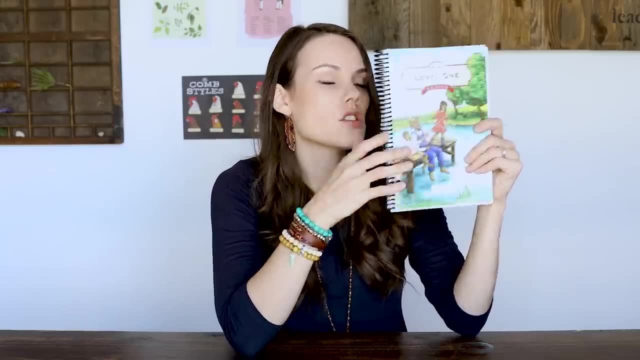 to do 20 minutes of their reading, and then they're supposed to do about 20 minutes or so of their course book, and then you just kind of stop at that point. so that's the way that it's laid out right now, and so it's something to keep in mind if you're looking for something. 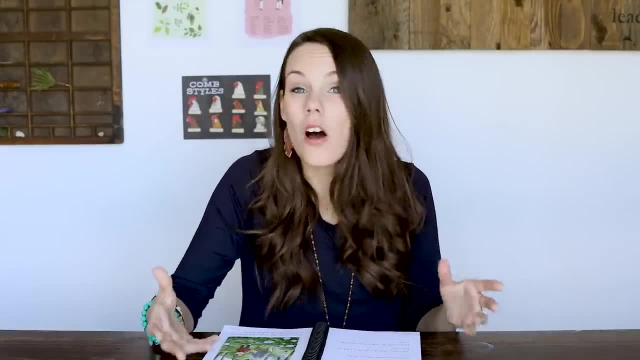 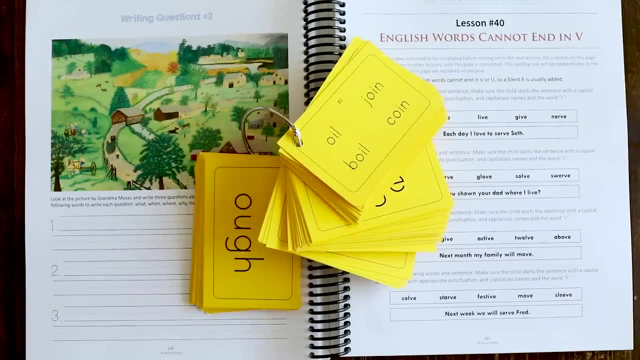 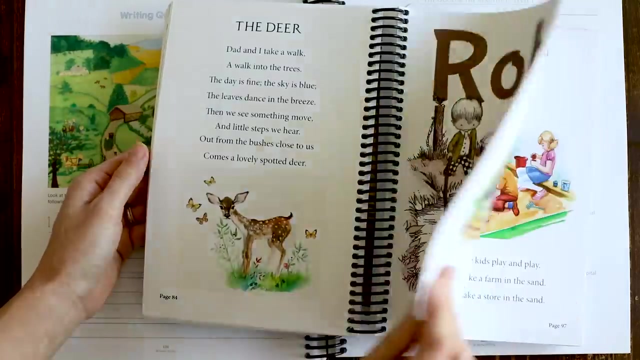 that is, is not as um, it doesn't take as long or is more adaptable to be used within the entire family. there's lots of other considerations there, so they also have a reader included with it that your kids will do. so that gives you an idea of what is included with the good. 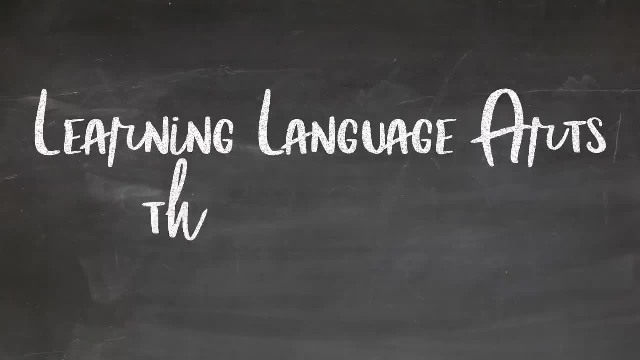 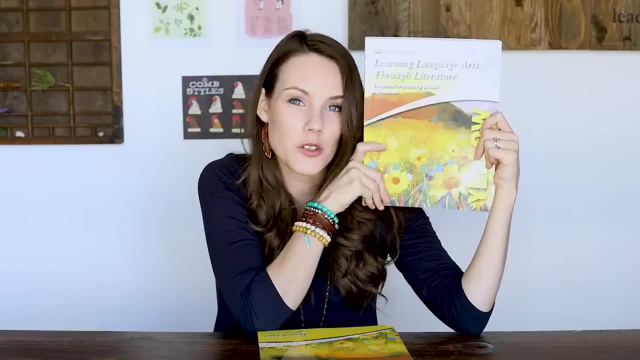 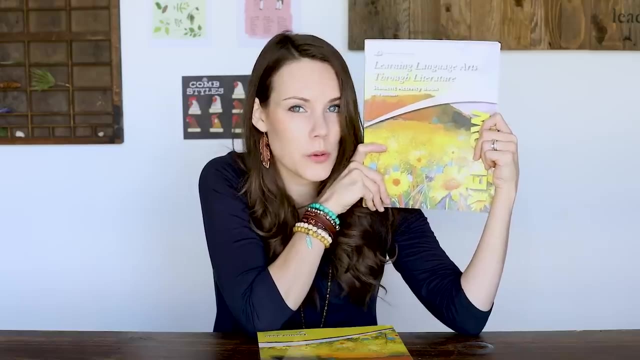 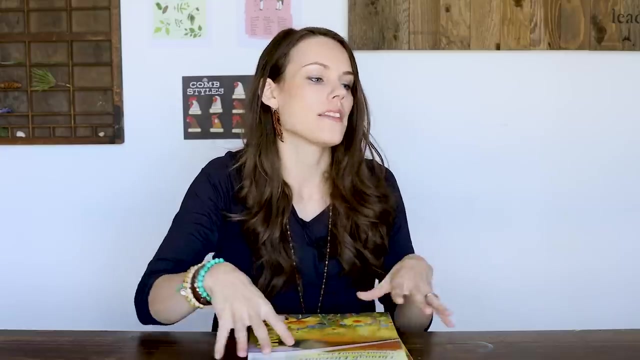 and the beautiful. all right, the next one i'm going to show you is learning language arts through literature. now, this is a very interesting and unique program, probably very set apart from almost everything else i'm going to show you today, in that there's not really a whole lot that does it in this unit. 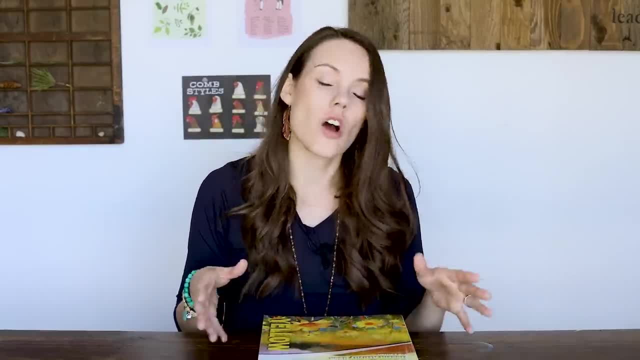 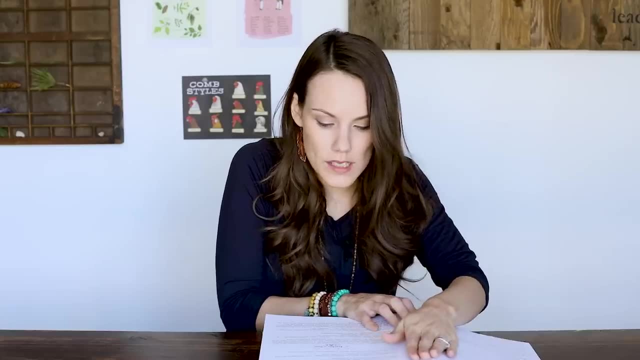 study kind of approach, um, and i i could talk about it or i could just show you, because you're going to get to see some of the things that i'm going to show you today and i'm going to show you very quickly how it's laid out. so you are going to be using literature, books that you will get. 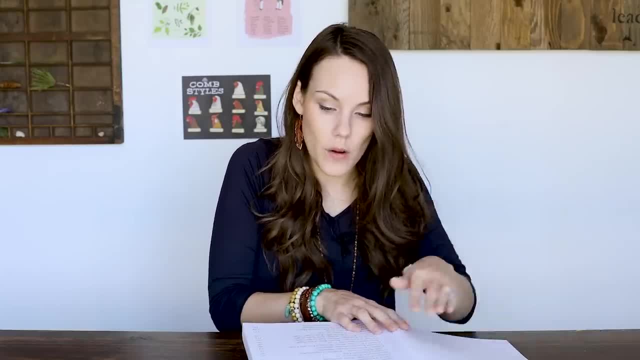 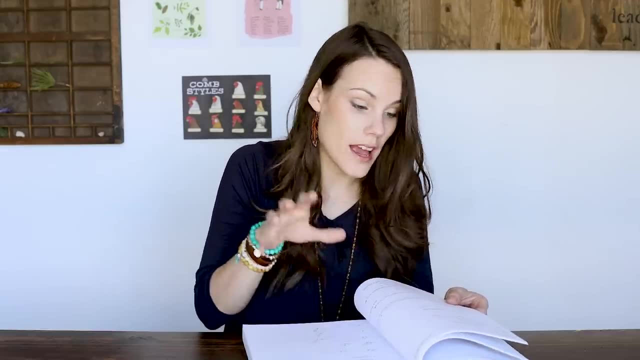 either on top of this um and it, it tells you what those are and you are going to be learning your language arts, every part of your language arts, through. there's handwriting, there's grammar, there's spelling. everything you're going to be learning is comprehensive. you're going to be 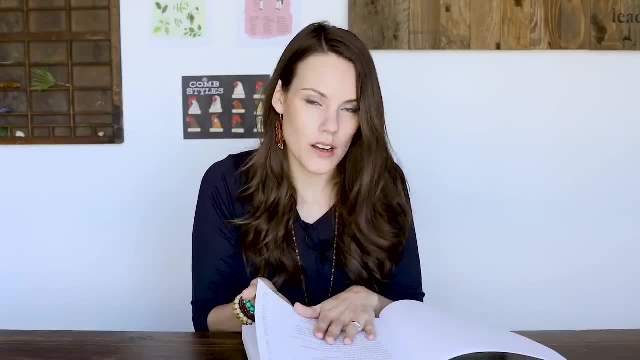 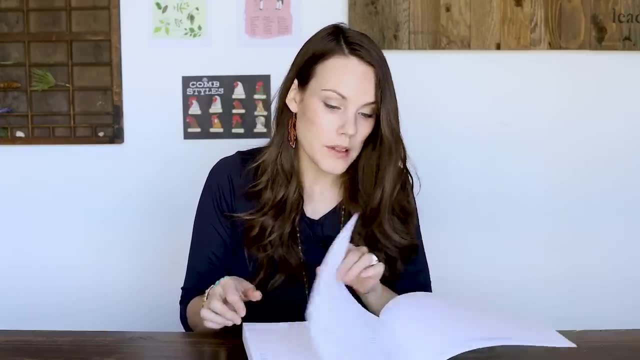 learning that through the reading, through the literature component of the program, which is really, really unique, everything is here that you need, so in that way it's relatively affordable. um, let's take a look at the table of contents here so you can see what they're doing. so you can see basically they're reading these stories. 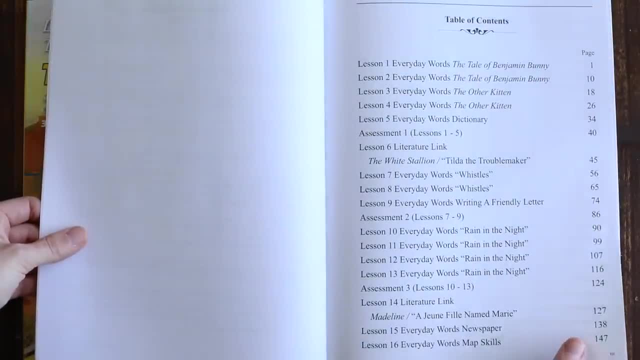 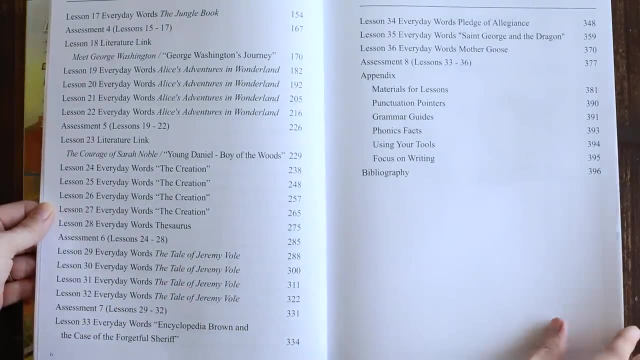 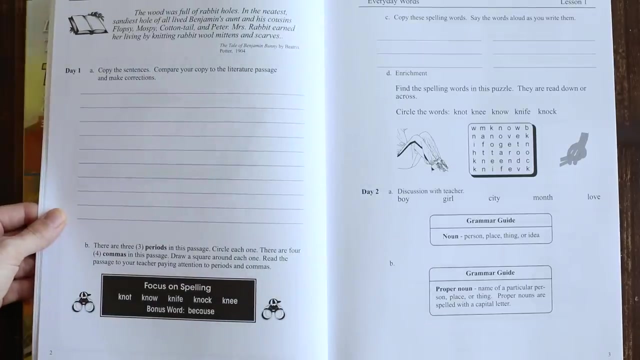 and these are the different ones that they're going to be doing throughout the year, and then there's additional resources in the appendix, so if we just do a little flip through, you can get an idea of how it works. so they're going to be doing some reading. they're going to 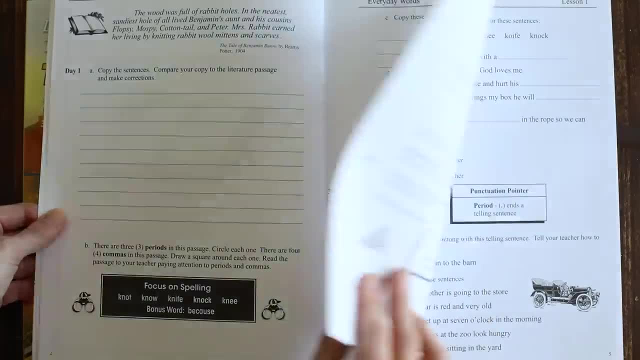 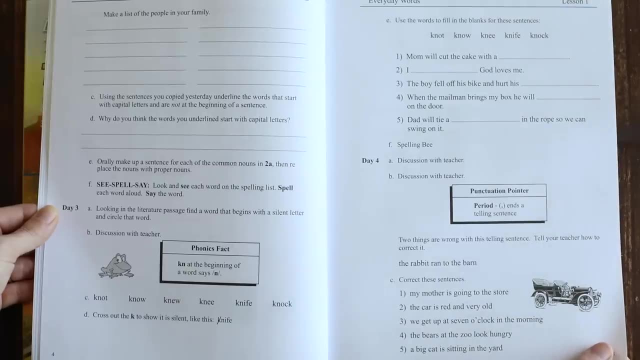 do copywriting. they're going to be doing some reading. they're going to do some reading. they're going to do some work. they're going to focus on some spelling, in that they're going to have a discussion about different nouns and proper nouns. they're making lists. so it is definitely still. 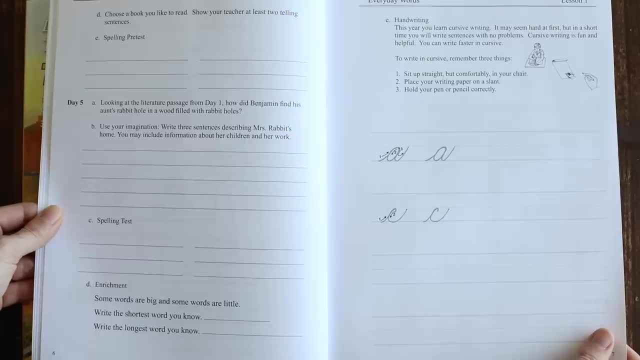 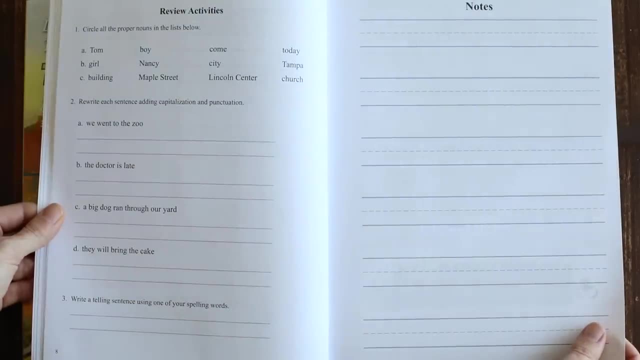 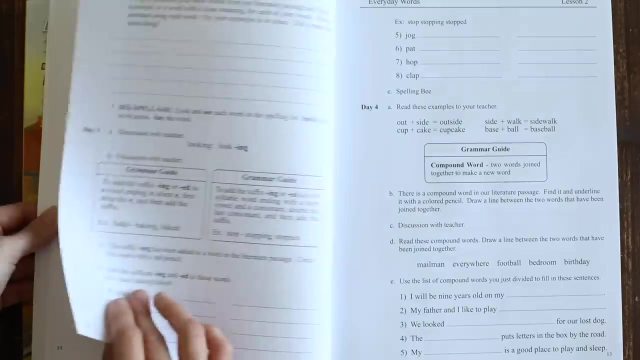 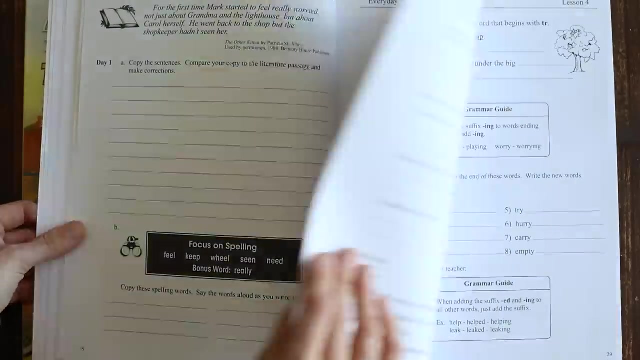 teacher-led- another thing to keep in mind. i'm going to show you the teacher's guide as well, so you can see how that is laid out. there's handwriting, spelling tests, notes, review activities, and then you're on to another lesson with reading and different things. so it incorporates everything through literature, and i think that is a really unique way of teaching. 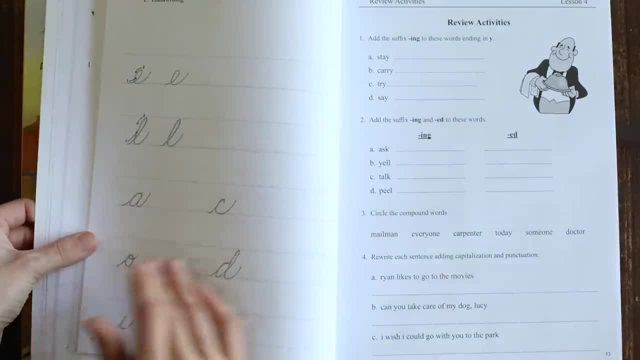 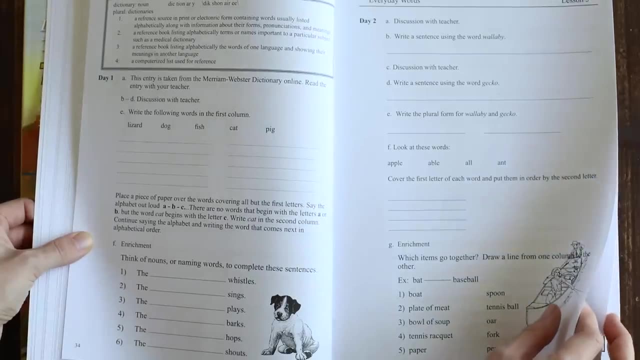 language arts. so if you're looking for something that's all in one, let's just kind of read this book and then here's the discussion and here's how to teach from that. then you can see that this program is going to be a good fit. there are also some um. there are some of the stories that are: 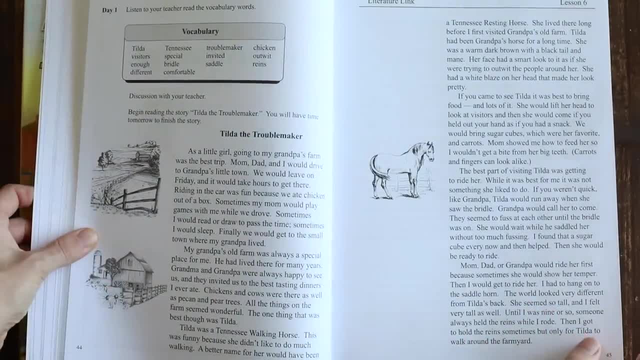 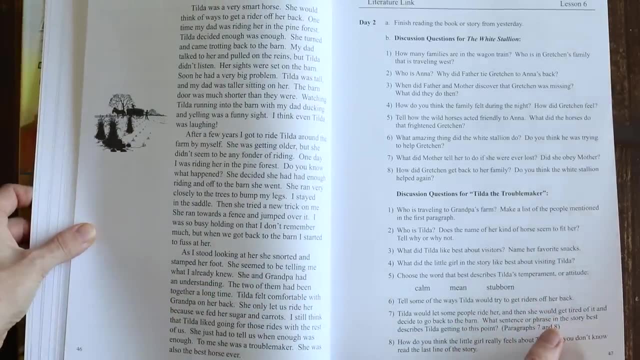 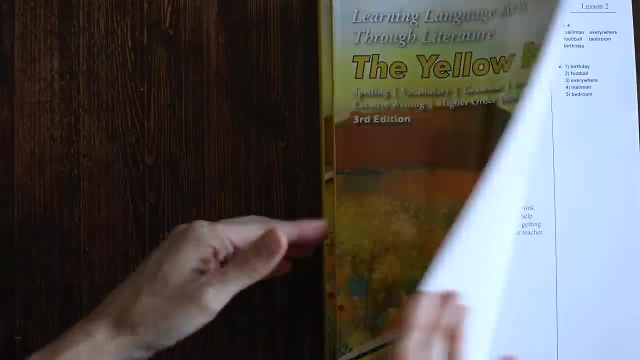 right inside the book, so you'll read that story and then you'll have discussion questions on it and continue to work through your literature components, which is super cool, okay. so inside the teacher book, it really teaches you how to use the program and and why it's laid out the way it. 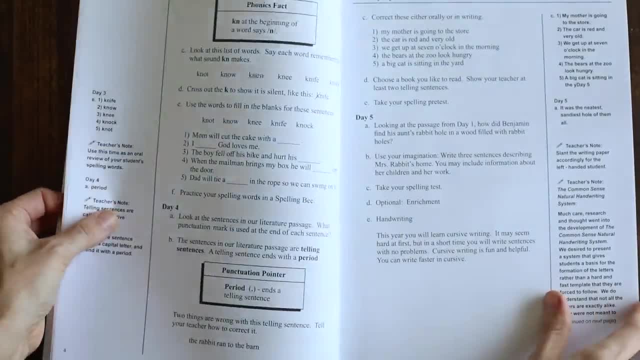 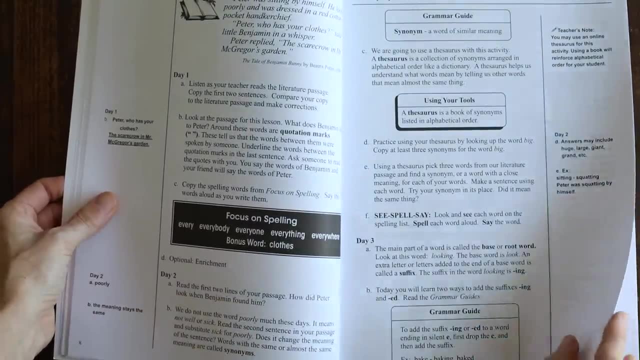 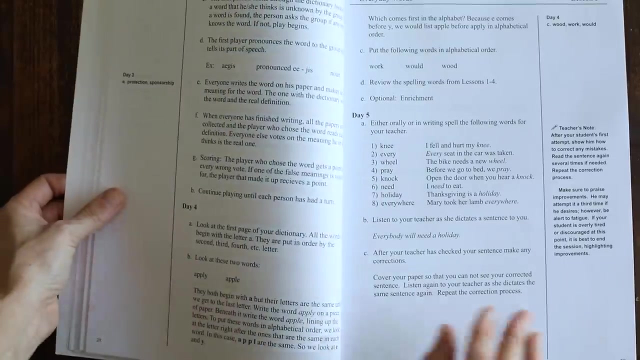 is and how it incorporates journal writing and handwriting and review and creative writing and all of that stuff. the table of contents is here as well, but it's very similar from the other one, so we'll just flip through it. um, but inside here it actually tells you now what you're going to do when you are teaching, so you'll. 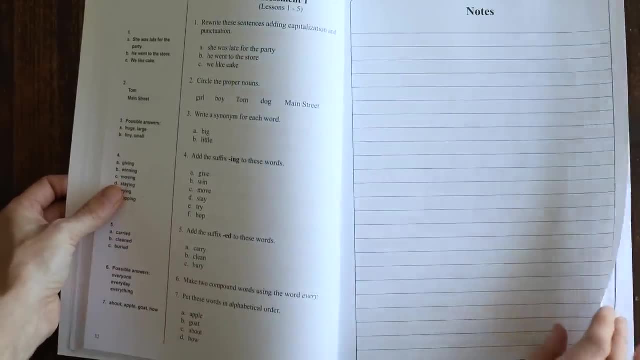 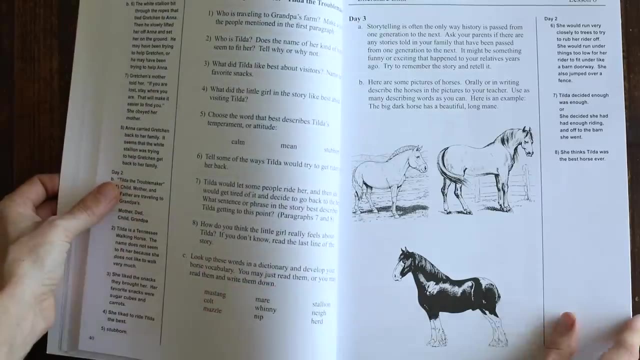 see, it's kind of scripted. there's teacher notes on the side, but you can also see what the child is doing here, so that you don't have to be flipping back and forth between your child's book and your own. so this program is going to work well. if you need something that has, you know the workbook. 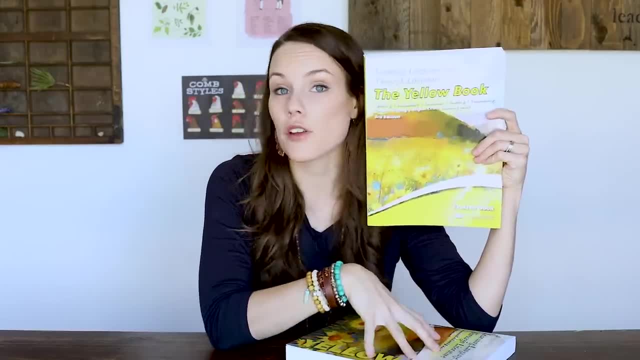 component. it's going to work well. if you need something that just has everything in one book, you don't want to get grammar, you don't want to get spelling, you want everything in one. this is going to work well. it's going to work well. if you don't have a grammar book, you don't want to get. 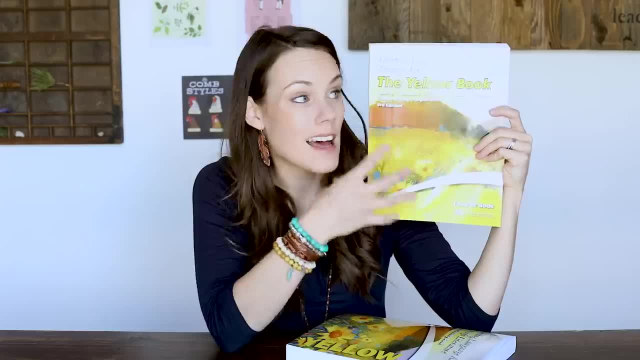 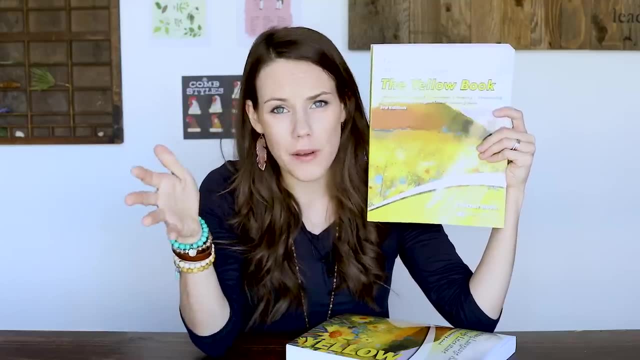 grammar. it's going to work well if you want to teach through literature, because that is exactly the entire title and approach of this book and this curriculum. so it goes all the way up. it has everything there. there's multiple levels available, so i would recommend going and checking it out. 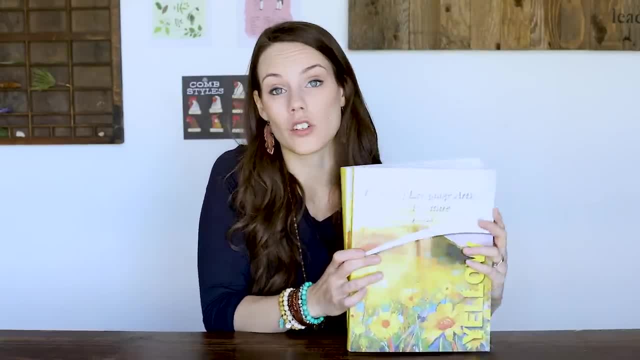 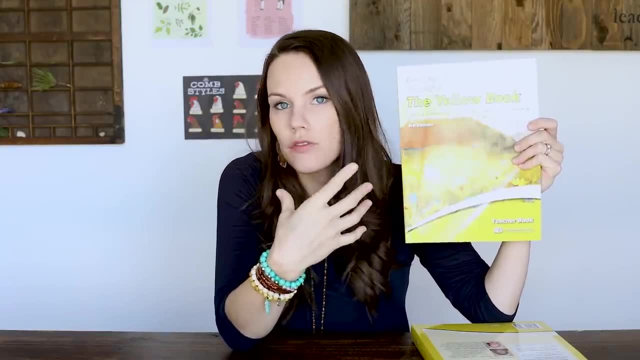 and considering this if you feel like that is going to be a good fit. so the program is not necessarily secular, but it doesn't have a lot of christian approach in the way that it's taught. it's mostly just the way that it's taught and it's not just the way that it's taught. 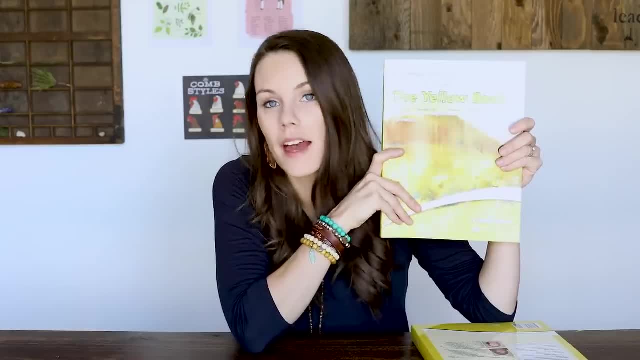 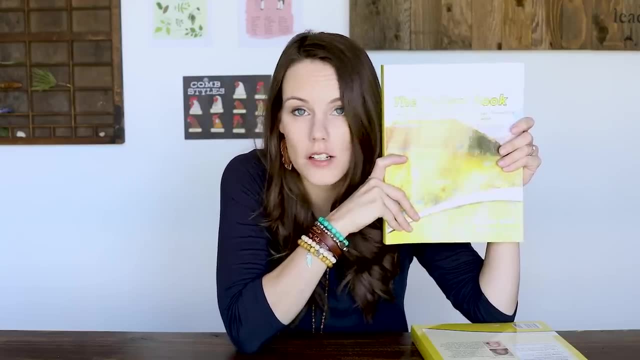 literature that you're using. there are some bible stories throughout, so, depending on how you feel about that or not, i've seen some mixed reviews. some secular homeschoolers have used it and thought it was fine, and others absolutely not. so something to keep in mind. it's definitely a gentler approach. 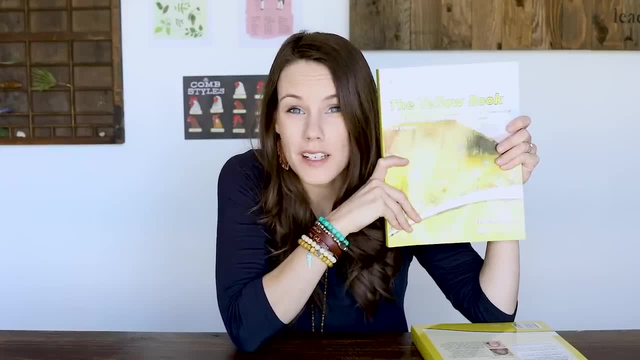 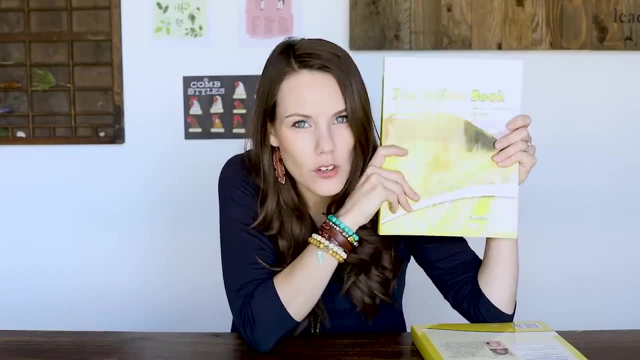 so if you're looking for something that's more challenging, or you are looking for something that is more, like i said, free and exploratory or charlotte mason inspired, then this probably won't be a good fit for you. it is relatively affordable, so just different things to keep. 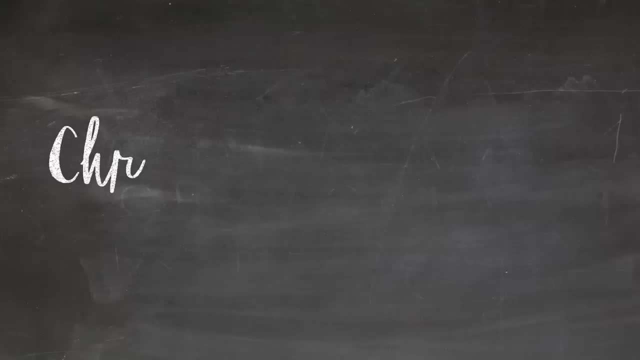 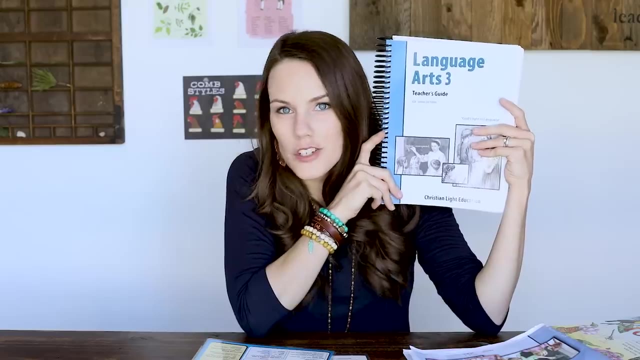 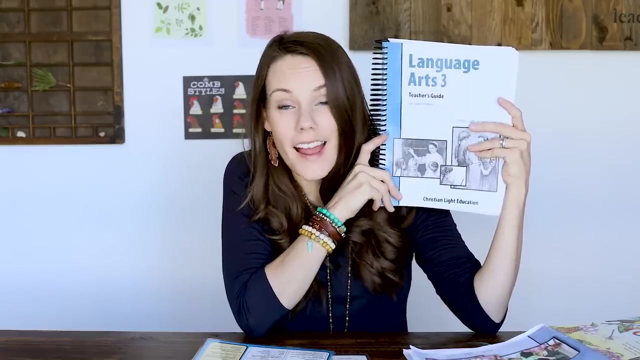 in mind when you're considering this program, so i would recommend going and checking it out. this is your language arts curriculum. the next one i'm going to show you is from christian light education. so these are their light units for language arts and i have to say we've been incredibly impressed with these. we've 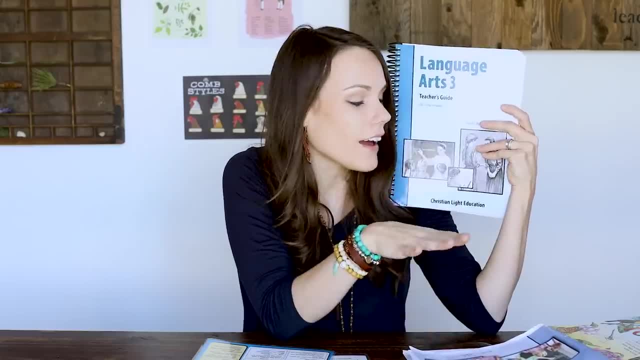 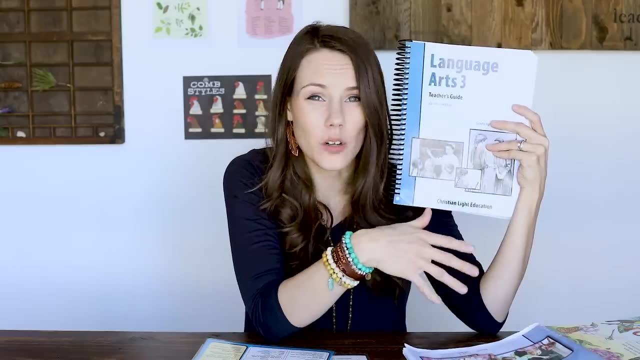 actually been using them ourselves. we were sent these from the company for free and we have been trying them out with my daughter at a reduced- so she is in a higher grade level. we've been trying a little bit of an easier one and we've been trying them out with my daughter at a reduced. 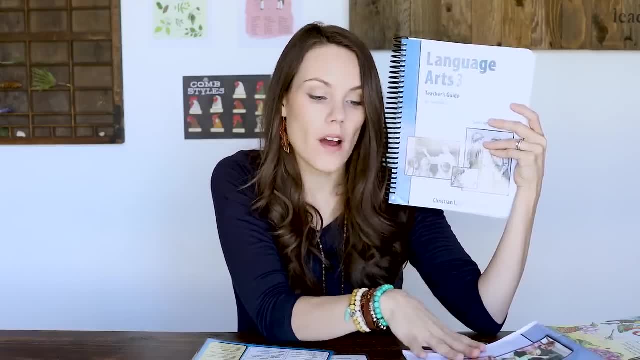 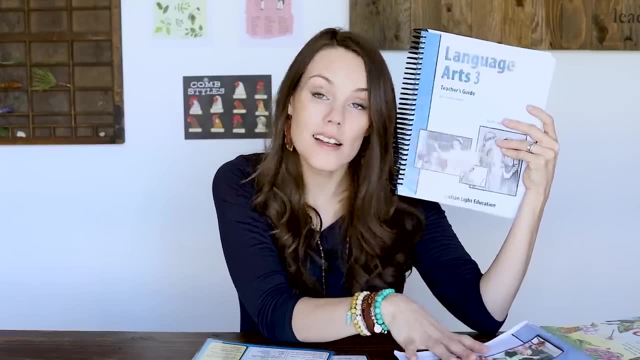 so she's been trying it out to see how it works for her. she likes something that's more independent, that she can do on her own to build her confidence, and so because of that she is thriving using these and incorporates your spelling, your grammar, creative writing, your handwriting, everything. 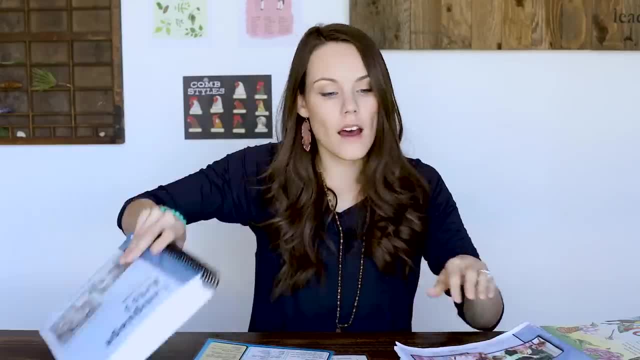 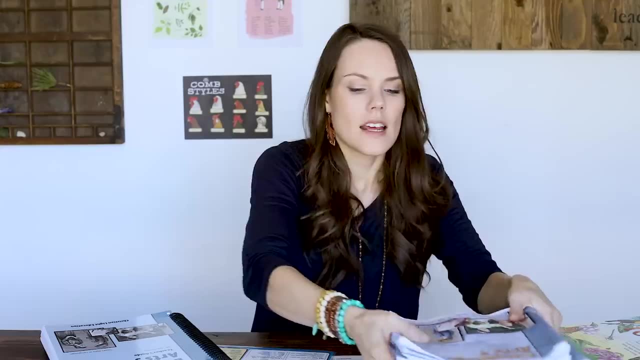 all within one book and it is very similar to alpha omega, where you have your light units they are called. so there are 10 of them, so they're working through one a month. it's not necessarily as bright as the other ones, but it's definitely more on the advanced side, so she's been trying. 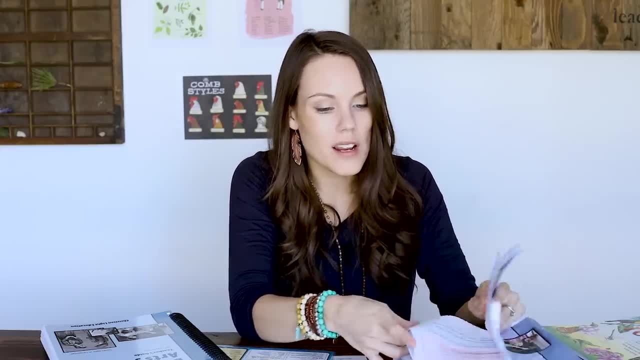 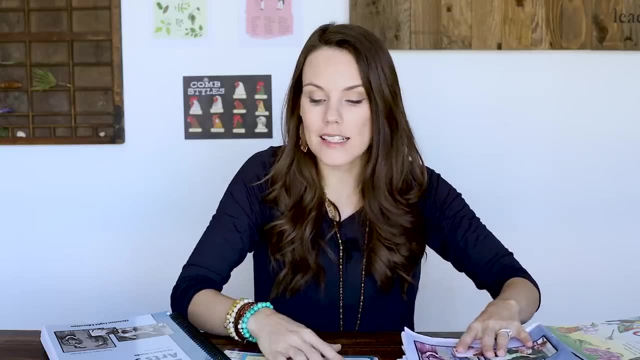 to keep up with all of her classes. it's very simple, which i think is in some ways a benefit, especially for visual learners. though they like that stuff, it sometimes is a bit distracting to them. so let's take a look inside and see, obviously, christian light education. it's incredibly christian. 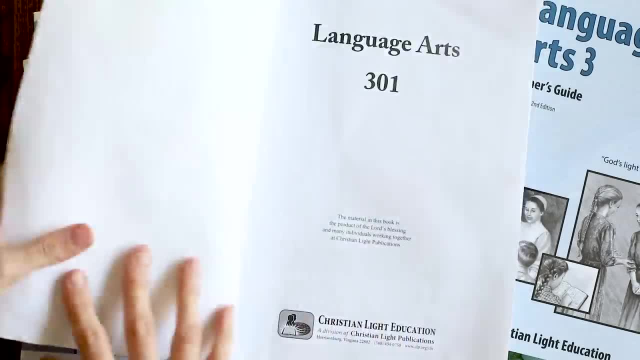 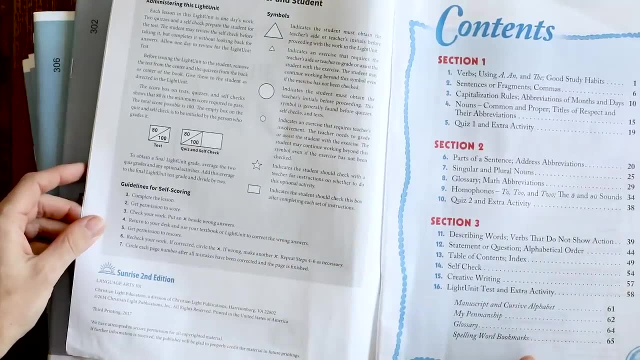 based, so that's going to be built into absolutely everything they do, so i'm going to show you inside a sample unit. here's the table of contents. this is the grade 3 version, so she's already finished this one, but you can see the different things that she's done on here, so i'm going to show you. 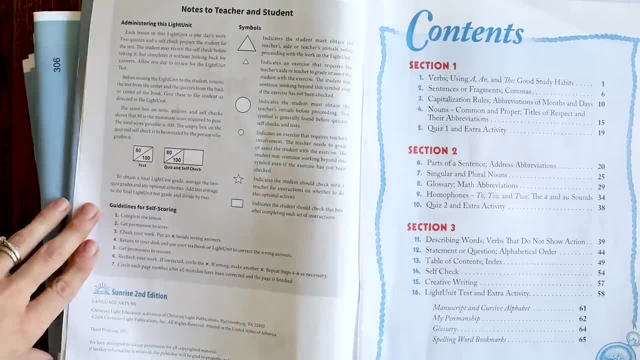 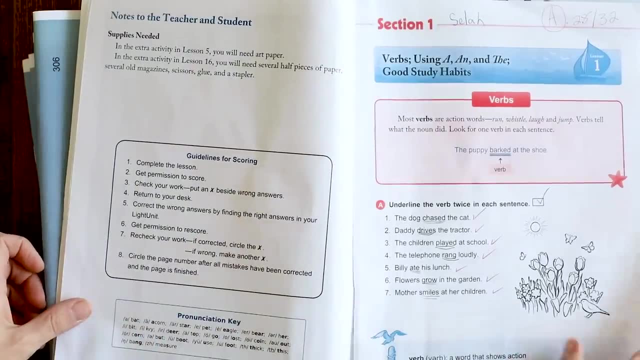 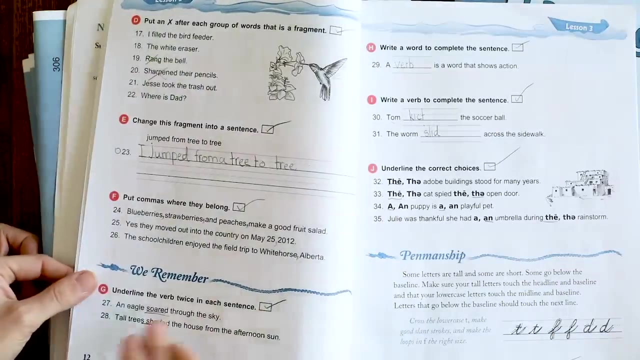 that they are going to be doing, and then we can do a little flip through so you can see it is done by her almost entirely independently. she even marks it herself, and then I just help her and mark her tests for her. so if you are needing something that can be done more independently, then this is going to be. 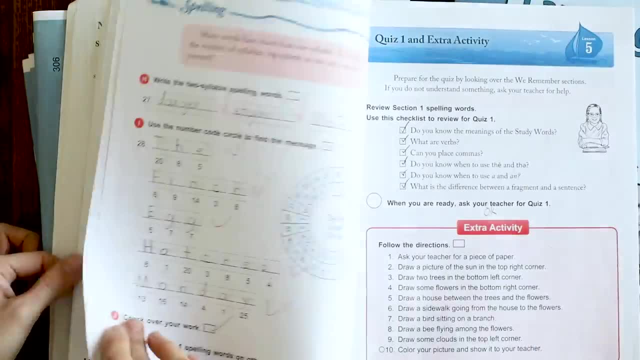 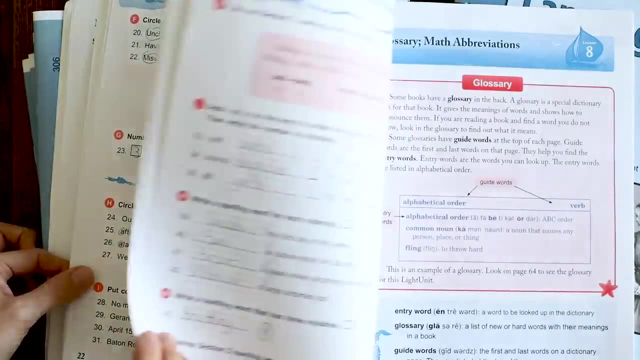 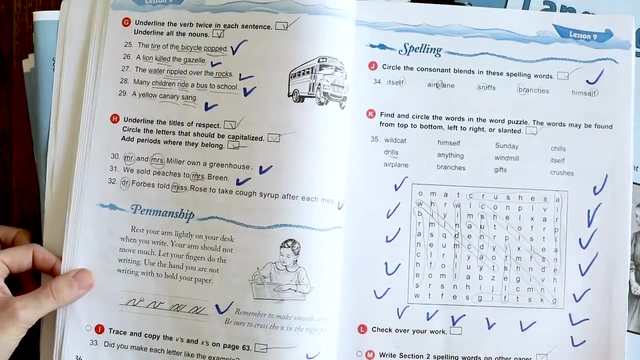 probably something that is a good fit for you. it's also obviously very traditional in its homeschool approach. this is not Charlotte Mason, it's not a unit study. it is a traditional curriculum where you open and go and fill in the blank and underline, but I think that this approach works really. 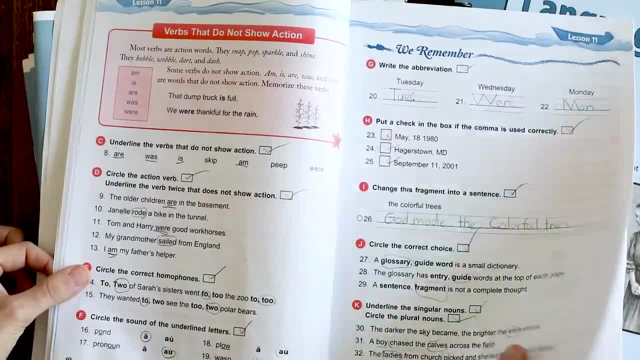 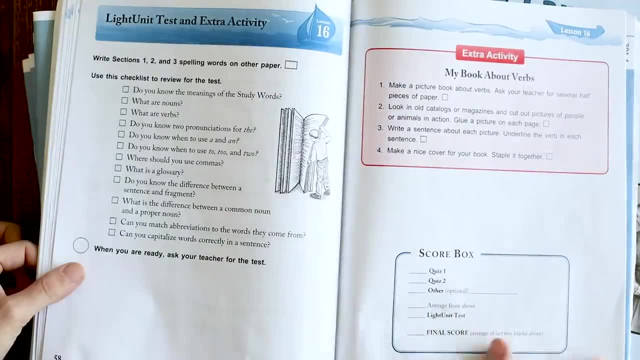 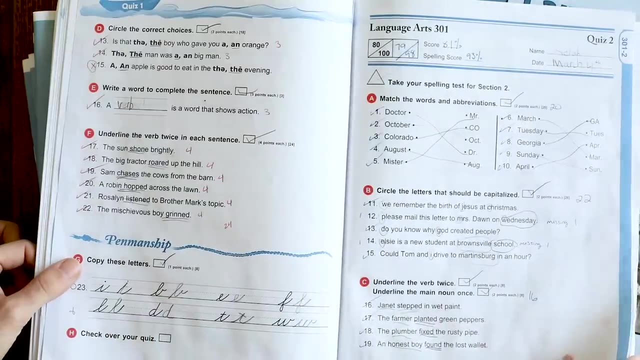 well for some kids and it is working very well for my daughter, so so this gives you an idea of some of the different things that are included. you can see how spelling is all throughout. they have a spelling list and at the end of every week they have a spelling test. grammar is built right into it and then 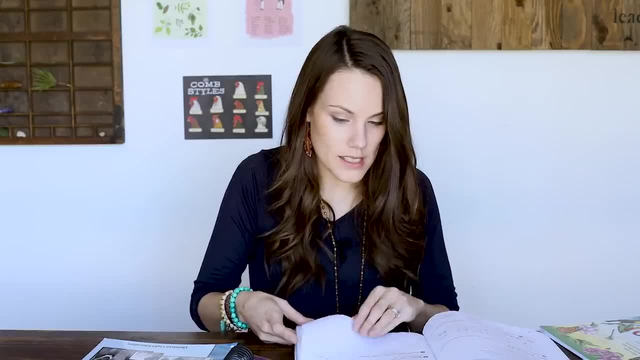 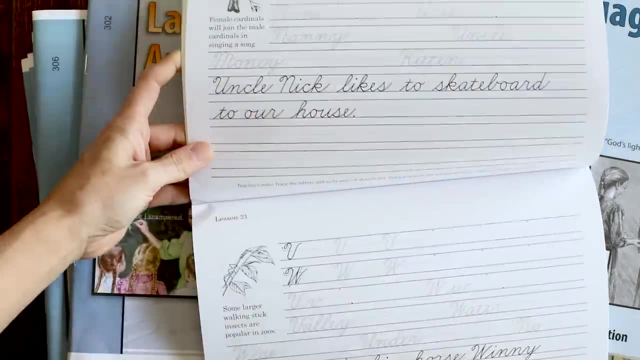 at the end. they're is a test that they do for this entire unit and then they are ready to move on. so you'll see there's handwriting here at the back. as they get on, they start to use this cursive book which was sent with us, so it actually includes: includes: 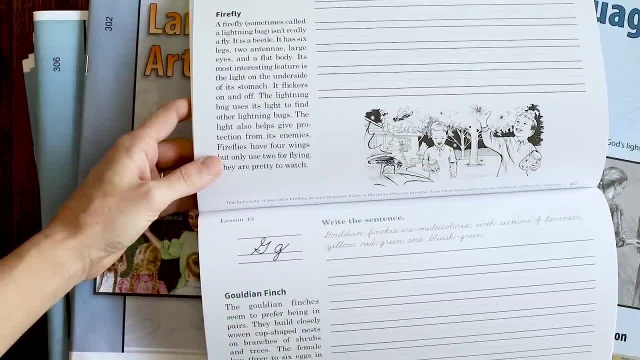 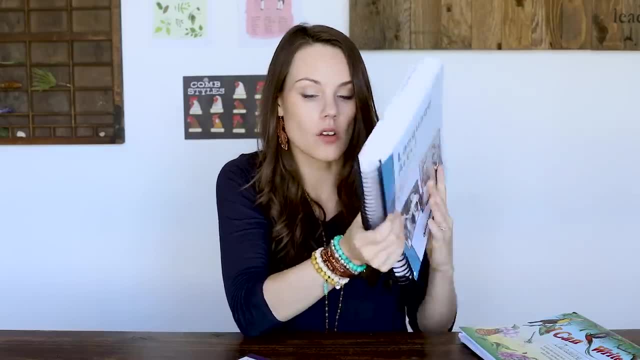 cursive writing, which I love, and then there is a teacher's guide which has all of your answer keys and everything in it and it actually shows you the exact page. so, as well as how to grade and all of that different things, so it is laid out. 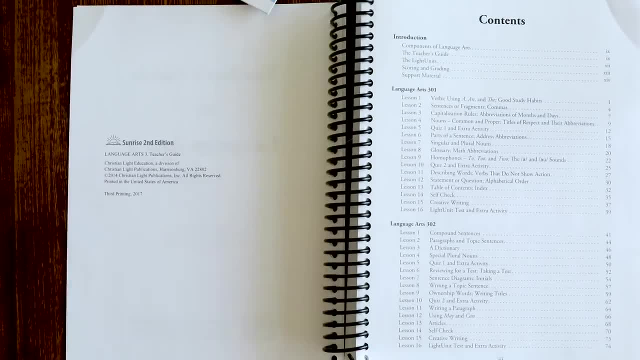 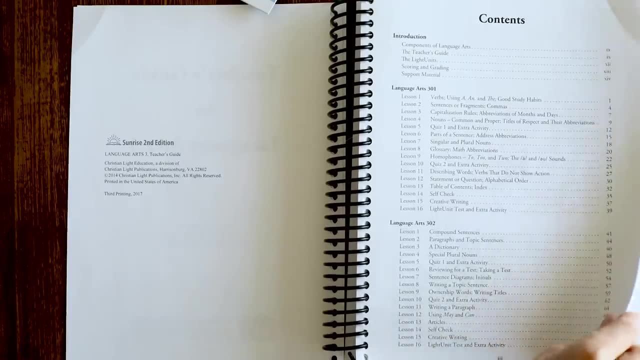 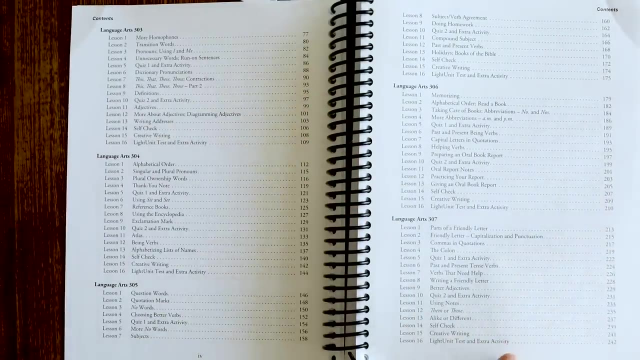 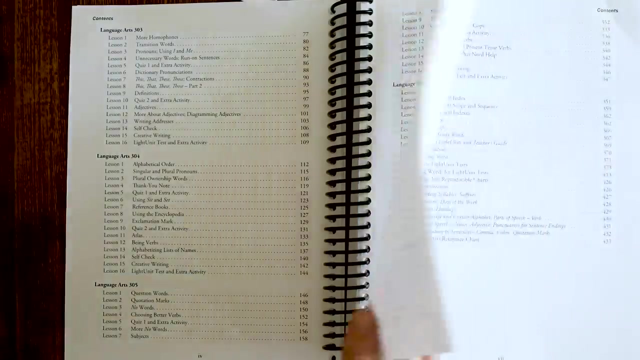 very, very well. I'll show you inside here so you can see the entire year at a glance. so 301 is the first unit, 302 is the second. so take a screenshot if you want to see this up close, because I'm going to be moving faster than you can probably read all of them, but you'll get. 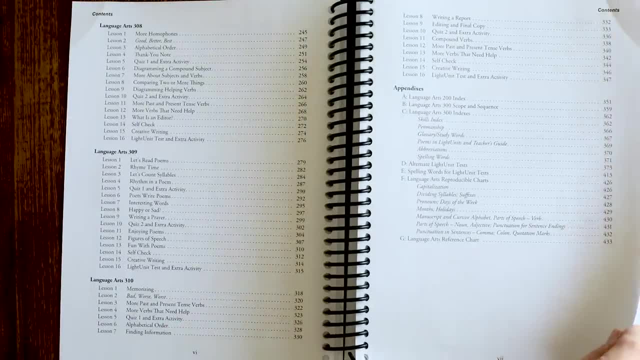 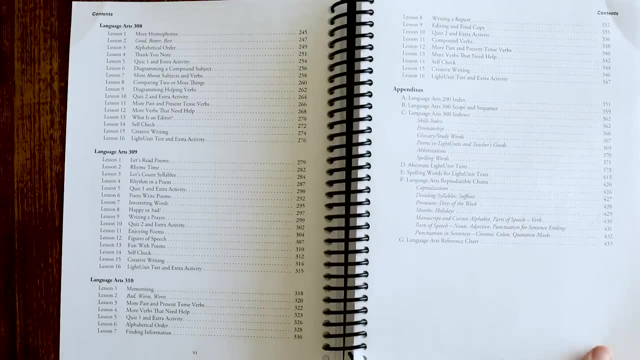 to see all the different things that are included and it's just giving your kids a very simple way of open and go and go through their language arts so it teaches you how to use it, how to score, and then you can see there's little kind of lessons as well, as you can see the 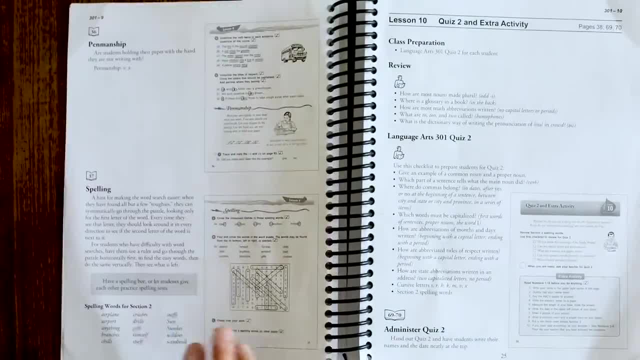 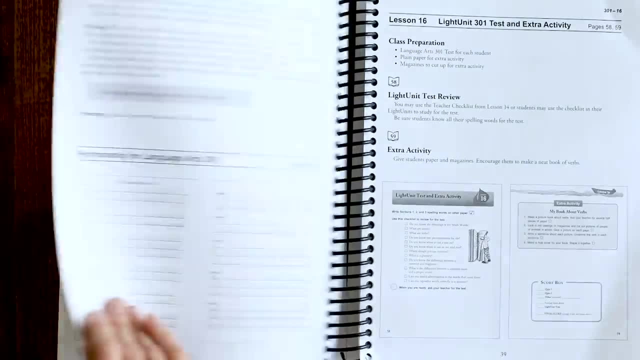 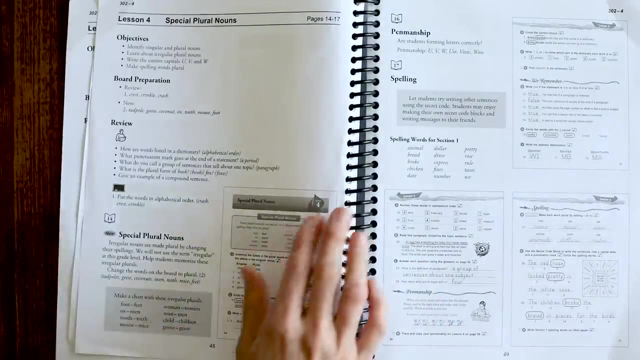 student page and so it explains it, and then they also you get to see what their answer should be and can market accordingly. so I like the way it's laid out. I think it's very, very easy to use and I think that it works really well for families that need need something that can be done more independently. so 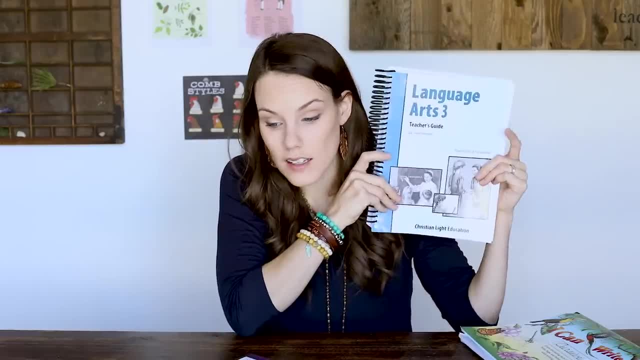 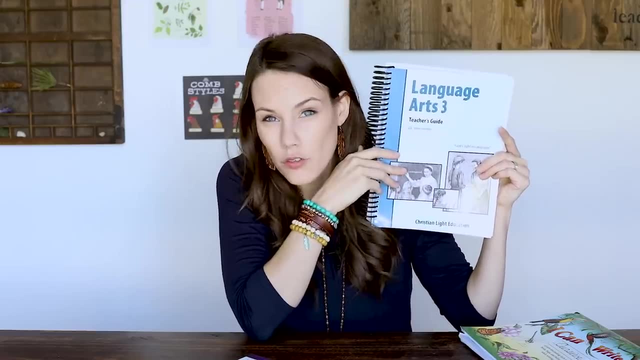 if you are looking for something that's Christian, if you're looking for something that is, you know, fairly affordable, if you're looking for something that can be done more independently, then this is going to be probably a good fit for you. it's not going to be a good fit for secular. 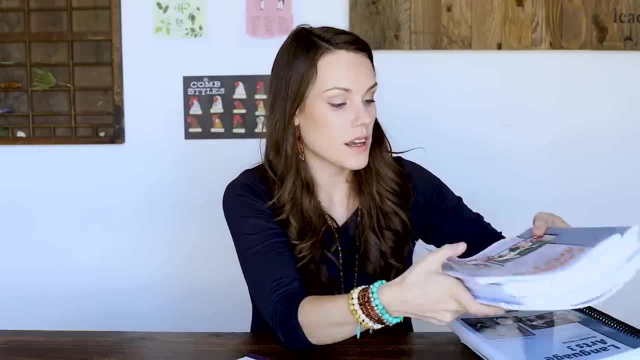 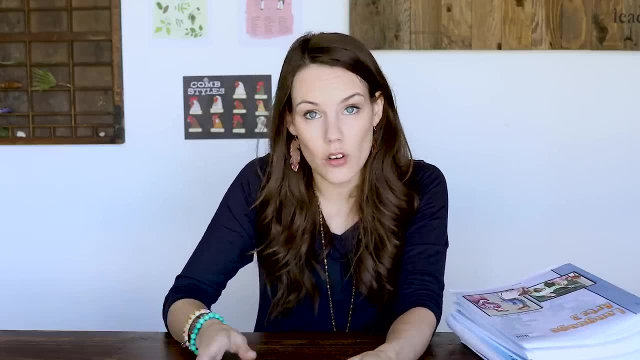 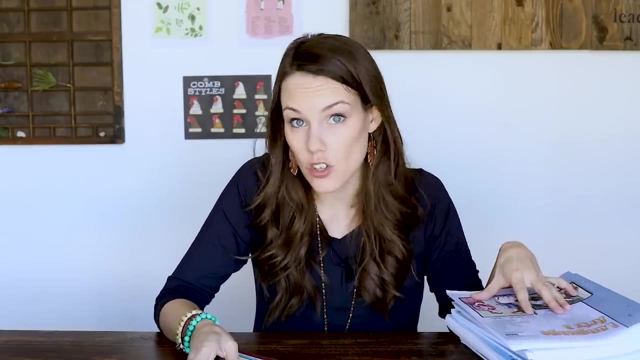 homeschoolers. it's not going to be a good fit if you are looking for something that is can either be blended or is more Charlotte Mason inspired or really any other homeschool style, because it's not. it also is not super kinesthetic, though I have to make note of the fact that my kinesthetic 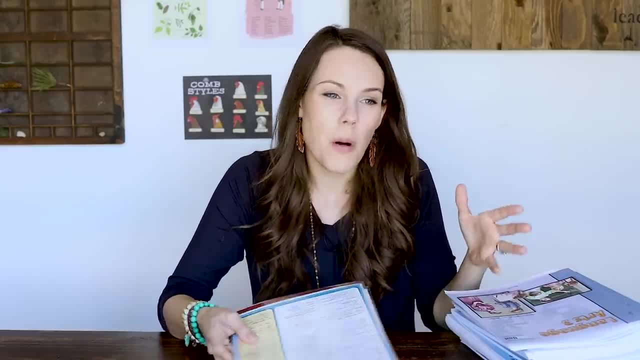 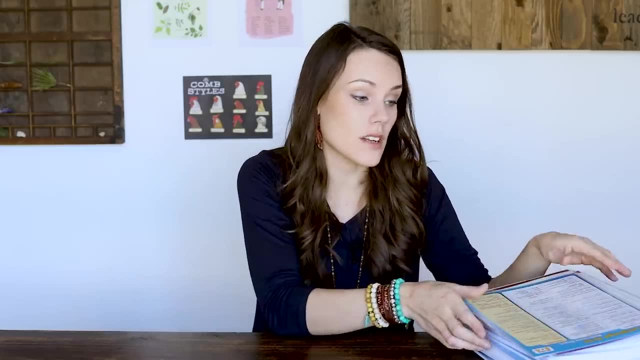 daughter is the one who's using this and thriving, so it's partly based on that. it also is partly based on the fact that she just loves doing stuff independently and building her confidence and not having to necessarily have me help her with every little thing. she likes to play, school and stuff like. 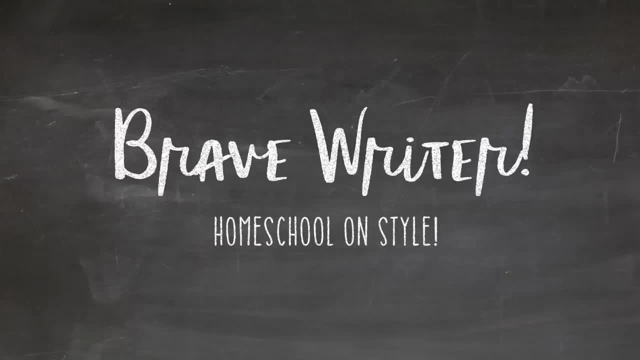 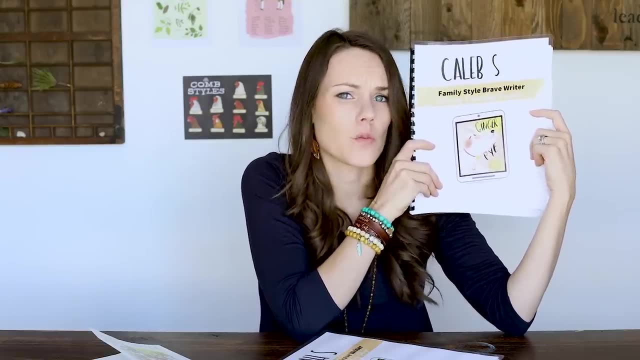 that. the next one I want to mention to you is brave writer. now, brave writer is something that could be done with the entire family. it is something that you can do with all your kids at home but doesn't make you feel extremelyata. name yourself. you found all these ear buds so far. I feel like we're in the 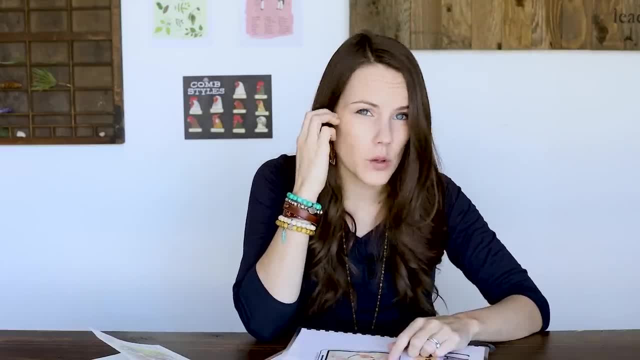 our Facebook fan club. that just sharing some stuff I would like for you. if it took some time before I actually was watching something that we talked about in my email chat, I would love to know your feedback on that after we get to by once, which is incredibly unique. There really isn't any other language arts program that does. 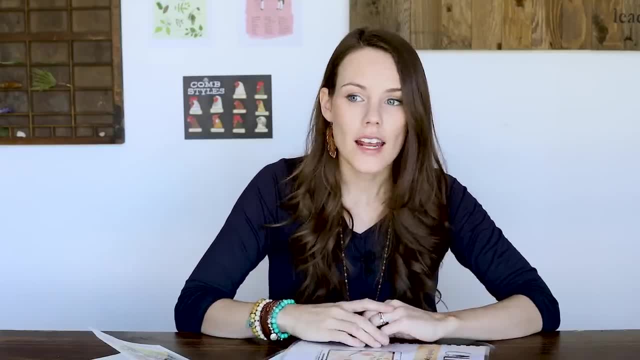 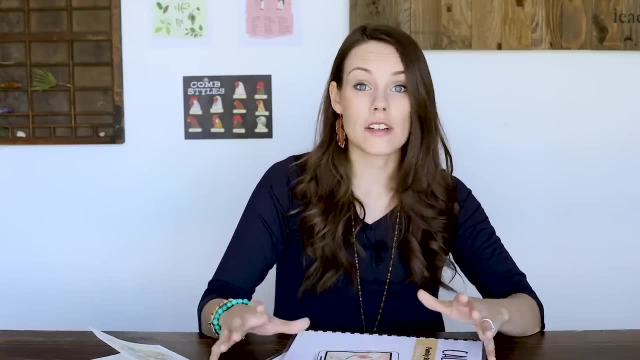 that, but it's more of a lifestyle. It's more Charlotte Mason inspired. It's just this beautiful expression of making language arts a part of your everyday life, rather than it having to be a separate curriculum or way that you approach it. So the way that it's laid out is this. I'm going 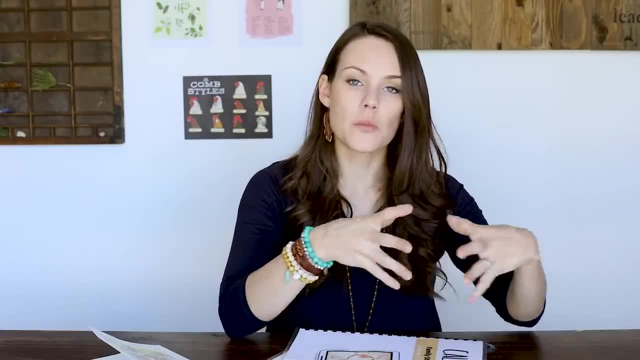 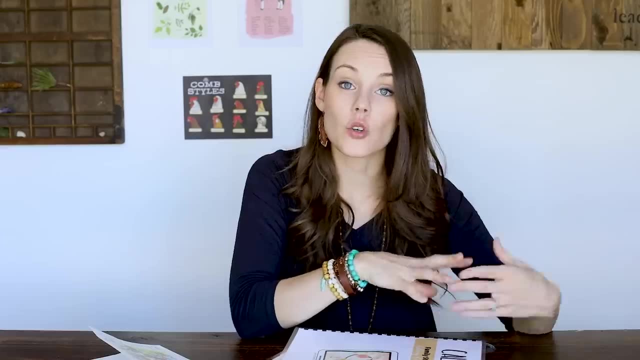 to lay it out for you very, very simply so you can have an idea. There is the Brave Writer lifestyle, which you're going to learn in the Writer's Jungle. The Writer's Jungle: it is a training manual for parents that teaches you how kids learn what their different writing stages are. 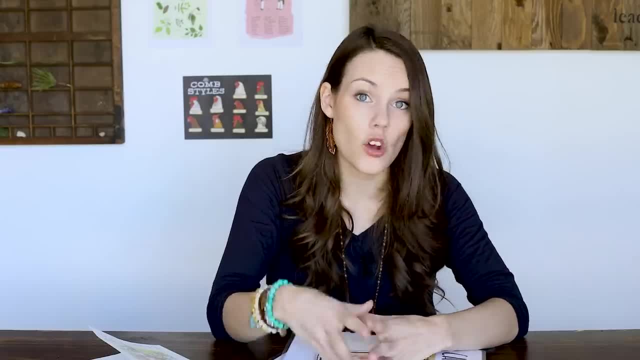 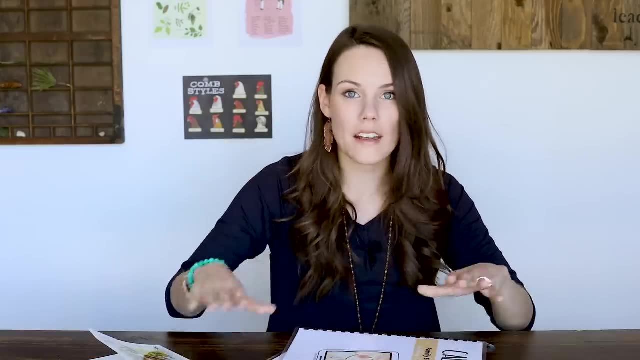 how to identify your child's writing stage, how to teach to that writing stage all the way through to high school, and how the Brave Writer lifestyle works. So how you can teach writing through anything, through any book that you read, how you can teach language arts through reading. 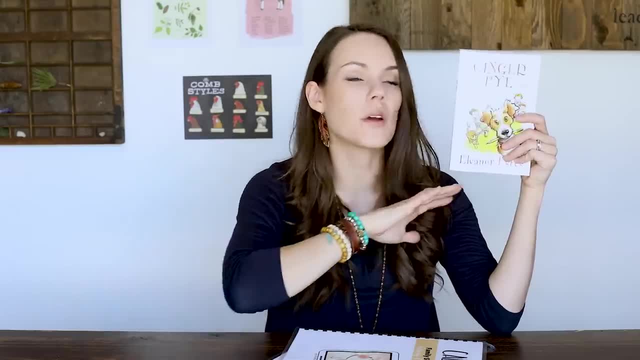 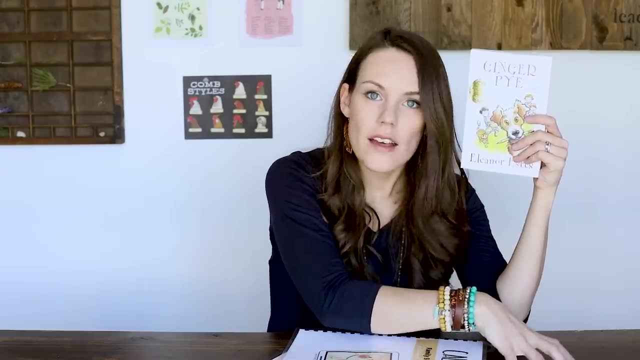 through movies, through poetry, through all of those. So it brings in how to teach language arts as a way of your life And so that training manual for parents is called the Writer's Jungle. Then you're going to see that there are writing, there's actually writing. 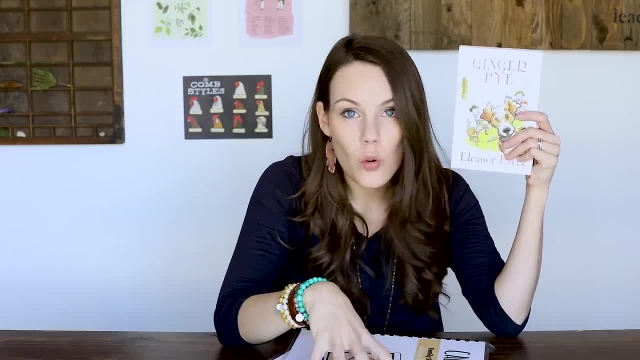 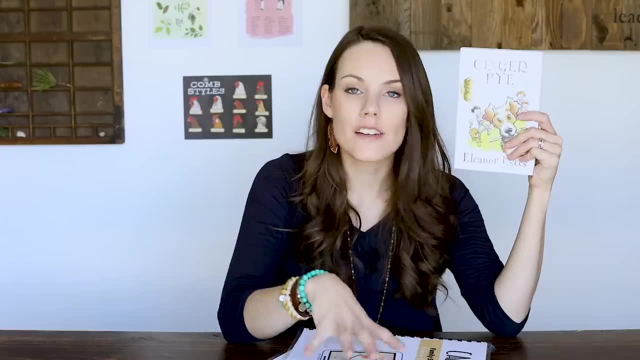 curriculum that's jotted down: partnership writing, faltering ownership, the great conversation, eavesdropping on the great conversation- Those are their writing projects. So that gives you 10 different writing projects that you can use throughout the year. So one writing project. 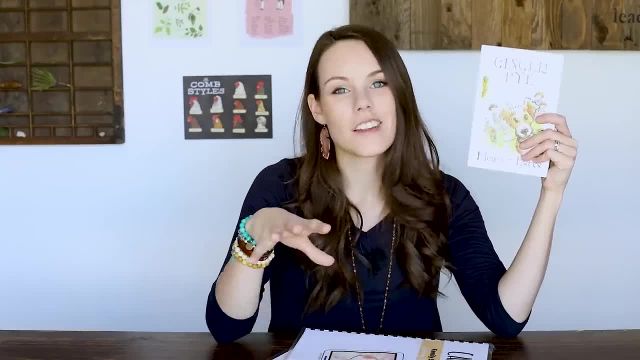 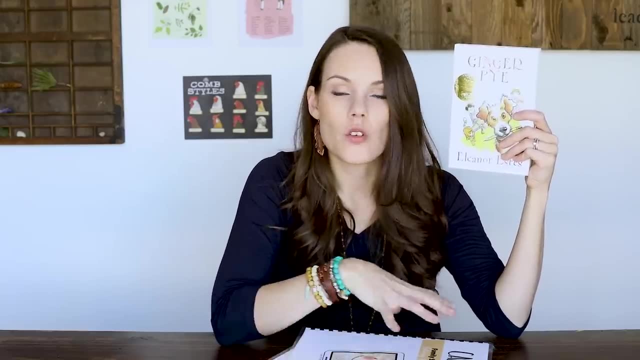 per month and it teaches you how to do that. Then you're going to see that there's the writing mechanics portion of it And that is things like the wand quiver of arrows, the arrow, So those titles that you're going to 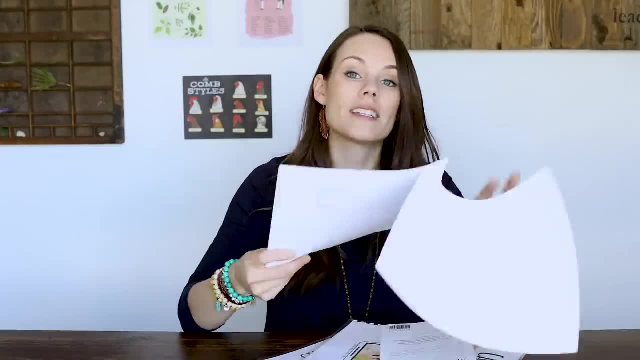 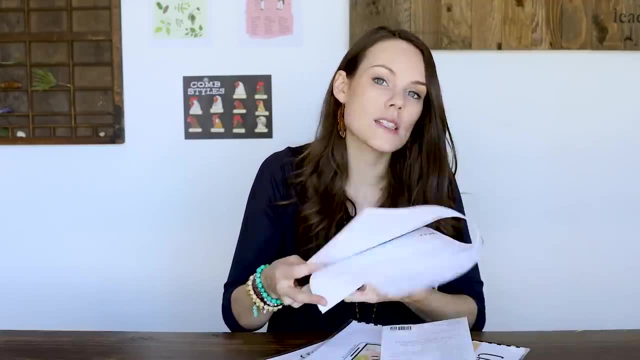 hear and be familiar with on the Brave Writer site. those are going to give you a book you're going to read with your kids, And then they're going to give you copywork passages and how to teach grammar and spelling through copywork. So it's going to show you a, a copywork passage. 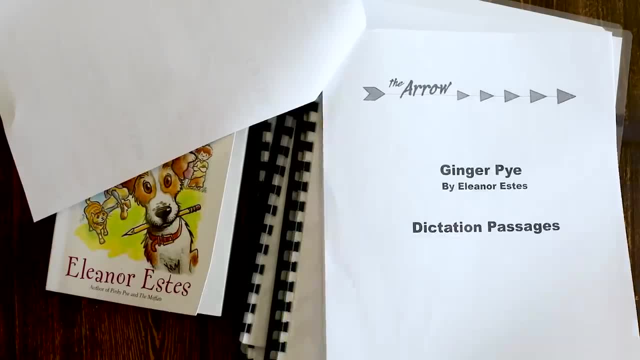 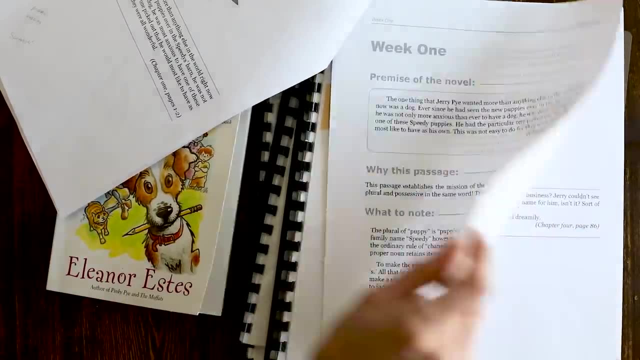 why this passage? things you're going to know. you're going to point out various grammar and spelling components And then the kids are going to be copying that through the book. So that's going to show you how to do it throughout the week And that is going to help them pay attention to. 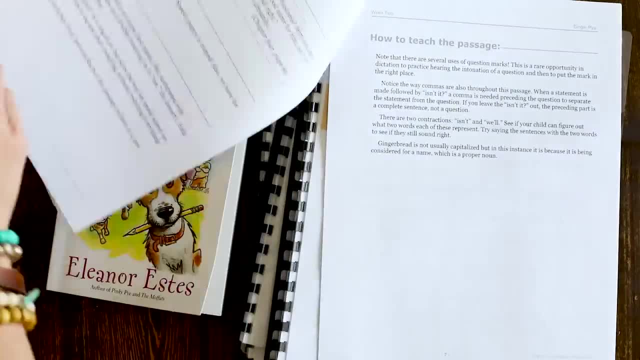 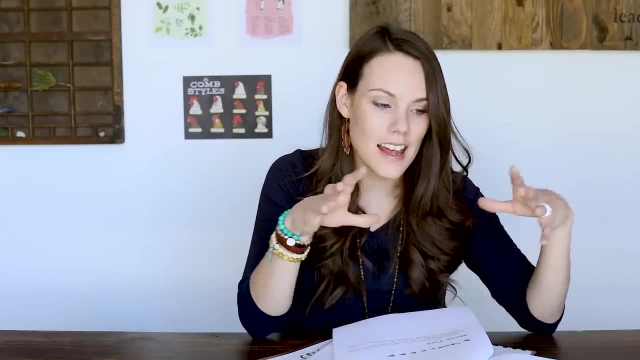 and focus on these different elements. So through their writing projects, they're also learning grammar and they're also learning spelling, because they are revising and editing their own writing. but they also get to revise and edit and pay attention to and examples from good quality. 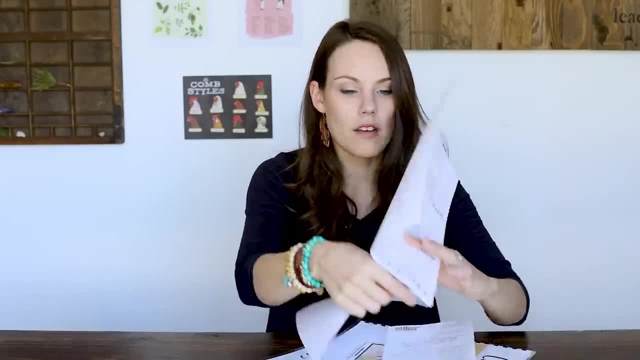 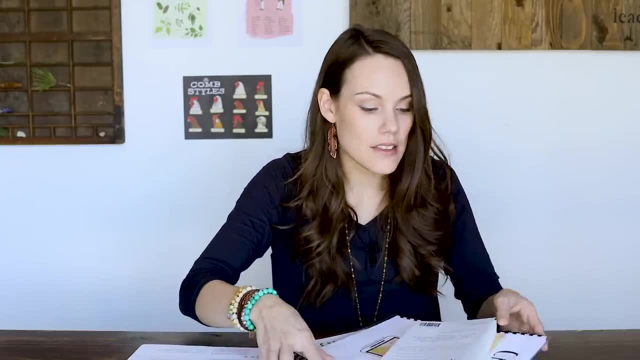 literature. So that is kind of the approach of Brave Writer Now for a lot of families. what what I love about it is that you can combine all of your kids. I've had some families say that they just don't know what to do, And I've had some families say that they just don't know what to do. 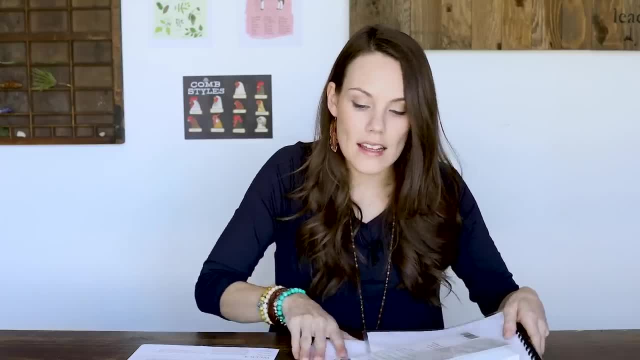 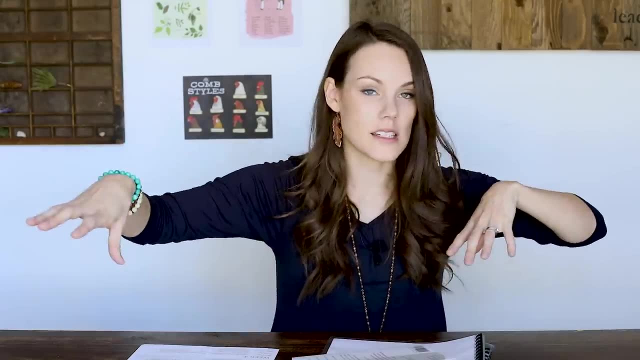 They don't know where to start or how to do that, because, though they they love that you can combine your kids, They they have some kids in this stage and some kids in this stage, and some kids need this arrow and some kids need the wand And, and so how can they read one book and teach? 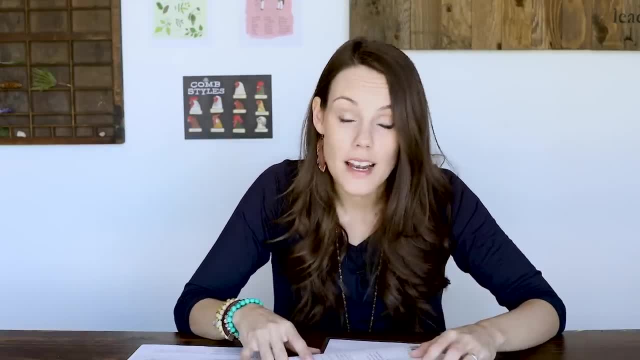 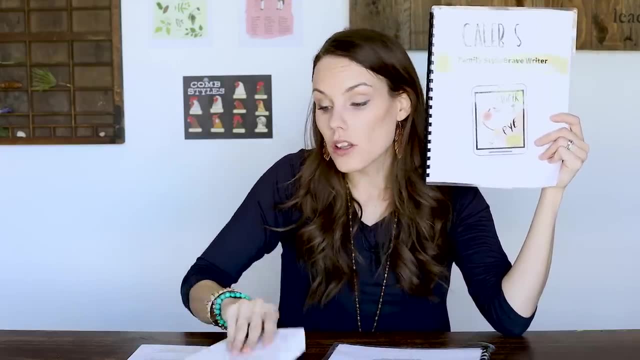 all of their kids language arts. So one of the exciting things that I am doing that I'm going to mention here is that I have put together a book club where I made a companion guide curriculum to go along with the arrow, as well as a schedule that's easy to follow So you could and it. 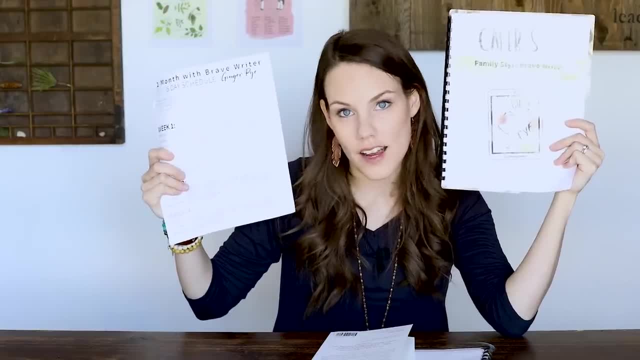 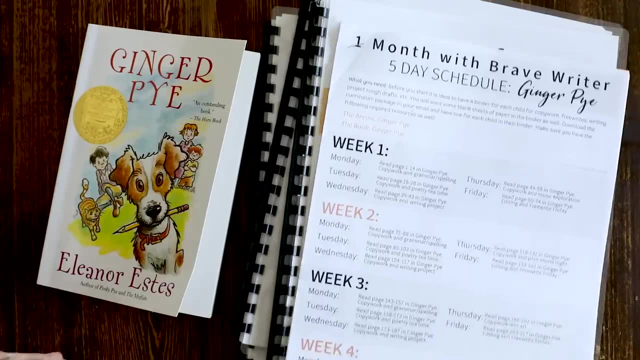 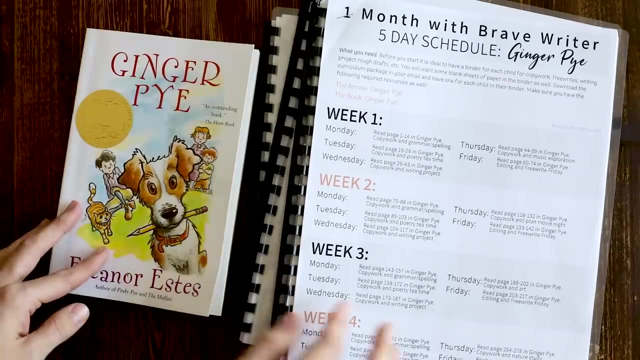 goes along with one another, So you would purchase the arrow off of the Brave Writer website. You're going to need to get the book that goes along with what we're doing. And then there's a schedule that says: this day, poetry, tea time. this day, free right. This day you're going to be. 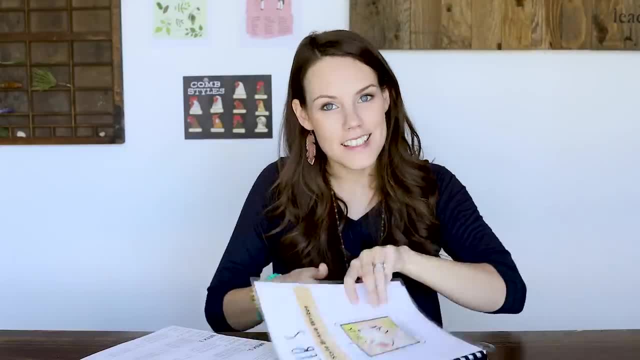 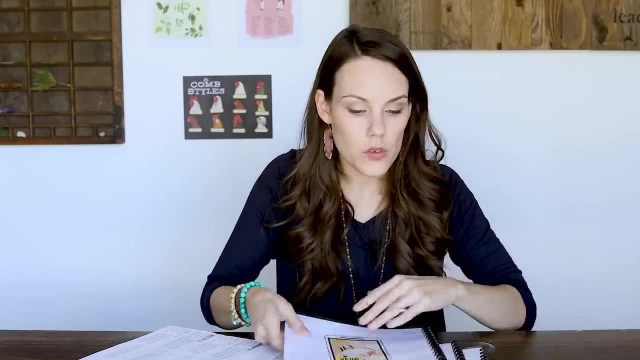 doing copywork or teaching your grammar, And then the kids books. there's three different levels available So you can download depending on the age of your child. So, for example, we'll start with the jot it down stage And then you can download the book that goes along with what we're. 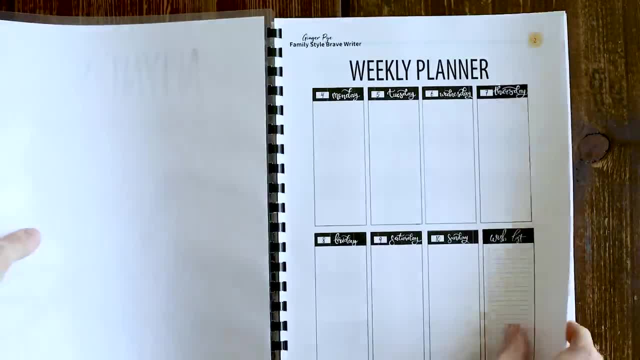 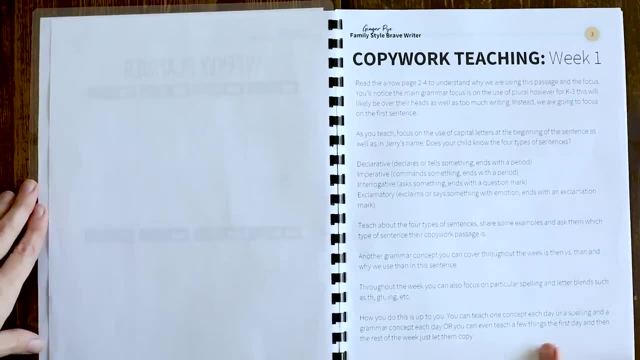 If we take a look inside, there's a weekly planner, there's how to teach copywork and there's adapted because in that, inside the arrow, some of that teaching, depending if you have a five-year old, that's going to be too advanced. So if you have a five-year old, let's focus on capital. 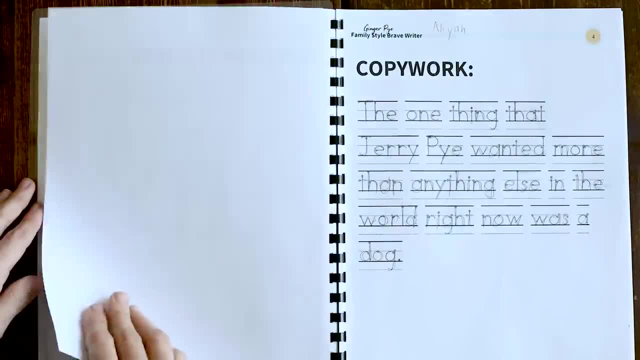 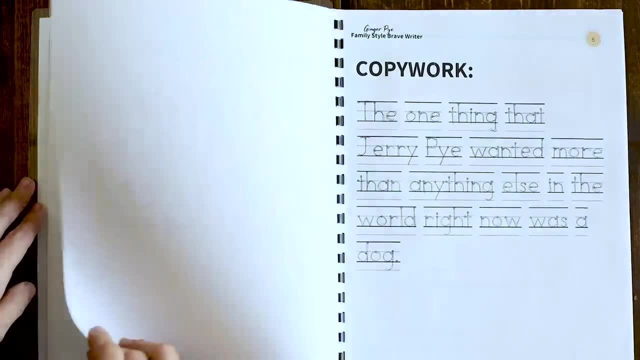 letters, And so it has those adaptations. It also has really traceable copywork passages which are easier for kids in the jot it down stage, So it's not so overwhelming. It has their writing projects and it gives them a bunch of different things they can choose from. So they can use it to do their writing projects. So if you're a 5-year old and you're a 5-year old, you can use it to do your writing projects. So if you have a 5-year old, you can use it to do your. 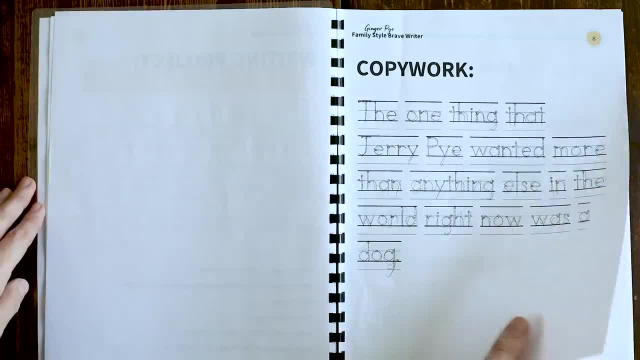 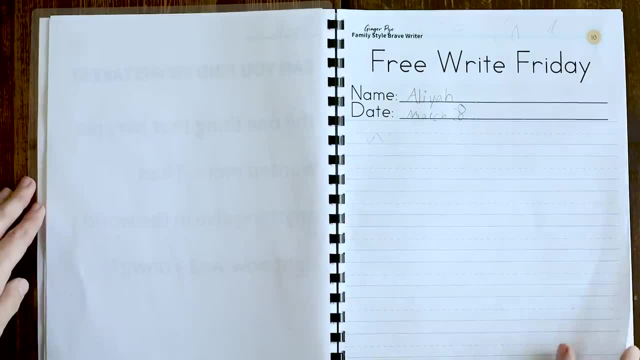 get to make it their own, and then at the end of their week they are going to be editing a passage rather than having to do any sort of dictation for that age. and then they also do free writes, and then it goes on to another week now. 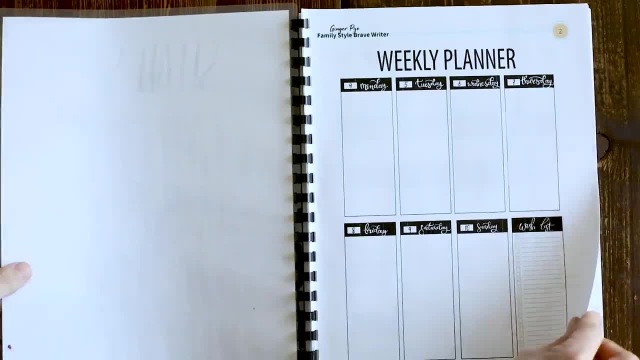 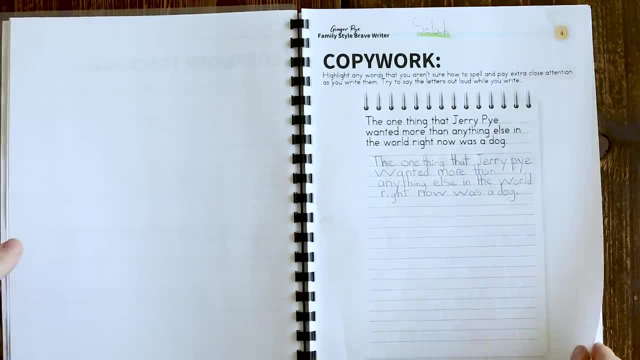 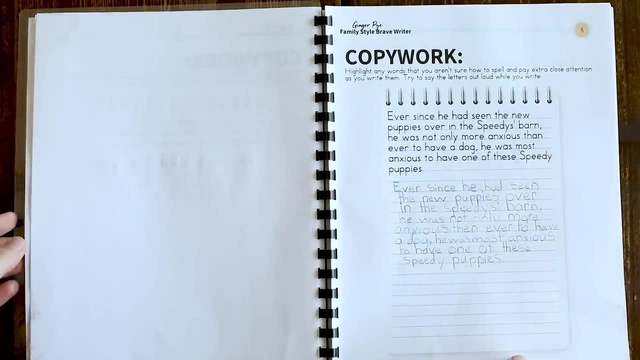 inside of the partnership writing curriculum bundle. it's the. the copywork teaching is a little bit different. you're going to be using a lot more of the arrow and the copywork passages are different. there's- and obviously they're not doing tracing at this stage so you can see how that is laid out and there. 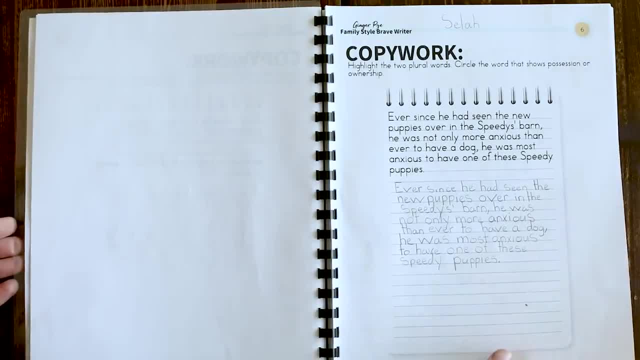 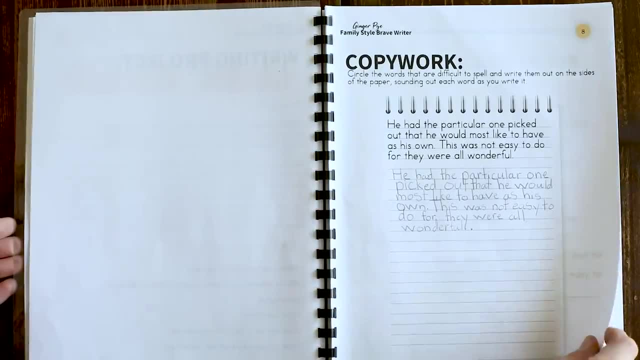 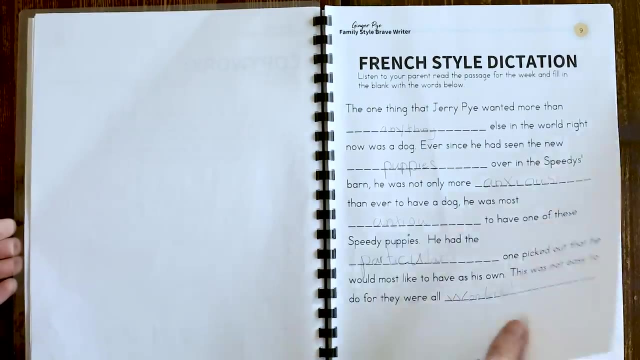 are some. you know different teachings as well. the writing projects are very similar, that they get to choose from, and then they do French style dictation instead of doing just the editing. so that is the way it is laid out for the partnership writing stage, so you would download whichever one you needed then. 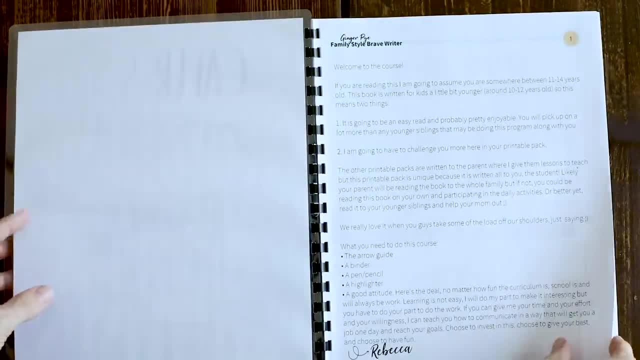 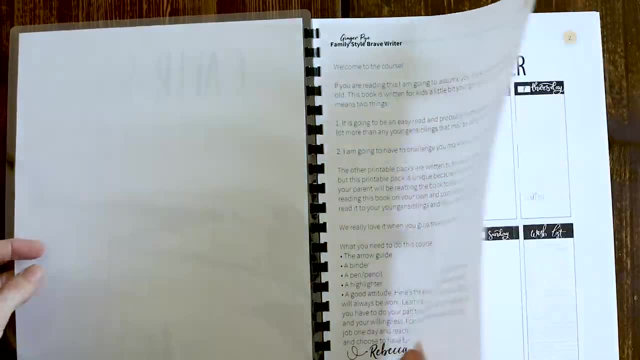 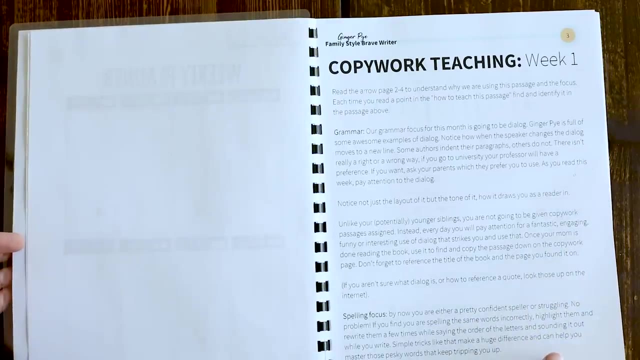 there is the faltering ownership stage. now this is written actually directly to the chapter a child. so at this point it's going to be different. they are going to be using it themselves, they get to read through and they actually are finding their own copy work passages based on what they're learning, which, for this particular 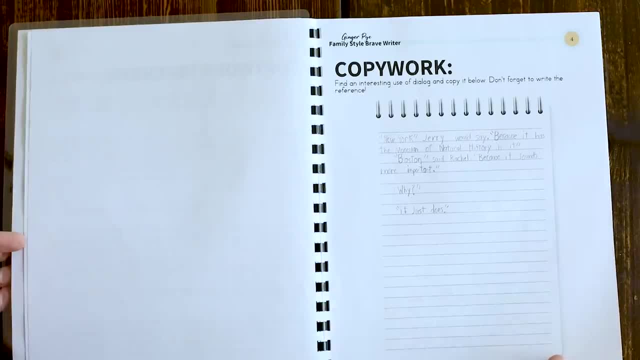 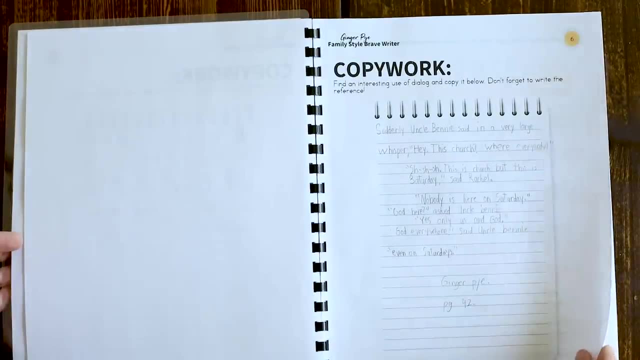 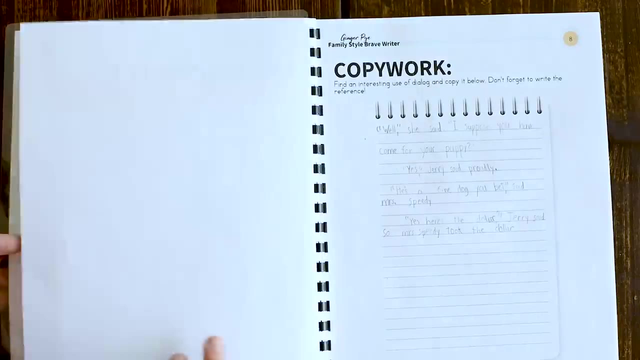 ginger pie. one that we did was they were learning about dialogue and how to write dialogue, and then they have some different kind of stories that they're working on and that's all built in to this one. so it's different for each level depending. So I've put together kind of this companion guide that shows you how the brave writer lifestyle works. 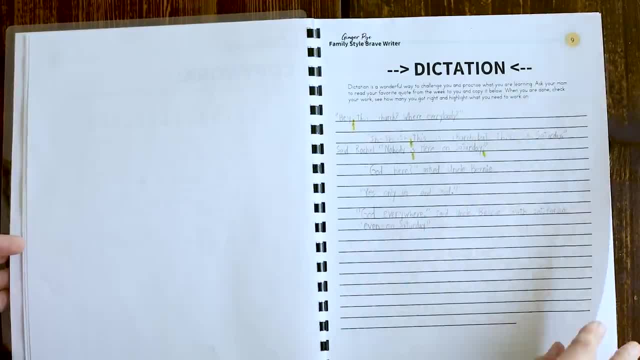 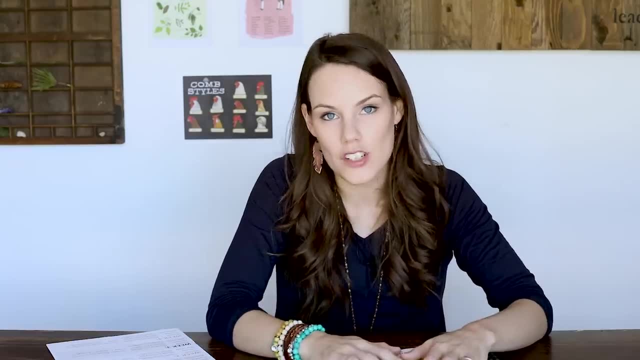 And it's a ton of fun because you get to do it as a family. It's also a ton of fun because you get to do it with other families. So you get emails, you get weekly videos and at the end, all the kids get to share the writing projects. 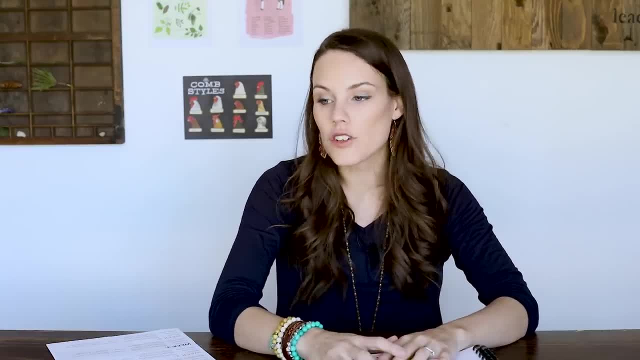 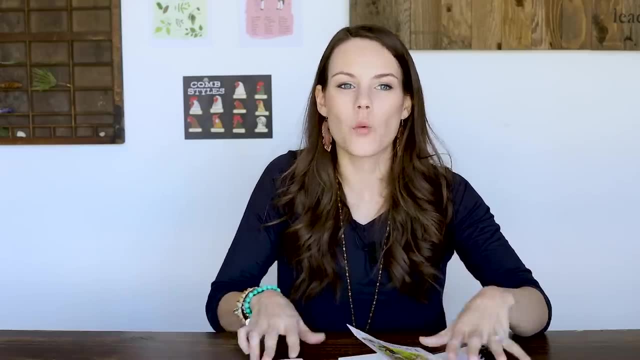 They've done, so you get this kind of community atmosphere. so if you're looking for something that is like really, really, really fun and Has that accountability and will lay it all out for you in a way that is really out of the box from most other language, 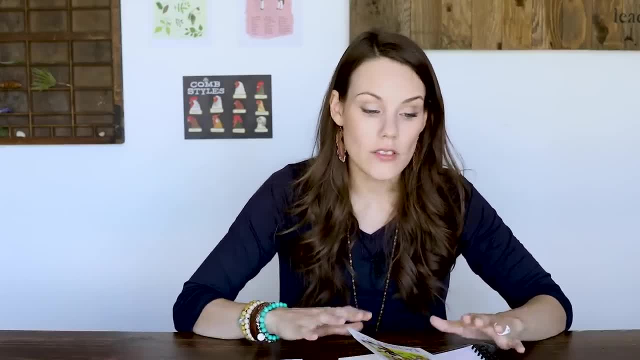 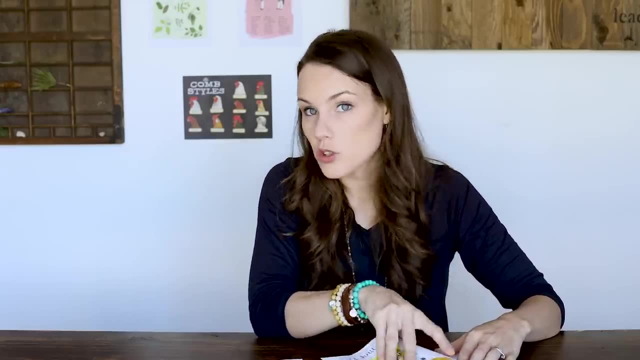 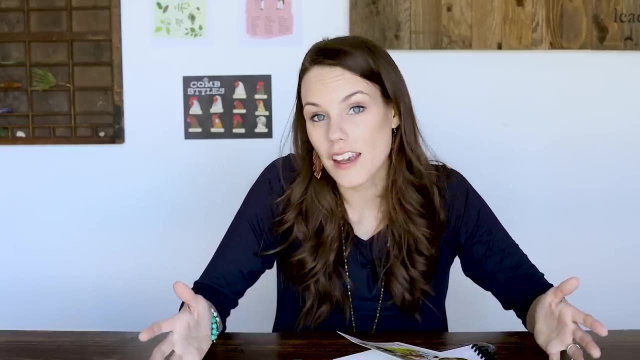 Arts curriculum, then that may be one to consider. It's relatively affordable to just join in for a month. It's $24.95 for the live month, and then you need to grab the book which you can get at the library, and the arrow, Which is usually around $10. So that's something to think about when you get to do it with all of your kids. 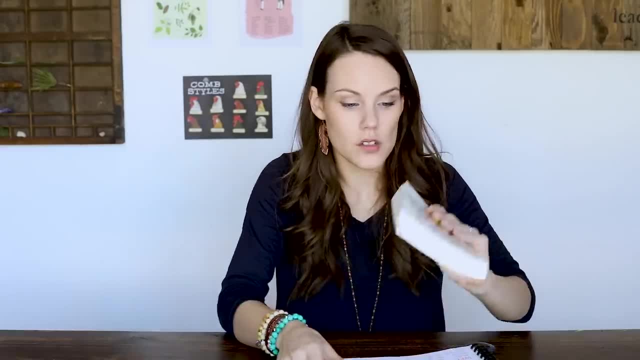 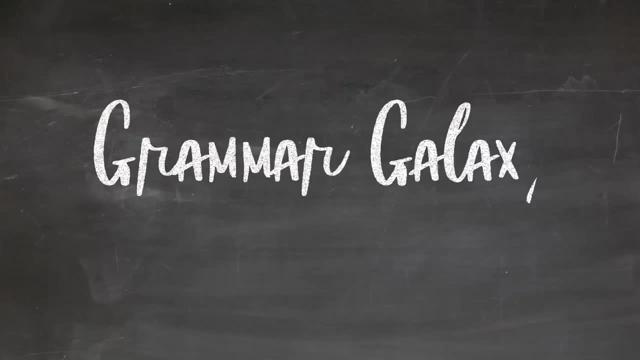 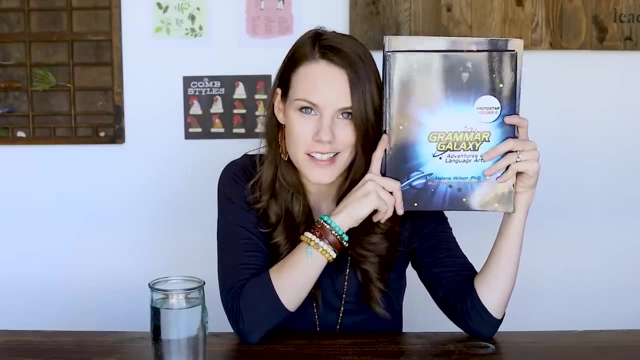 Then it makes it a very affordable language arts option. So you can check that out. all the links for this are going to be below, so you can check in the description below. All right, the next one I want to show you is grammar galaxy. Now, grammar galaxy is a little bit unique because they have this mission. 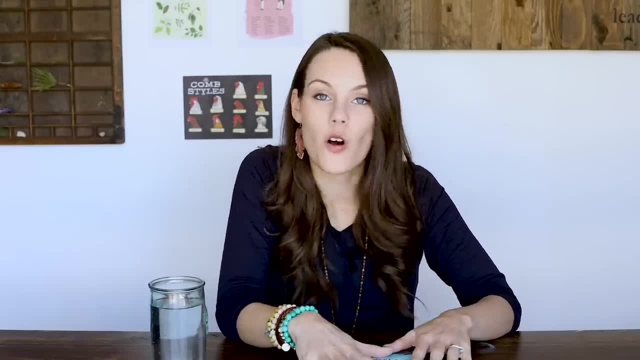 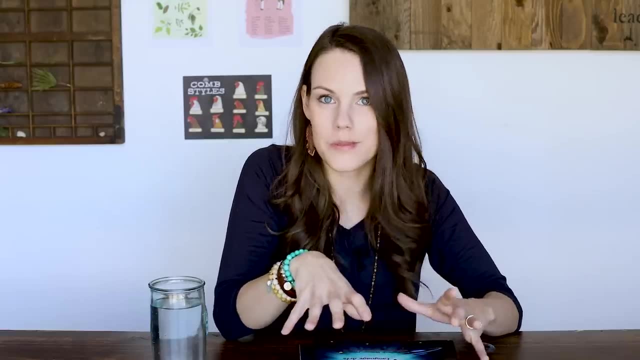 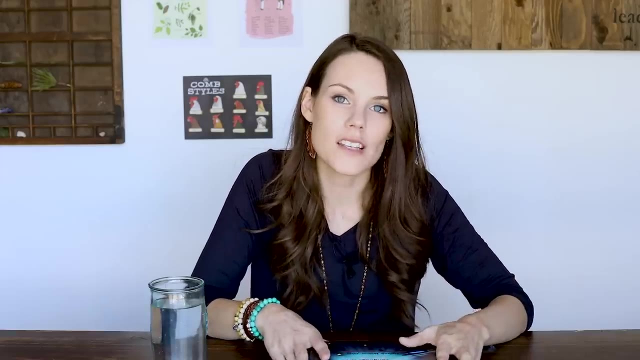 Manual where they are going to be reading stories following these three kids, these three children who are trying to save the galaxy and giving them different missions to help them save the galaxy, things like saving spelling planet and Different things like that. So it incorporates all their language arts. 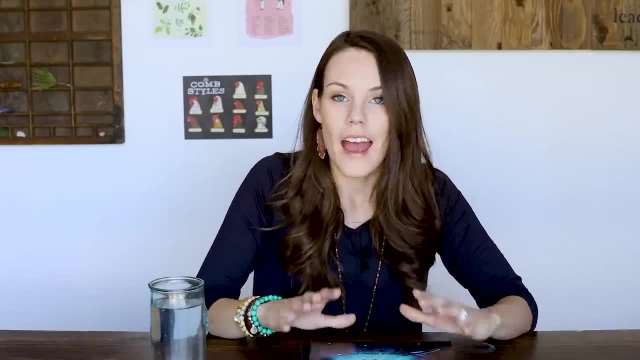 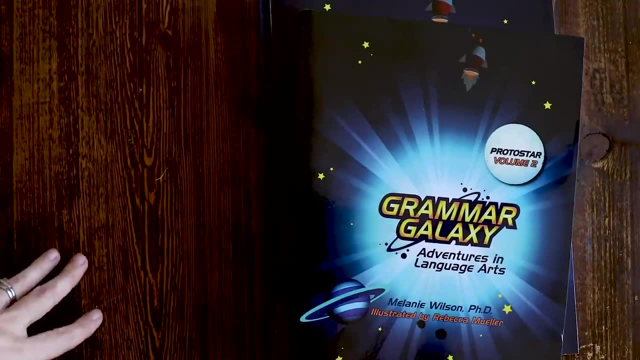 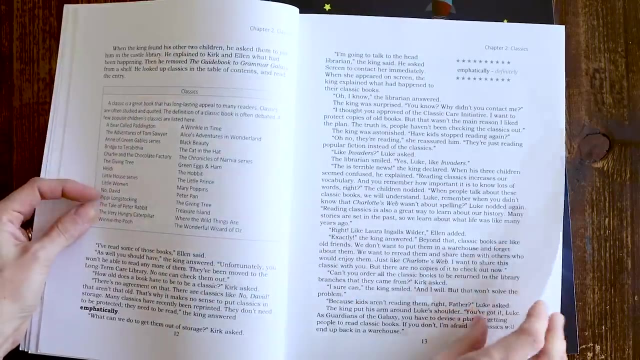 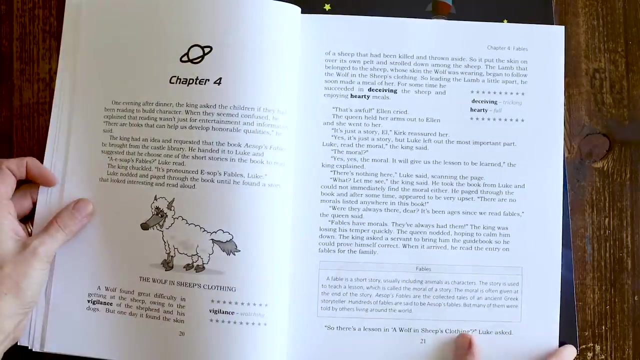 but in this really fun, adventurous way and through stories, which is kind of unique. so inside the actual mission manual it is, it is laid out in a way that is not too overwhelming. so this is protostar. this is volume two. so if we take a look at the table of 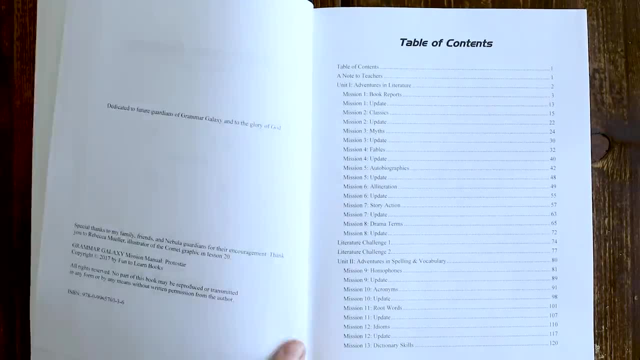 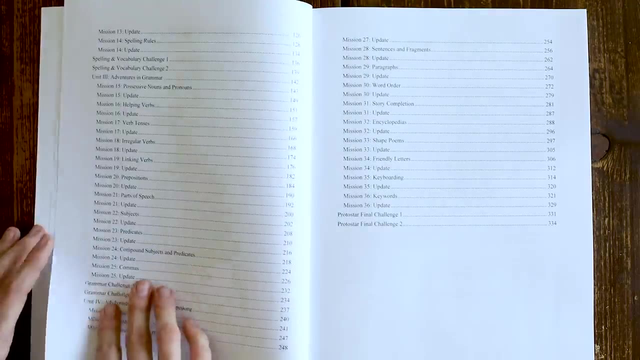 contents, you can see some of the different things that they are going to be learning about throughout the year, so you can see how it includes some composition towards the end. it's including grammar, it's including spelling and all of those things. so lots of people use this as their soul. 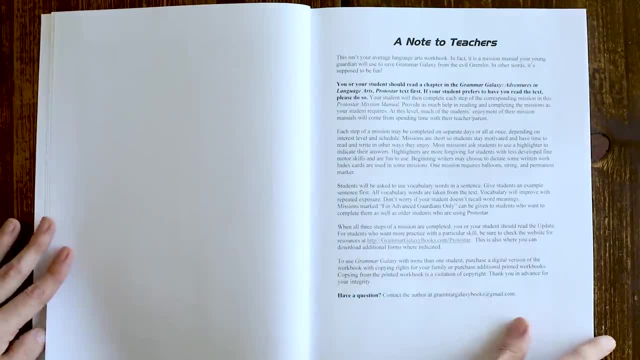 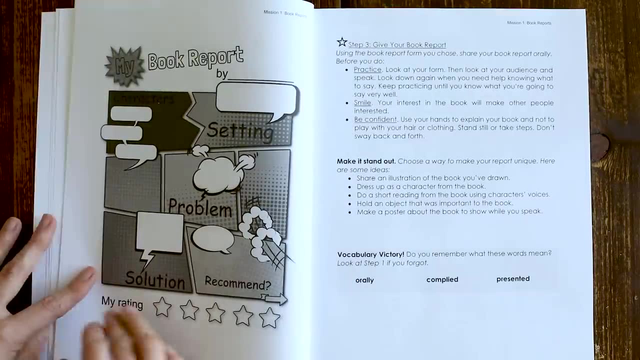 language arts curriculum. some people use this as a supplement. it's going to depend on your family, as how you want to use this and what and how much language arts you want to do. so, at the beginning, they get their mission. they read their story and they receive a mission, and then 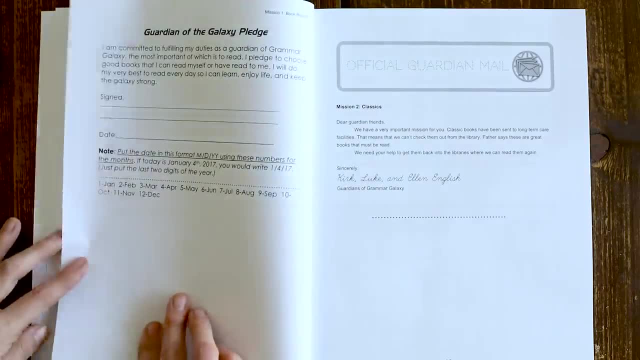 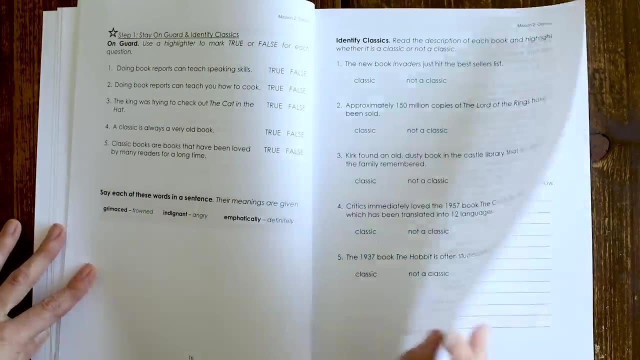 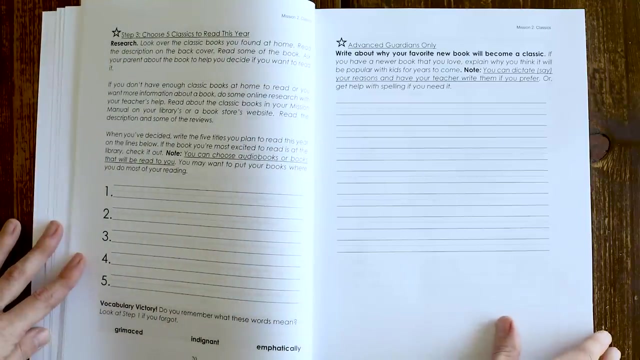 they work on a step a day. So this shows you, they includes. you can see there's vocabulary words. they're circling, so it's not as much writing. there's lots of circle, the right answer, um, and, and gives them really basic. okay, we're going to work on a book report, so here's how we're going. 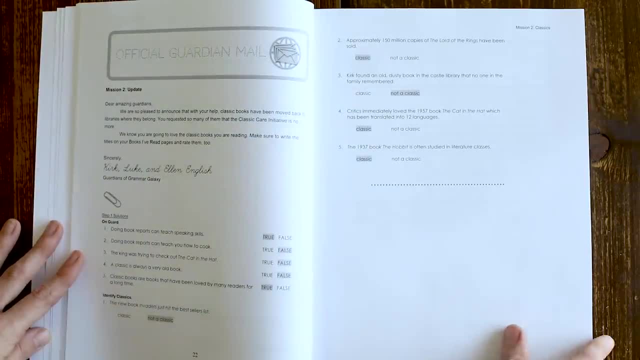 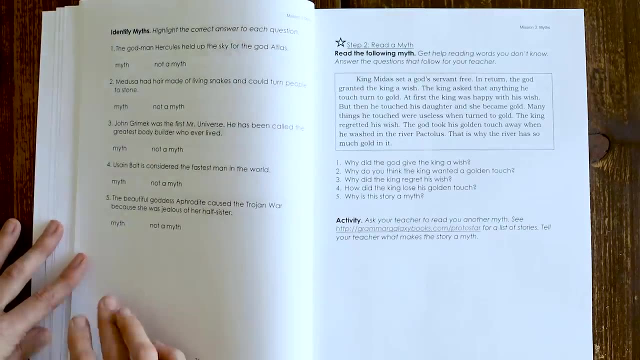 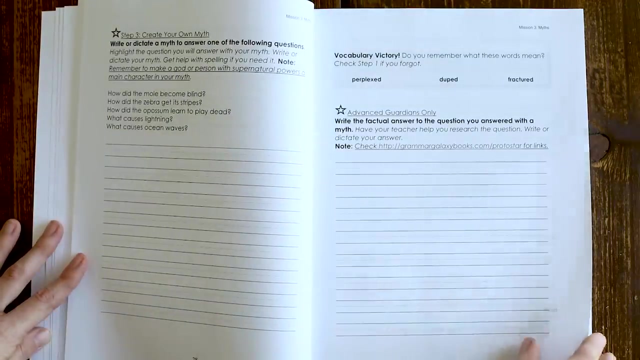 to do it and so it's not too overwhelming for them. This works really well for kids that are struggling or reluctant writers. It works really well for kids that are disinterested in school and can be a way of making language arts more fun and out of the box and even a bit surprising. 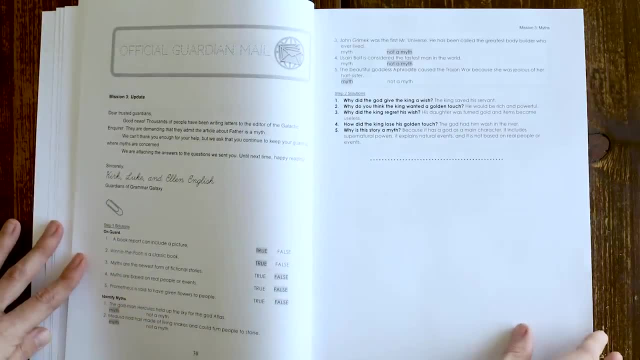 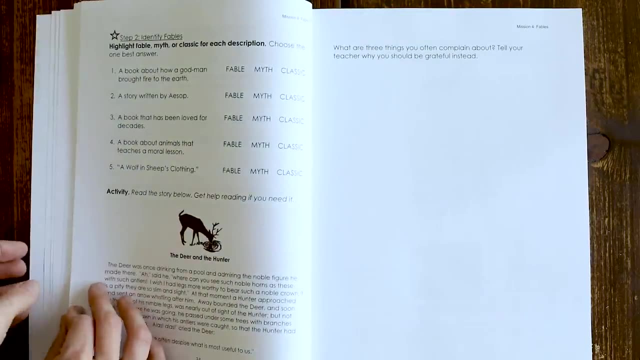 So if you're looking for something like that, check it out. it is still teacher led, but the lessons are short, so it isn't something that's going to take up a ton of time and you're going to need one per child, so that is also something to keep in mind, even if you do choose to blend. 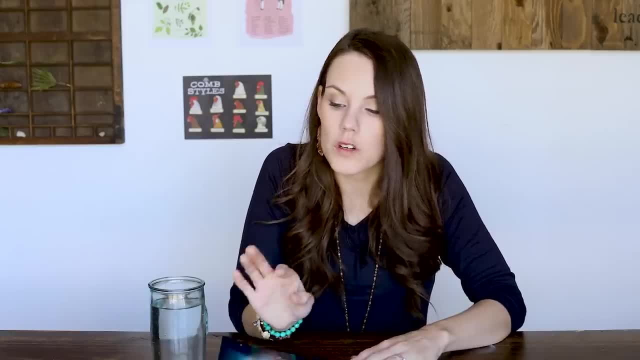 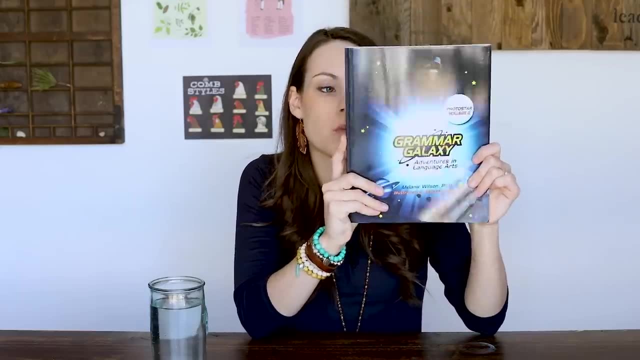 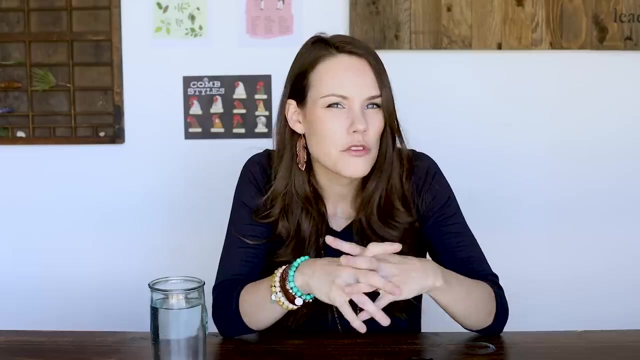 your kids together. Each child is going to need their own mission manual and then you can have one of your stories that you would be doing as well. So that is Grammar Galaxy. you can go and check it out. it's definitely has a bit of a Charlotte Mason flair with the stories it also has- um, it has a little. 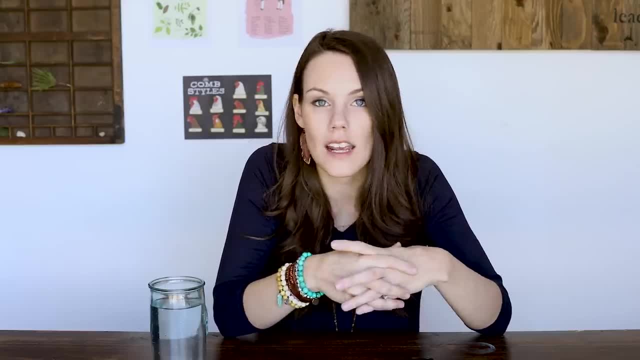 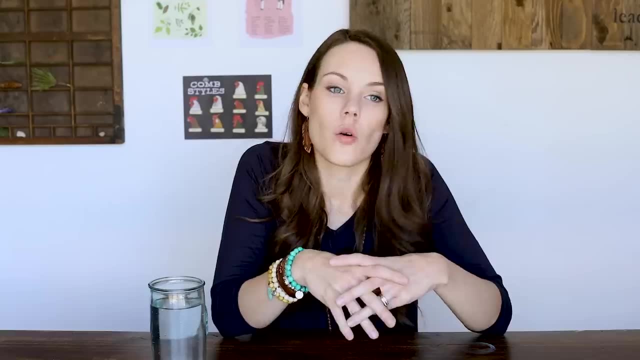 bit of a traditional flair with, with the way it's laid out and it's very open and go, so that works well for a lot of families as well. It is relative, It's relatively affordable and so it's not one of those you know crazy, crazy, crazy expensive ones. 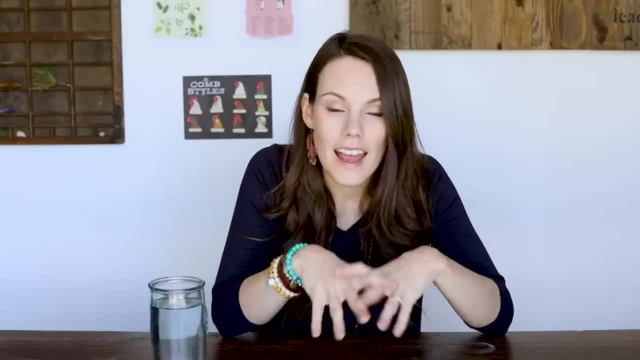 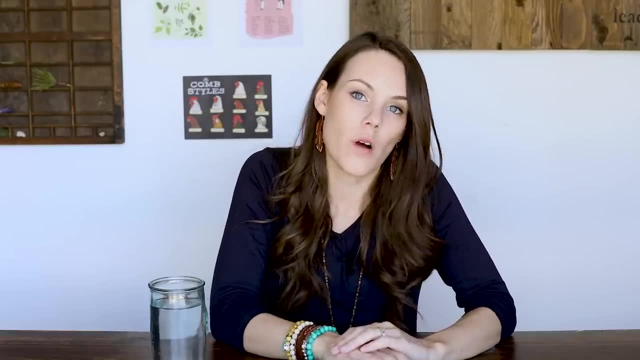 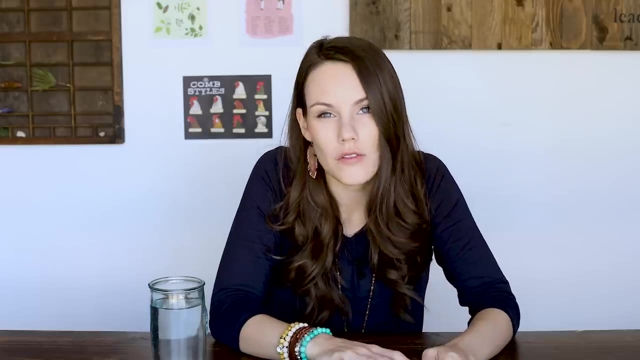 that is super hands-on and it can get your kids involved, no matter what their learning style. it can gear and be targeted towards any learning style, so that works well as well. The other thing to keep in mind is this is secular, it is neutral, it doesn't have God in it. so if you're looking for 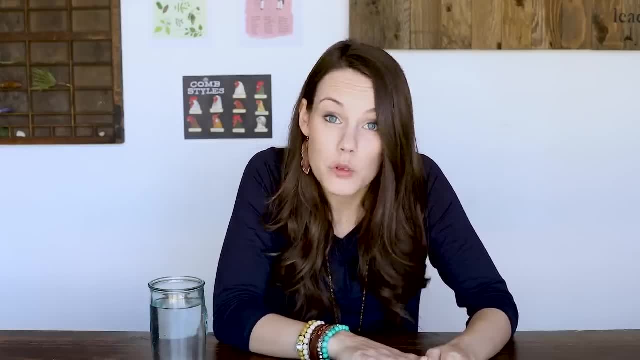 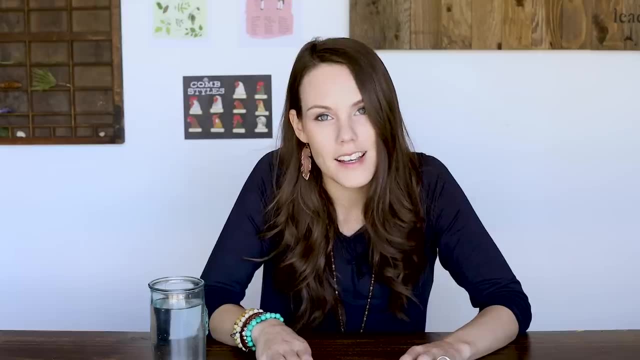 a secular curriculum option for language arts, then I wanted to make sure to include this so you guys could see that there are options out there that are not Christian based, because we don't have a lot of Christian books. we've shown you a lot of Christian ones so far, so Grammar Galaxy is secular and it is a 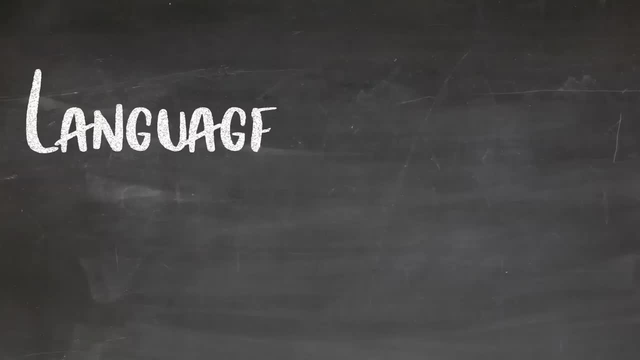 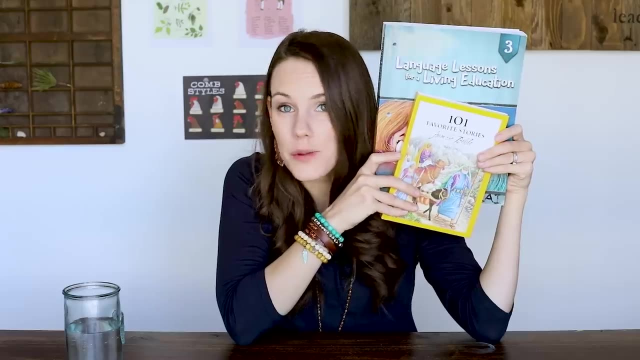 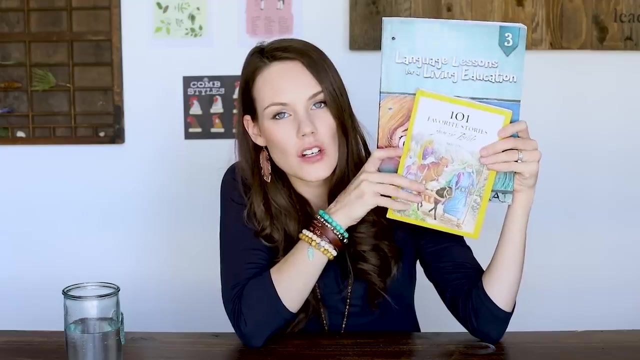 a fantastic program to check out for your language arts. 唾 🎵, 🎵, 🎵. Alright, the next one I'm going to show you is Language lessons for Living Education from Masterbooks. now, language lessons for living education is also super open and go, but it also incorporates some. 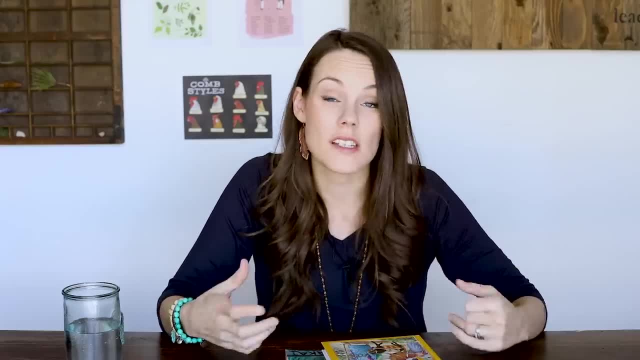 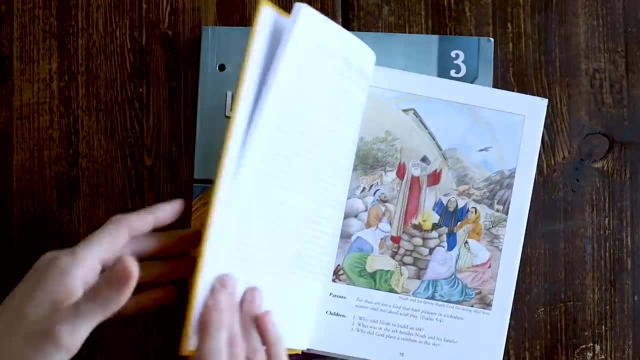 Charlotte Mason things like poetry and picture stuff. So they go intoologiuos. they are really nice- picture study and all of those different things as well, So it works well in that capacity. It comes with a Bible story reader that they're going to be reading about a page a week And then what's. 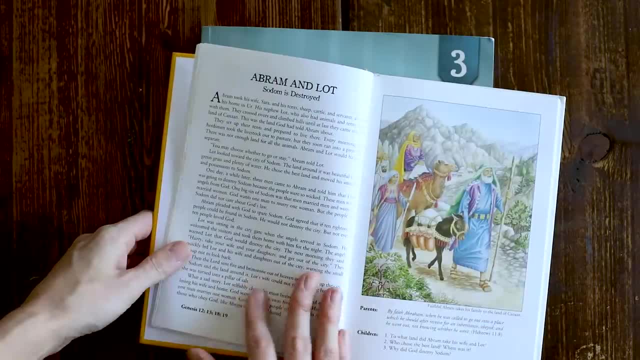 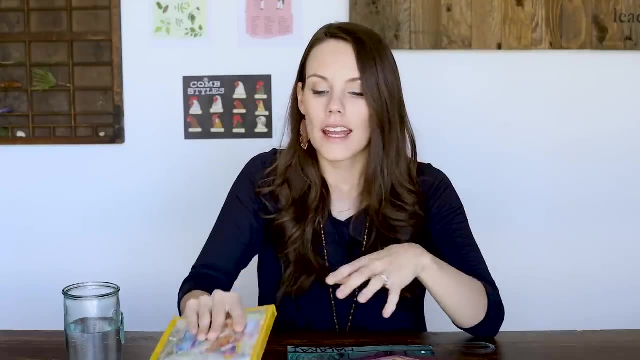 really unique is it's got beautiful paintings. They're going to copy that and they get to draw it in a space, They get to do copy work from within this book and they get to answer some questions. So it brings in that narration and that copy work and some of those different, Charlotte. 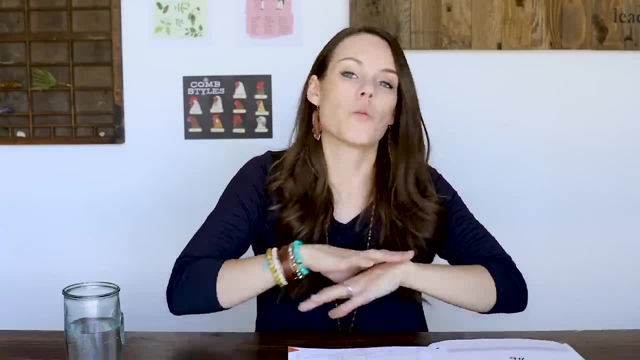 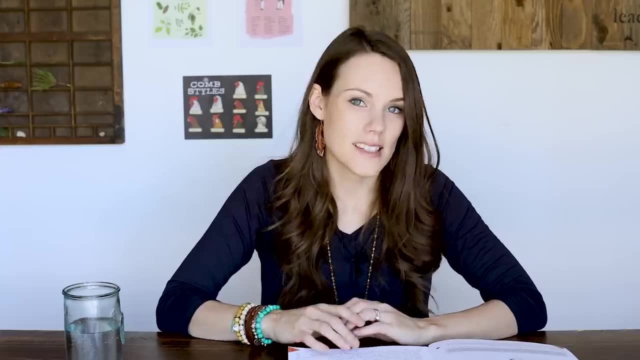 Mason things in there. What is really unique about it, though, is that, while it has the Charlotte Mason flair- and it's really just beautiful in its approach- it is also short lessons that are not too overwhelming. It's it's very, in that way, also Charlotte Mason, because Charlotte Mason 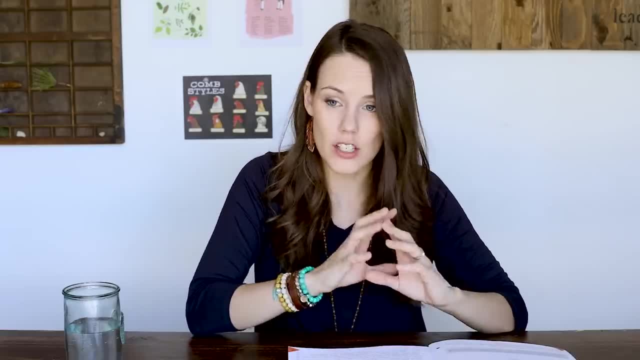 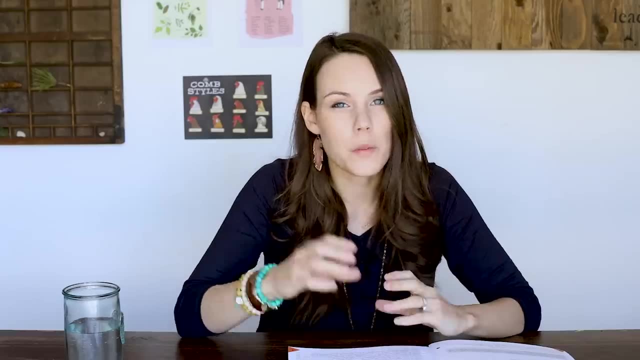 one of the principles was that you would do less and you would expect more from that less. So, rather than bogging our kids down with hours and hours and hours of work, let's give them less work, but let's expect greatness from them. So this really fills that Charlotte Mason philosophy of. 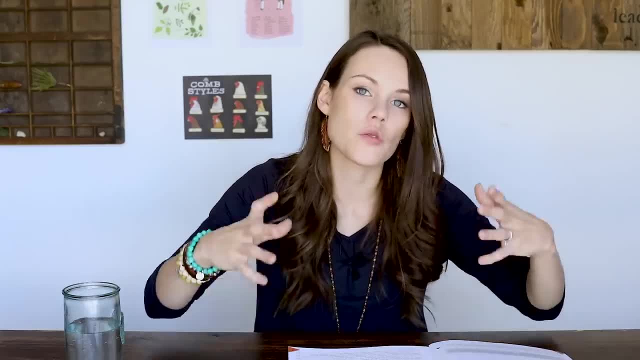 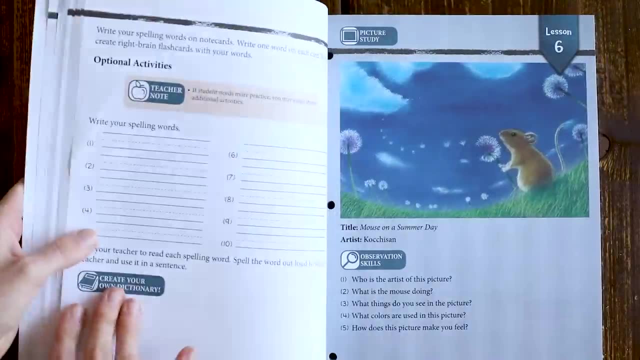 lessening the workload, but then our kids are actually able to absorb that information. So let's take a look at the scope and sequence so you can see some of the different things that are included in this. So there's 36 weekly lessons. It is laid out with 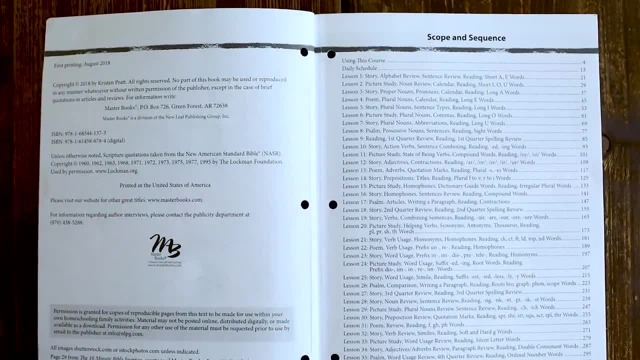 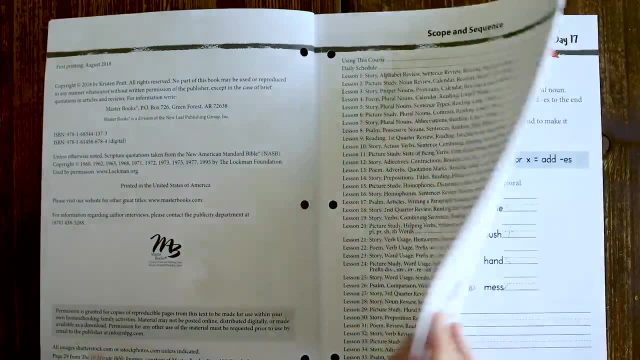 five days a week, So they're just going to do a couple pages a day, and there is no teacher's guide for this, So all of the teaching is built right into it. There's little kind of notes for the teacher, if there needs to be. So let's take a look at some samples. We're going to 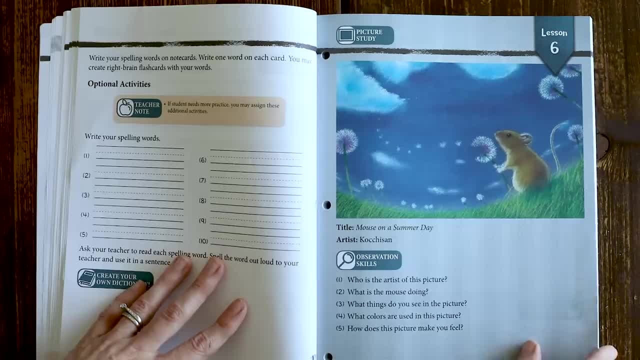 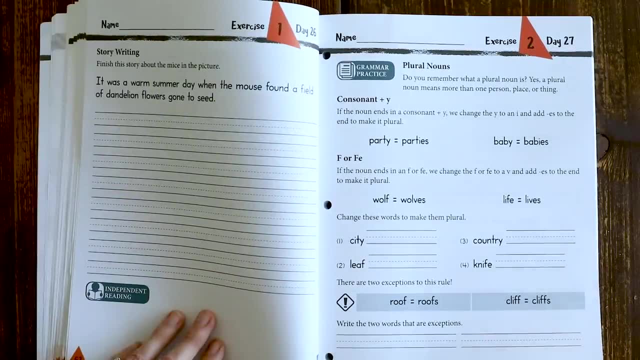 start with the first one And see. so there's, it starts off with some reading. So, again, it's very story based. It's also very biblical and very, very Christian built into everything that they do. So you're going to read, and the highlighted portions are ones that the children are going to. 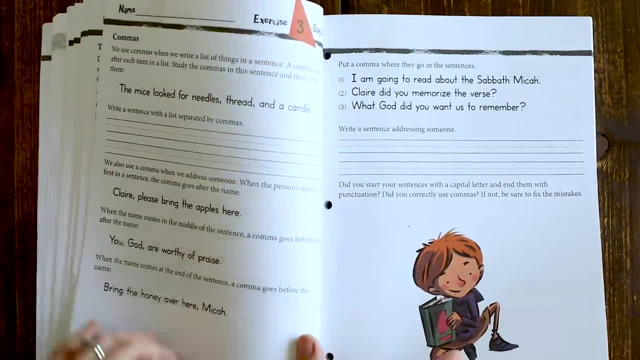 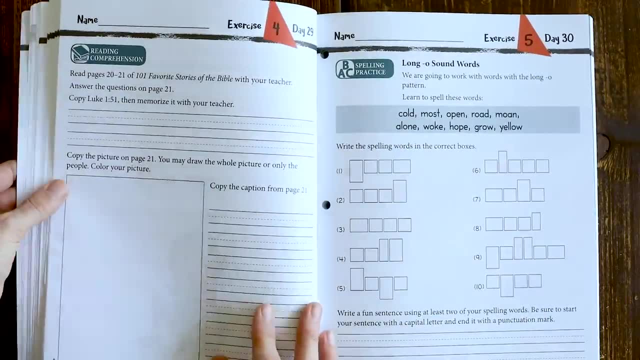 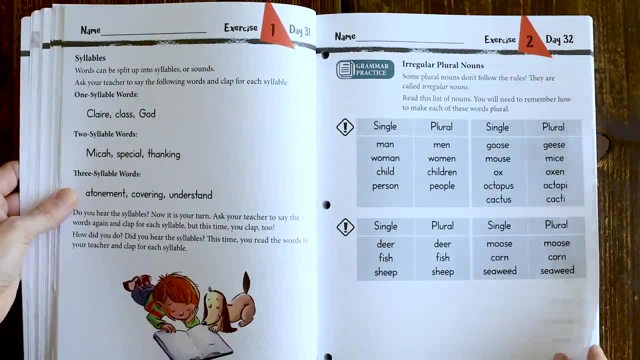 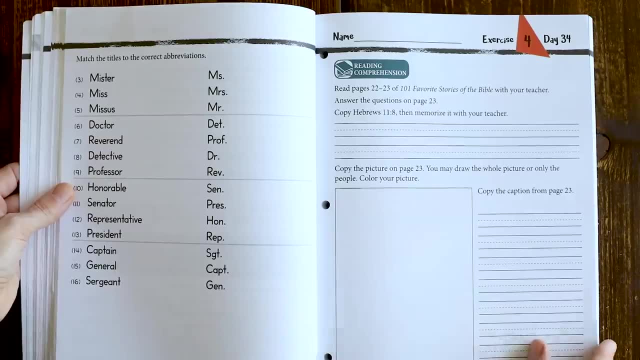 week For this week, here and then reading. comprehension is where they're going to use their stories from the Bible and they're going to read, they're going to copy, and they're going to copy the picture and color it. There's spelling practice built in as well, And then you're on to 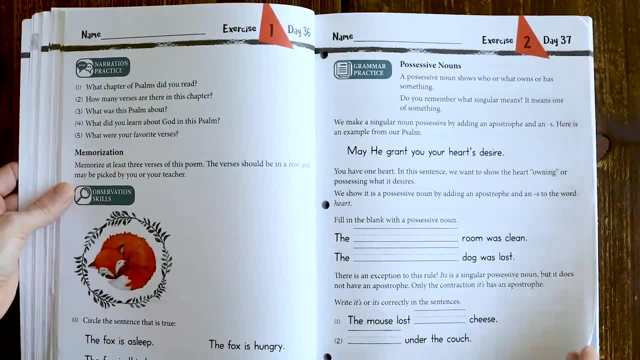 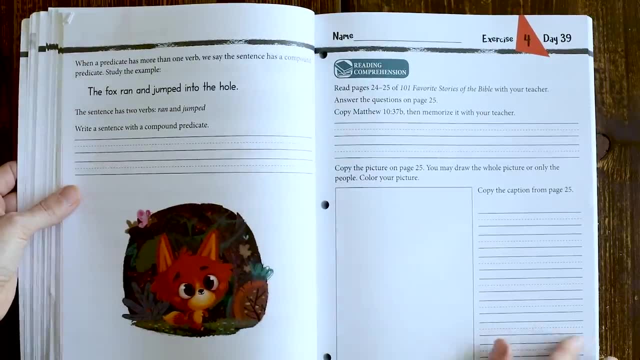 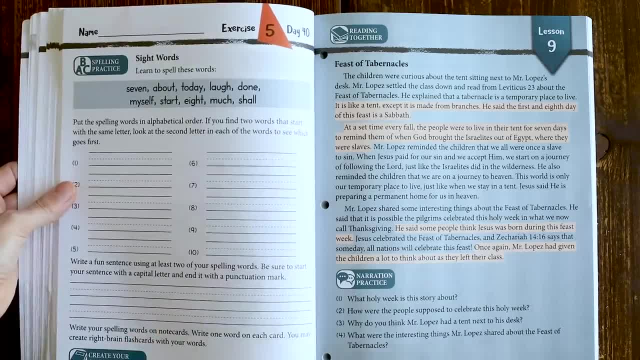 they're studying these Psalms, they're going to be reading the Bible, And then they're going to be reading the Bible, And then they're going to be reading the Psalms, And then they're going to get it. It's getting them to analyze it, It's getting them to ask good questions about it, and 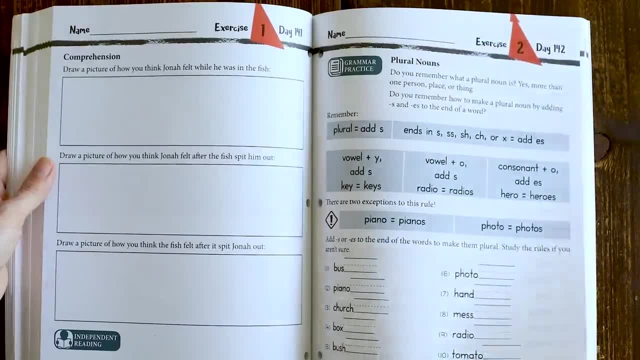 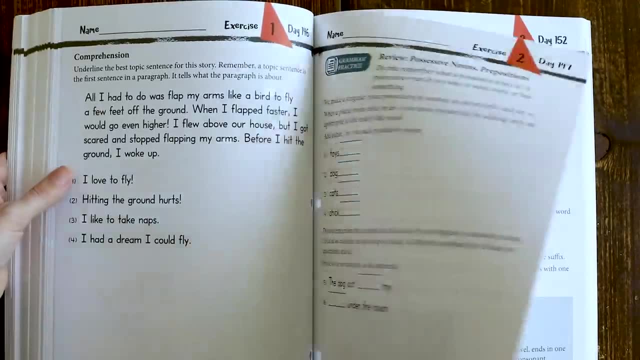 understand. They highlight things they don't understand and ask you. So I think it's very unique in the approach of it And I love how it can be done semi-independently, with just a little bit of direction from the teacher, and it does not take a lot of time. So that is language lessons. 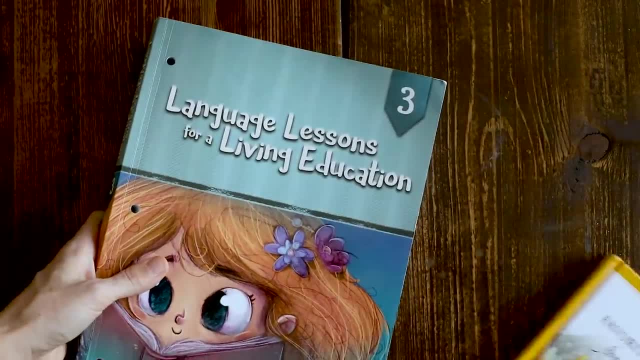 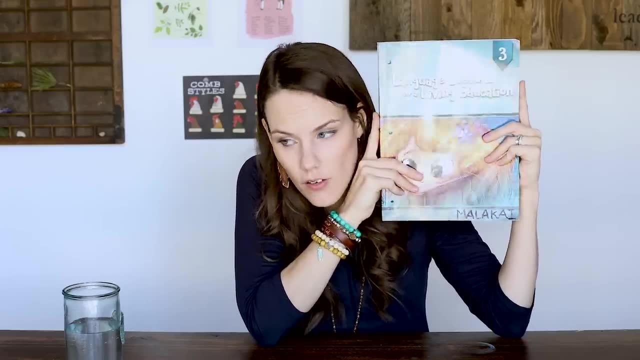 for living education. It is fantastic and it is probably the cheapest option that I'm going to be showing you today, because their levels are incredible, So you'll want to go check those out. That's on masterbookscom: Language lessons for a living. 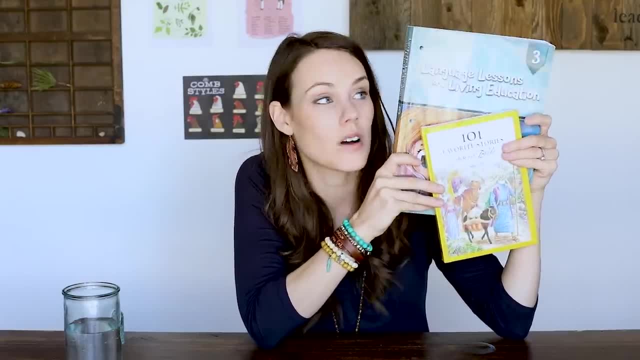 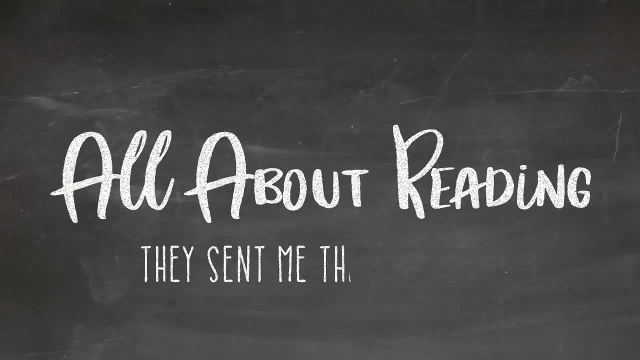 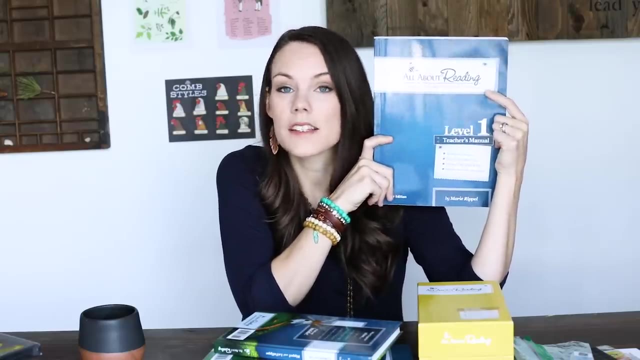 education is an amazing language arts curriculum and it will cover everything that you need for language arts. The next one I want to talk to you about is all about reading. Now, all about reading is from a company called All About Learning Press, which also has All About Spelling, So, together, 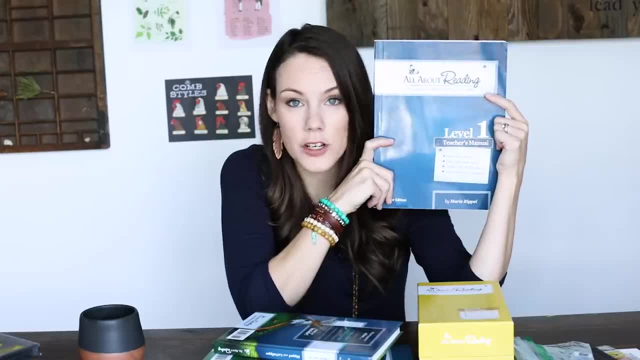 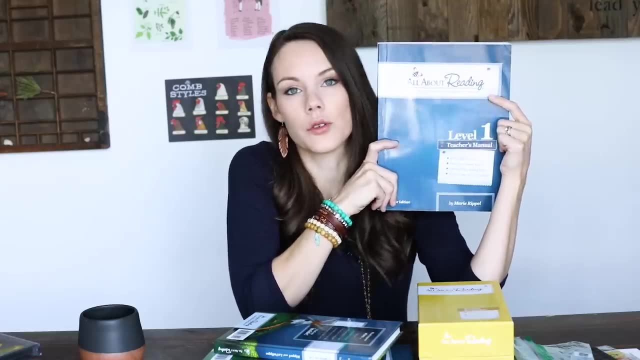 with the two of those, you're going to be able to learn a lot of new things And I'm going to be getting pretty comprehensive language arts, especially in the beginning years. This is a fantastic program to take your kids from not reading at all to reading fluently. So if you 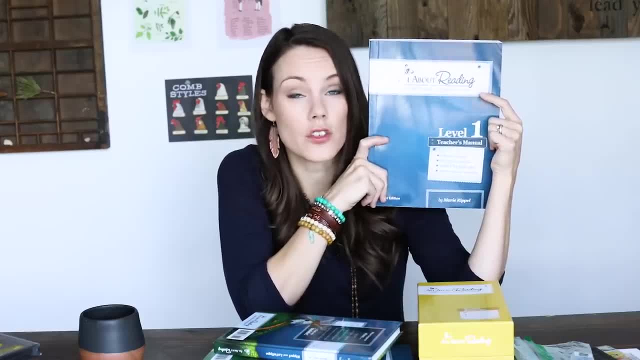 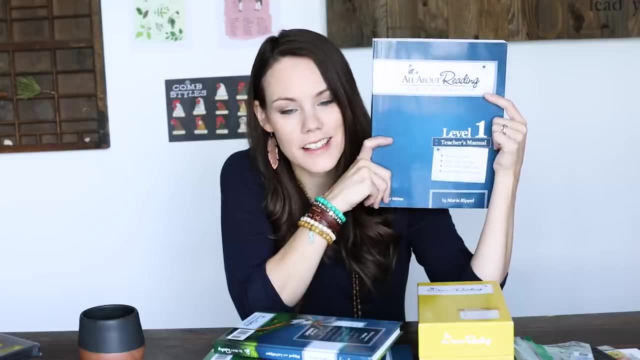 have a struggling reader. this works really, really well and I wanted to make sure to include it. I also guys it was just released in full color, so you get to see that up close and see how beautiful it is inside. But I want to explain a little bit about how this program works and who 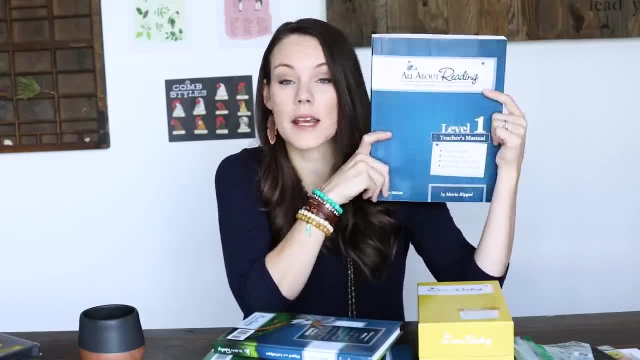 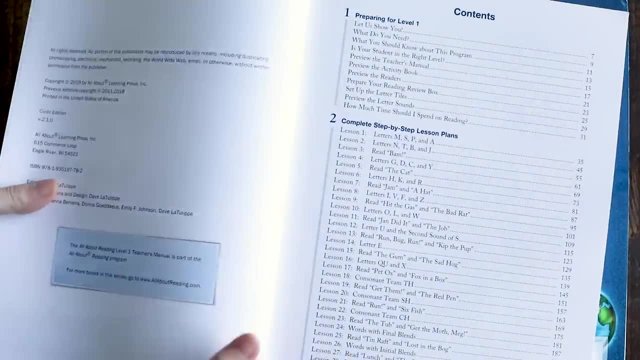 it's going to work the best for. So first let's take a look at the program. So I'm going to take a look at the table of contents here in the teacher's manual So you can see it's got a little bit of how to use it, what to do, and then it has your step-by-step lesson plan. So these are all the. 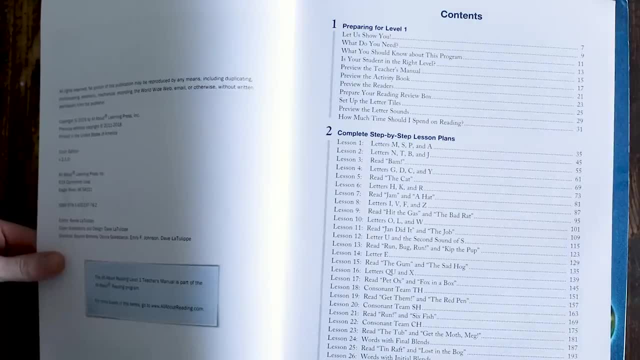 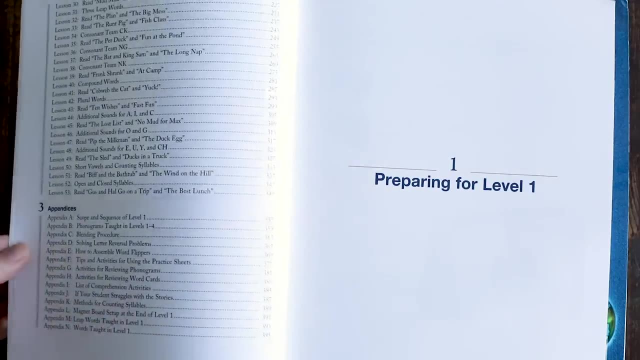 letters. It starts with making sure they understand their actual letter sounds and they're going to be reading books and stories And it does recommend that you also are doing read aloud with them: reading aloud poetry, reading aloud books. So there is a scope and sequence. 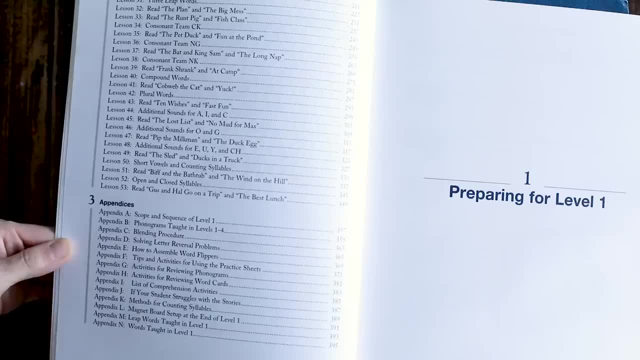 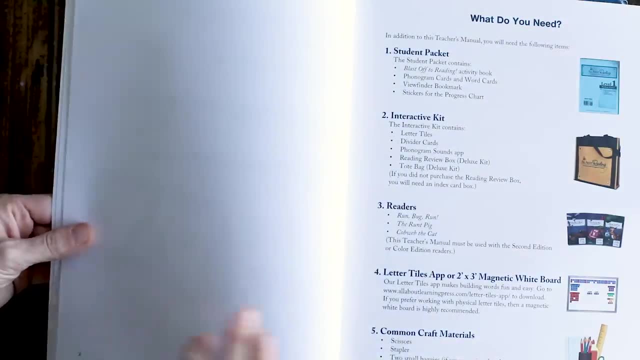 All of your lessons are laid out for you there and it teaches you step-by-step how to actually teach it. And it's really cool because in the teacher's manual itself you actually get to see the full color, you know, flashcards and everything that you should be using. So let's flip through a. 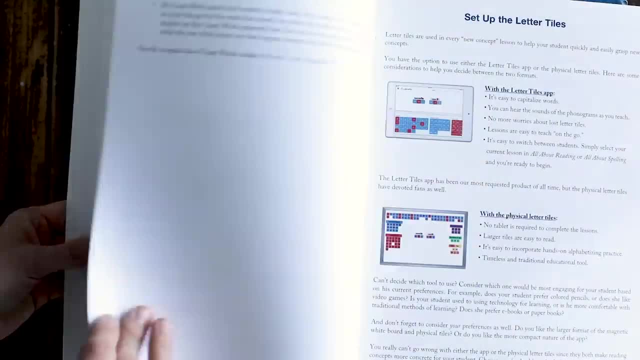 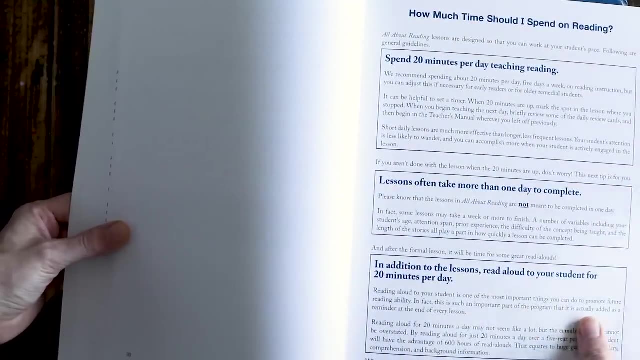 little bit of the teacher's manual so you can see how it works. So it focuses on the five key components of reading: phonological awareness, phonics and decoding, fluency, vocabulary and comprehension. It's a mastery-based program, So, as your 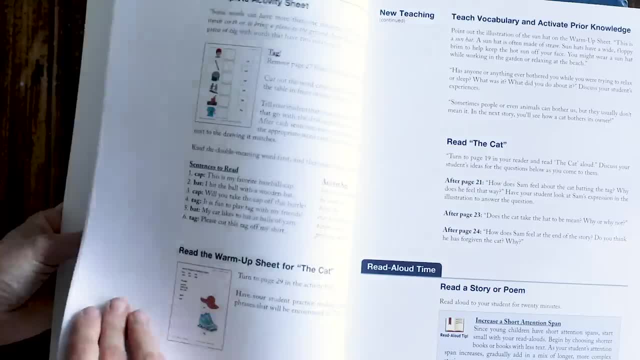 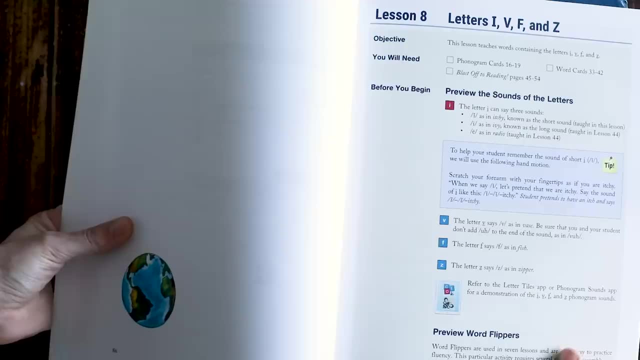 kids are reading even a story. before they read, they have a reading warmup to make sure that they're familiar with the words that are going to be introduced in that story. They also, at the end, you're going to ask questions and make sure that they understand. I think it's really important to 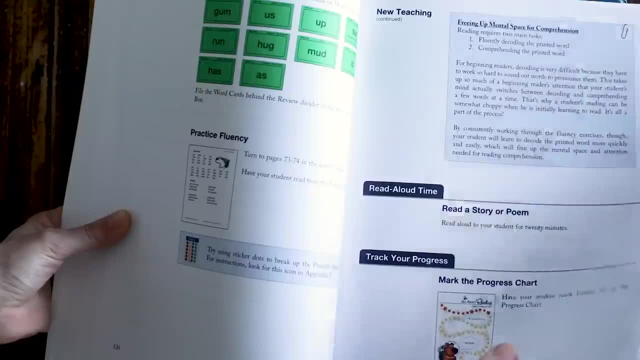 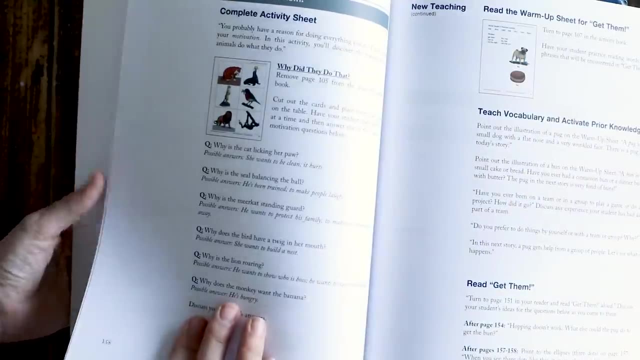 note that they now have alerting. they have an app that goes along with the program. It is their Letter Tiles app. So one of for me, one of the frustrations when I use this way in the past was that it comes with all of the information that they're going to be using. So they're going to 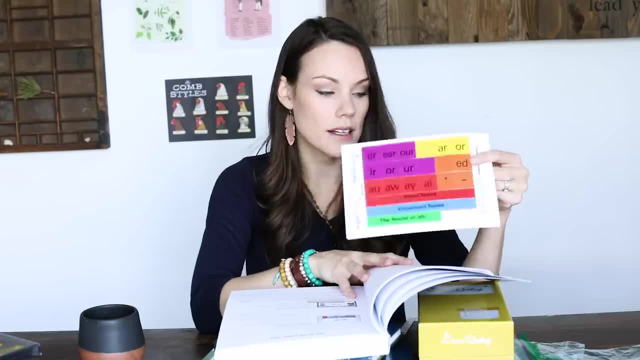 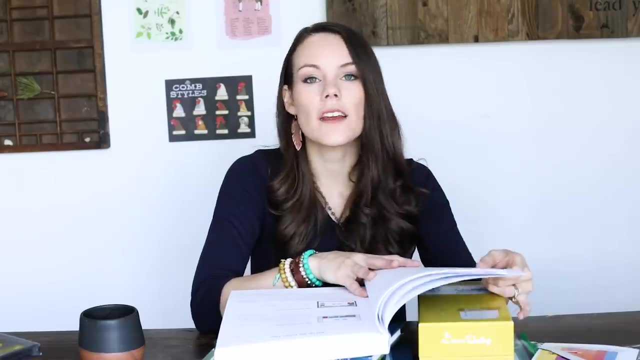 have all of these magnetic um letter tiles and you add magnets to the backs of them And each child is supposed to have a board, or you use a big board and they build their words, which is fantastic. However, they get lost all the time, And so I love. this Letter Tiles app is amazing. 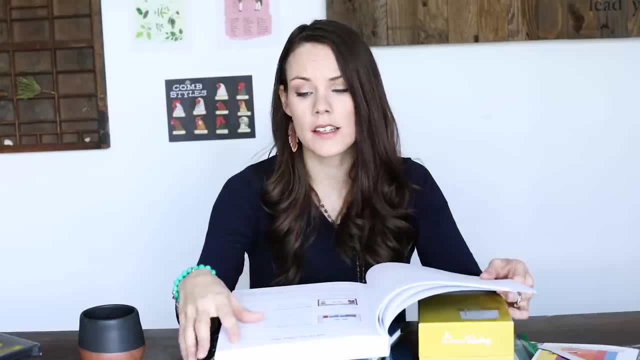 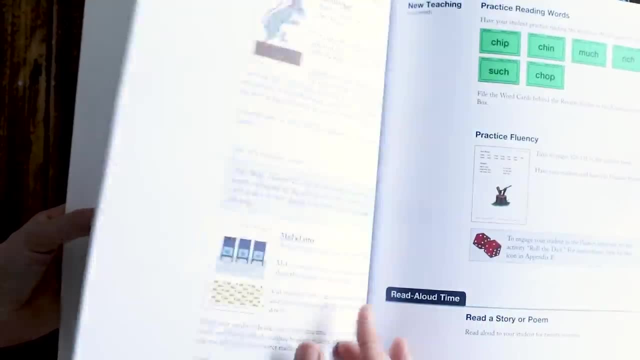 because they can build all their words on there. You can use it for all sorts of different subjects. It's available on the app store and it is highly worth it in my opinion. I purchased that myself. I loved it so much. So you can see kind of the layout of it. It's a little bit more of a 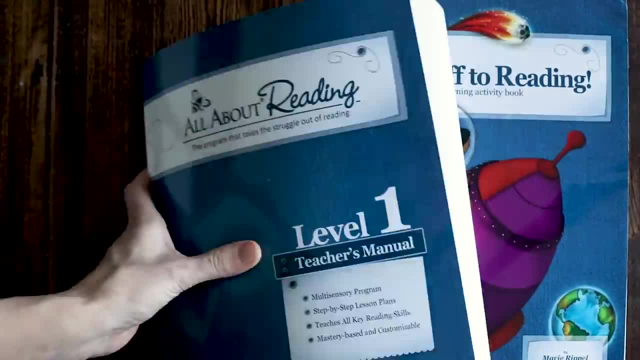 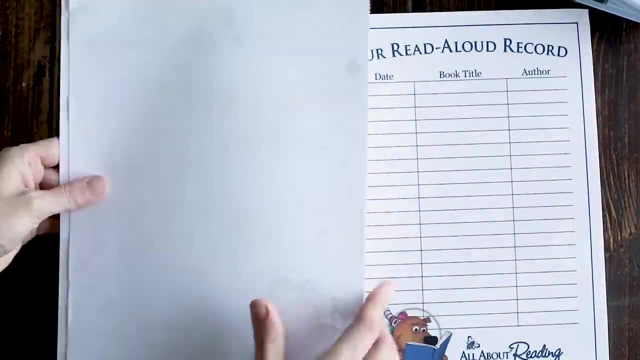 template how it teaches. It's going to tell you: okay, teach this flashcard. You know they're going to do this worksheet, So in the beginning you have this map, that this progress chart. So they put stickers on as they go. There's a read aloud record and then it's just fun things. So there's. 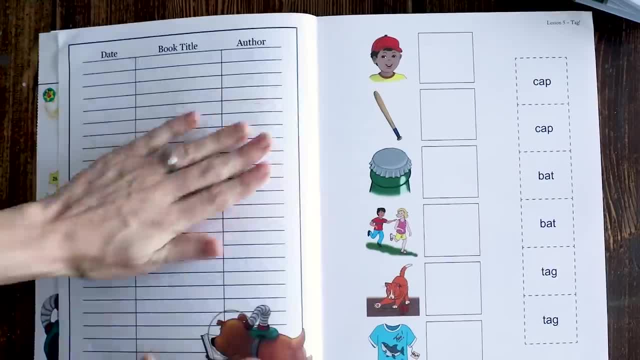 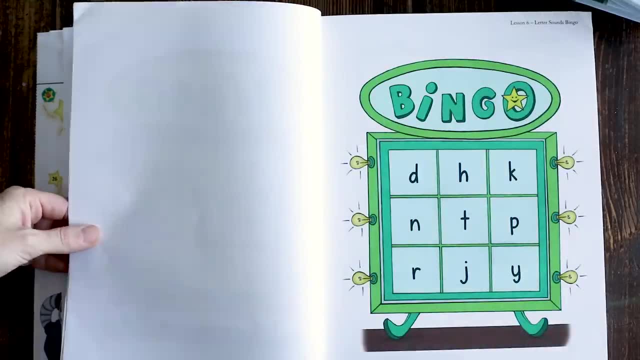 warmups. that that's what you're going to do before you read a story. There is bingo games, there's cutout and paste and then there's practice sheets and your practice sheets. those help with fluency. So if you've got a child that is struggling with fluency, that's where it kind of is all. 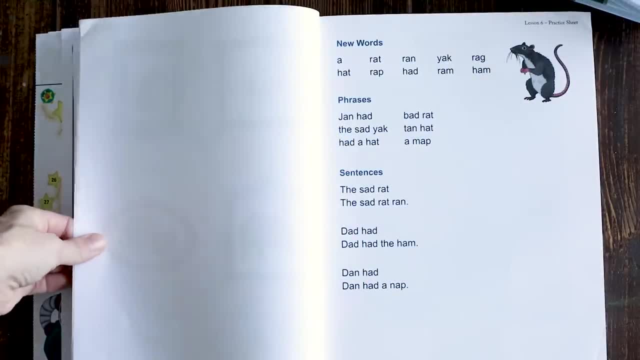 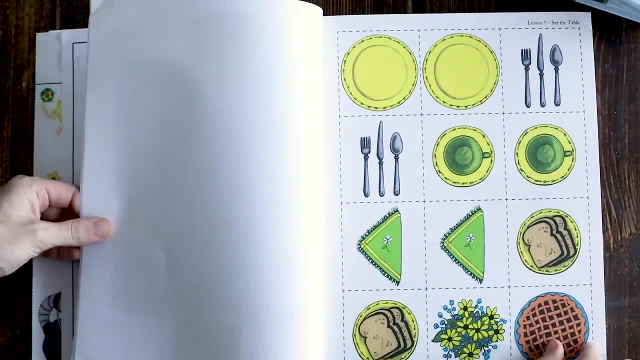 built into this program. It's not just let's teach you how to read, Let's make sure you understand what you're reading and let's make sure that your reading is fluent. It has these word flippers all throughout. So these are kind of little staple books that you're going to flip. 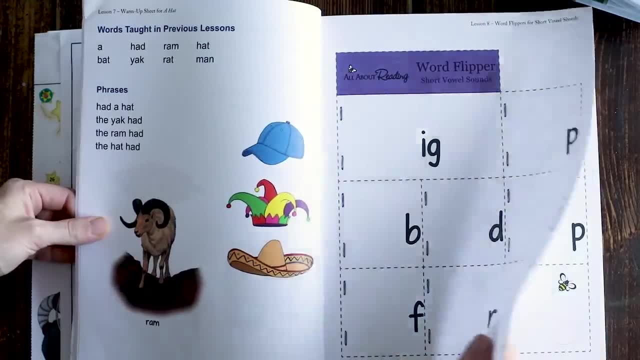 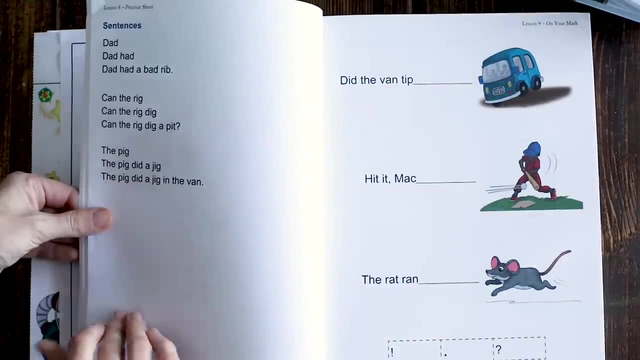 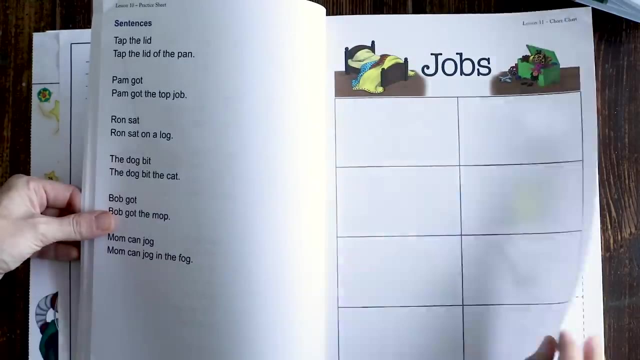 the first and see what that end blend sounds like, with all the first consonants changed. So it's just a fantastic, fantastic program. It's very engaging, very fun. The kids love it. I'm using this right now with my kindergartner at a slower pace because she's a little bit. 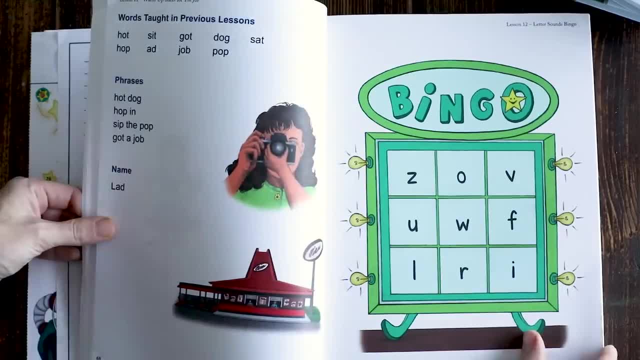 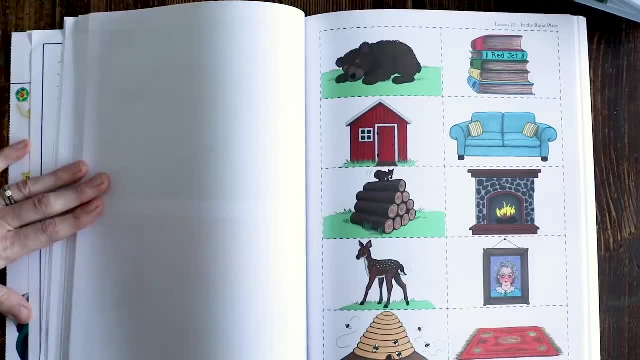 um behind, but she is reading and she was nowhere near ready for that just a little while ago. So the other thing that it includes: give you guys a good look at the inside here. There's so many different pages, Um. the other thing that it includes is: let's just, let's just look at. 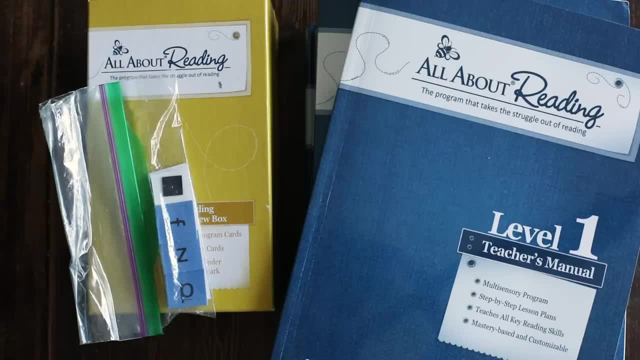 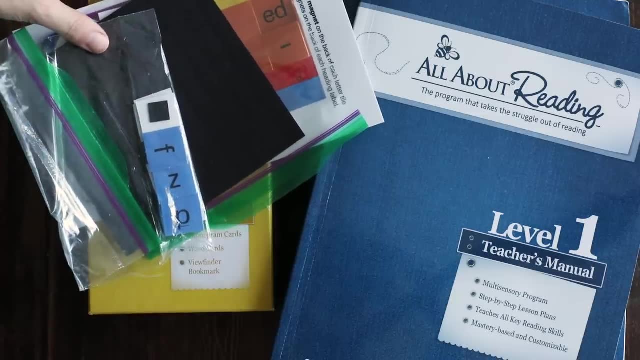 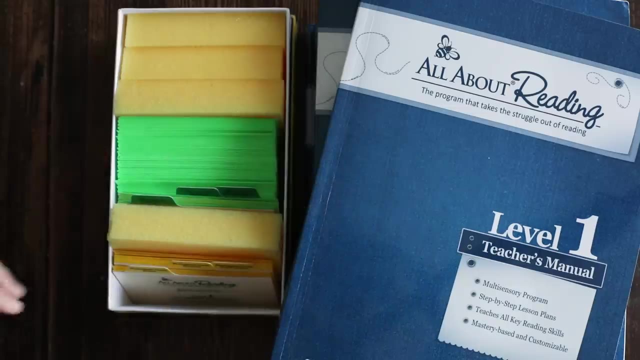 everything it includes here I'm just going to show you up close. So you get your teacher's guide. you get your activity book for the students and, of course, all of your um magnetic tiles that you can build. You also get the the reading review box, So that comes with all of your cards. 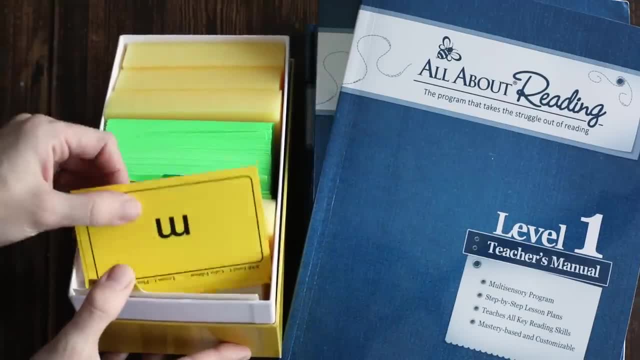 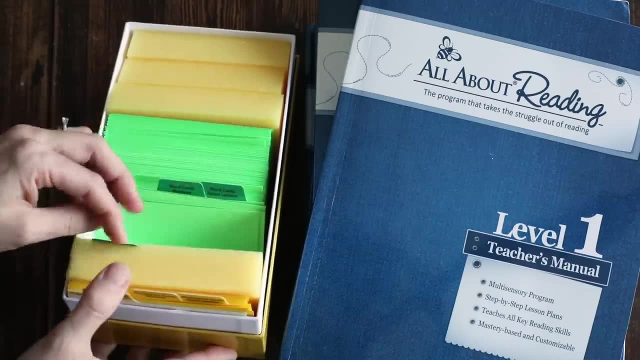 So phonogram cards and the sounds right. So those are ones and you put them in: ones They need to review, ones they've mastered and the ones for future lessons. And then there's also their word cards. So you can see the word cards that they need to review, They've mastered and ones for 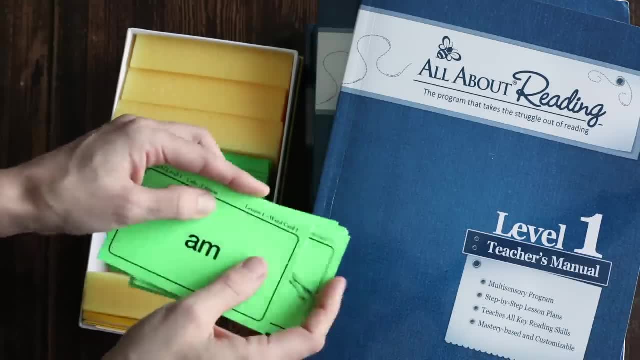 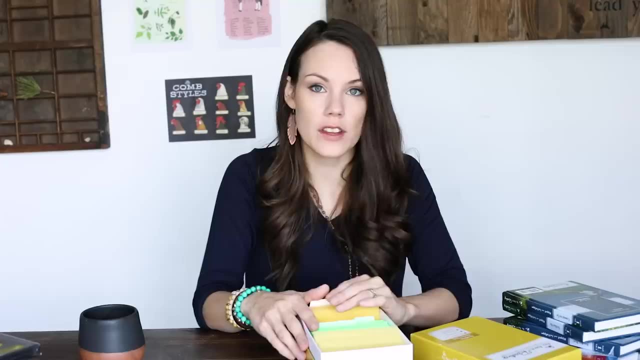 future lessons, And these really, really, really help them with fluency. We're going to go over them so many times that you've mastered them, And then you get the reading review box So you get to master them. So when we read the story, it is not daunting. You don't have to sound everything. 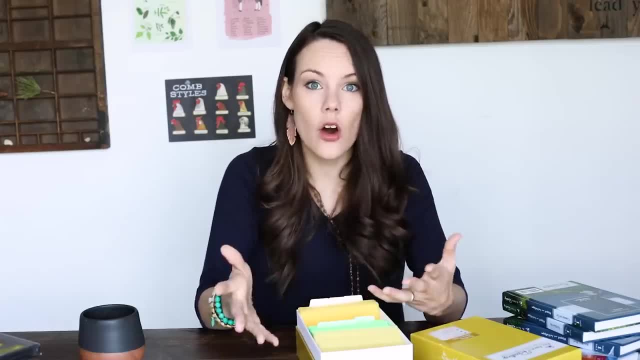 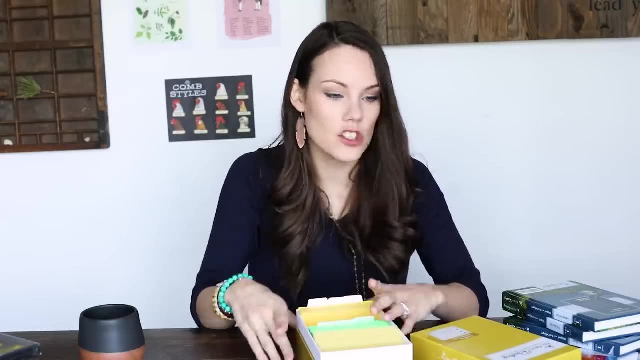 out. It's easy, And so that even builds their confidence, because when they go to actually read the story now it's like, Oh my goodness, I can do this. This is easy, I can read because you've done all the work beforehand with flashcards, with worksheets, with these fluency um practice. 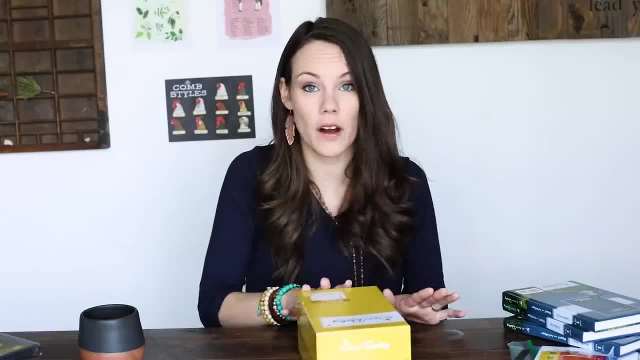 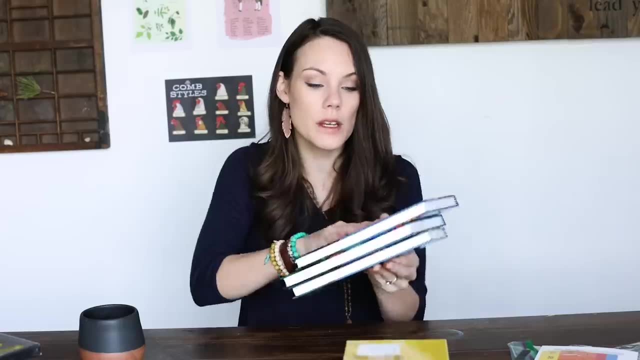 sheets that you're doing and these reading warmups. So by the time you get to that story, it's easy, And that is a huge component of it because it builds that confidence. The other thing that it comes with is three readers, which now, in full color, are just amazing. Um, and I'm going to show you inside these as well. 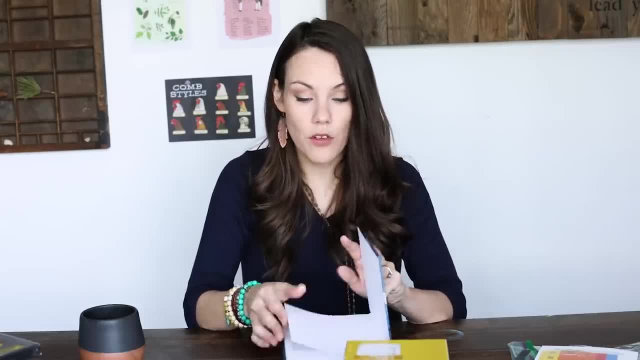 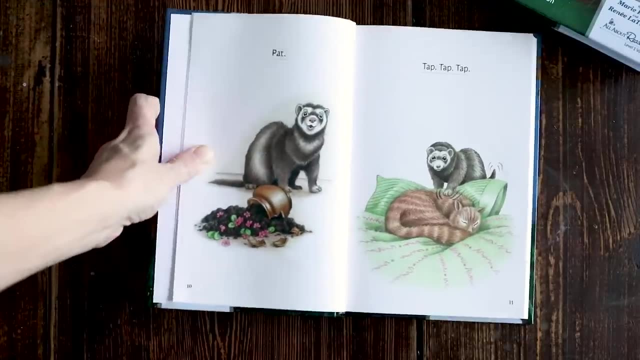 I want you to see what they start off with in volume one, the very first one, And then I want to show you where you end up, all the way to volume three. So just a quick flip through. you can see how beautiful the colors are. You're starting with three letter words: Um. 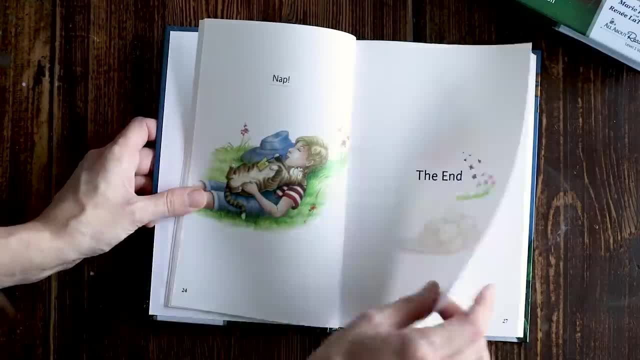 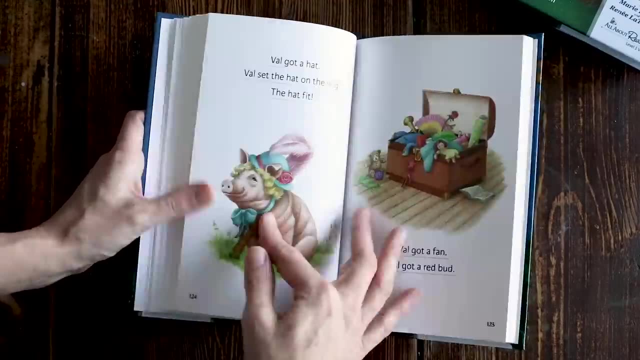 and you know, very simple short stories can be read in a few minutes, And so I just I love the pictures. The stories are funny, They make the kids laugh. Um, they love it, They absolutely love it. So this is volume one, And then in volume two, 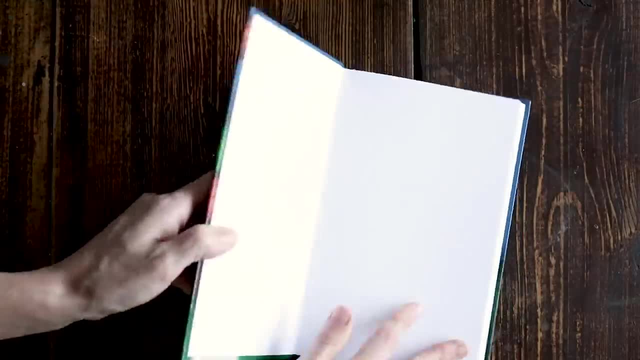 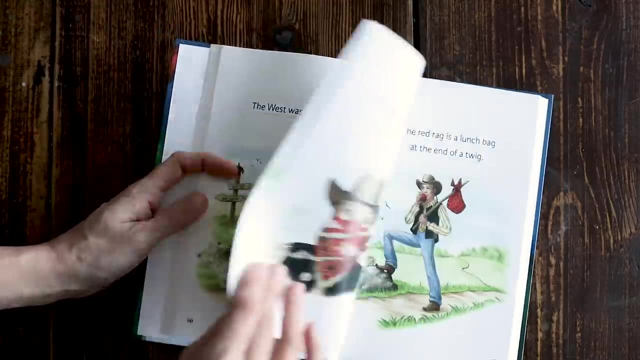 you can see that it's getting a little bit more challenging. We're now getting into longer sentences that they're reading. It's still kind of three to four letter words, but we now have some sound blends that we've we've mastered and have learned at this point. 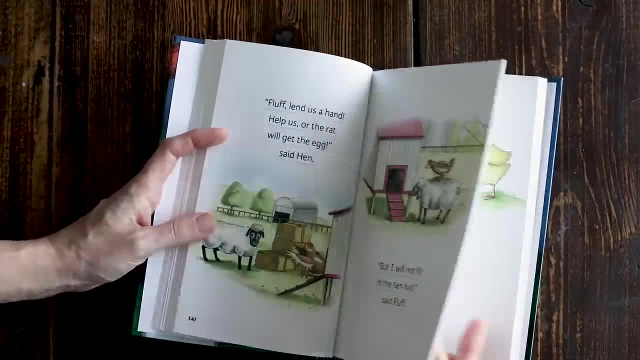 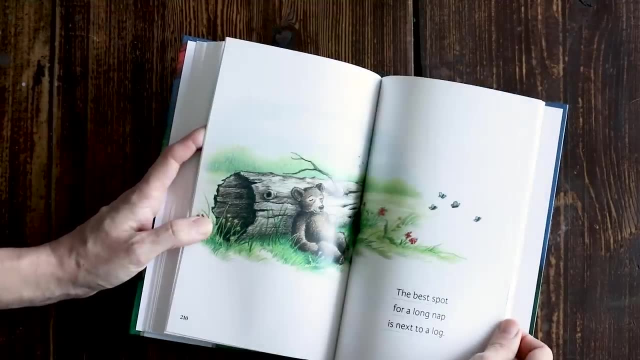 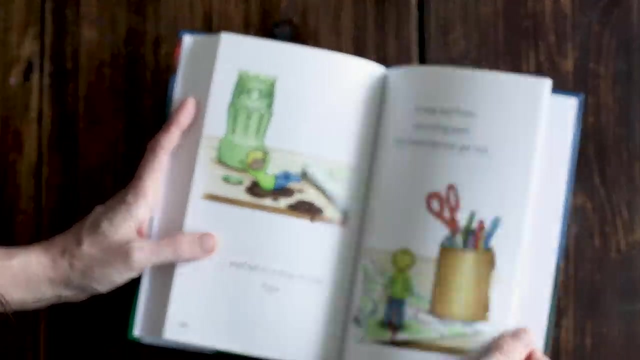 So all just in volume one. you can see that already such an incredible growth. Sometimes this is all you see in one whole year of a level of language arts. So if you are looking for something that's specifically targeted for reading, this is fantastic. So this is volume two, And now, if we take us over to volume three, you're going to see 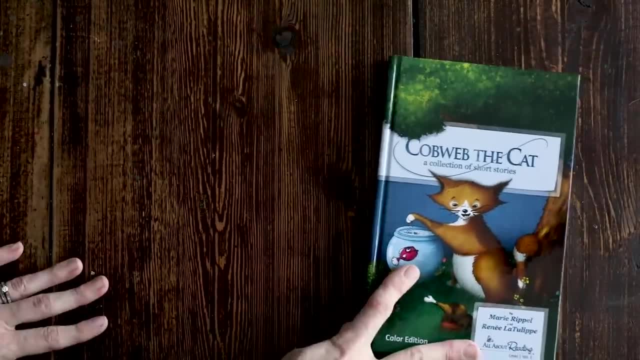 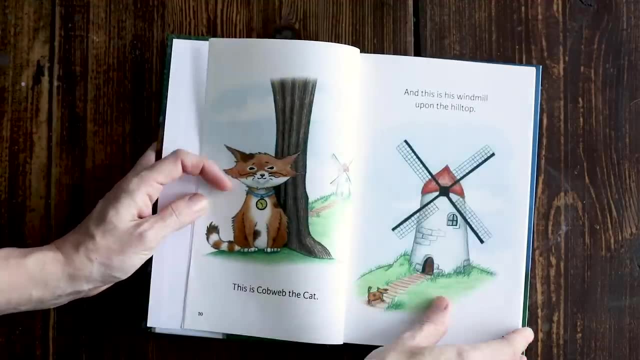 where it takes you towards the end. So again, it's still got the funny, silly stories that are really engaging. beautiful, beautiful full color pictures, um, that really pull the kids in. But now you're getting into almost an easy chapter book kind of thing. Still easy enough to read. 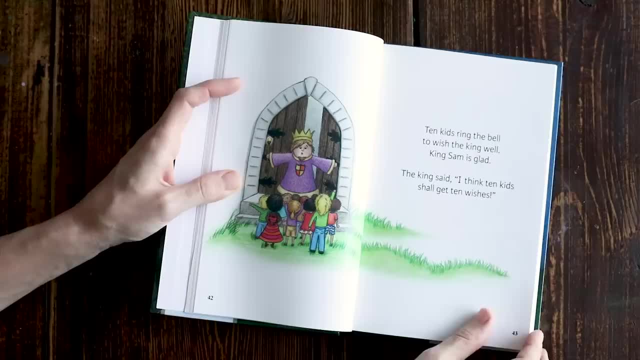 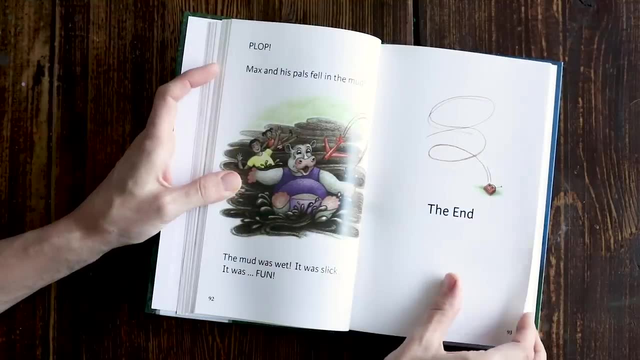 They're not super, super long, but it's getting into lots more writing and um and a little bit more natural writing, And so the kids are are able to read at a more advanced level. So that is where it takes them, beginning to end: three letter words. 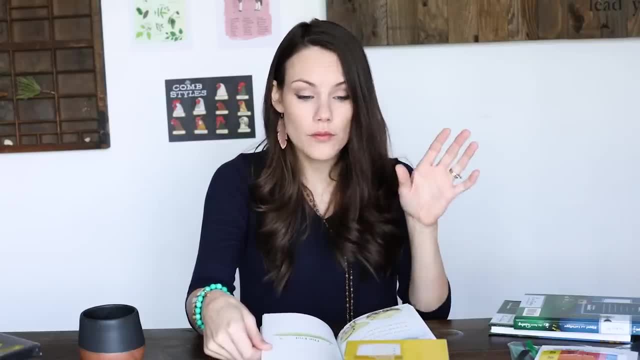 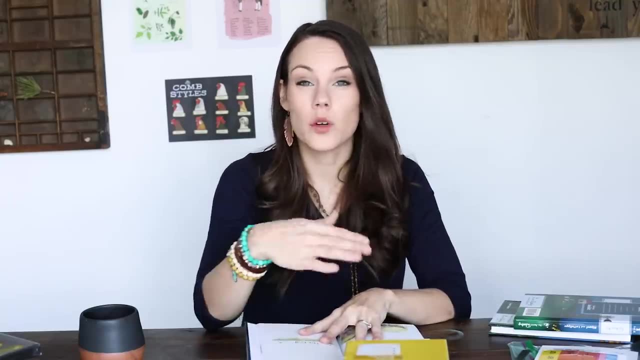 knowing their letters and sounds. They need to know their letters and sounds before you start, their alphabet letters and sounds before you start is is generally a good idea, Um, otherwise you're going to want to start with their pre-reading one, So, but this takes them. 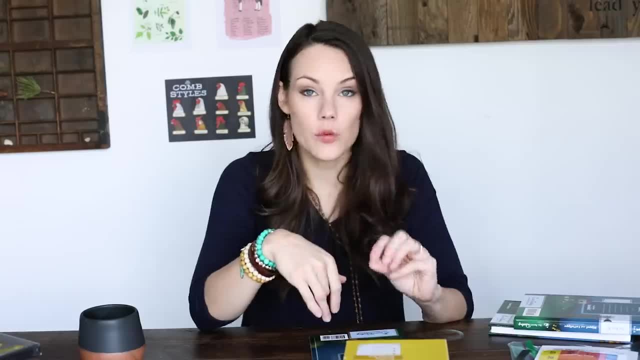 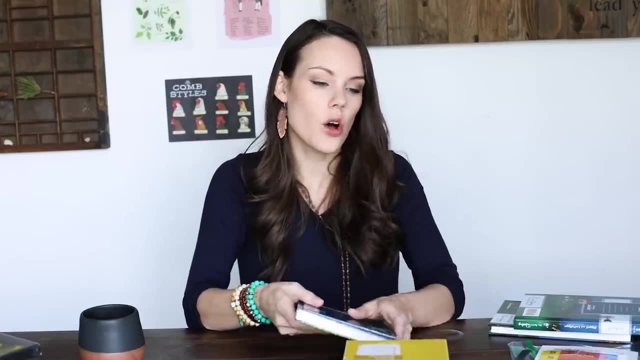 from. okay, now that we know our letters and sounds, we'll start to learn blends. We'll start with words: How do they fit together? And let's, let's figure out you know the sound blends and the different sounds that these letters can make, kind of thing. So it is an amazing program. who? 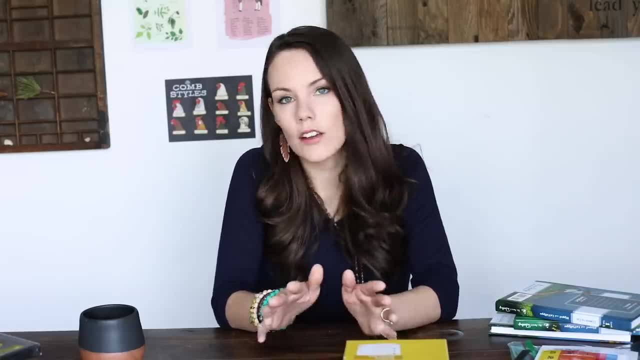 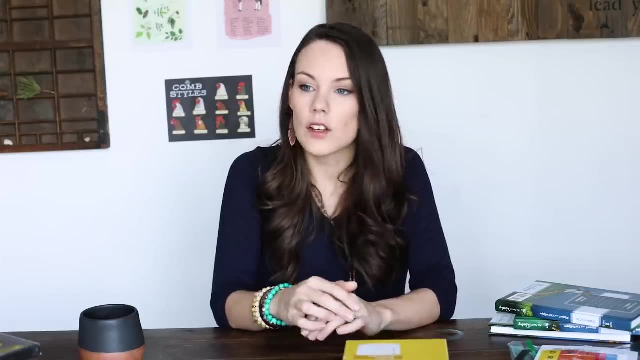 this is going to work well for anybody who is looking for something that is really targeted to reading. If you have a lots of language arts programs, do not give that targeted reading instruction. They'll say go read for 20 minutes, but they do not give that phonics based teaching. 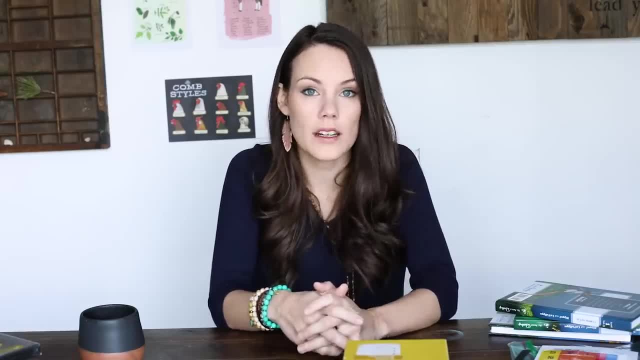 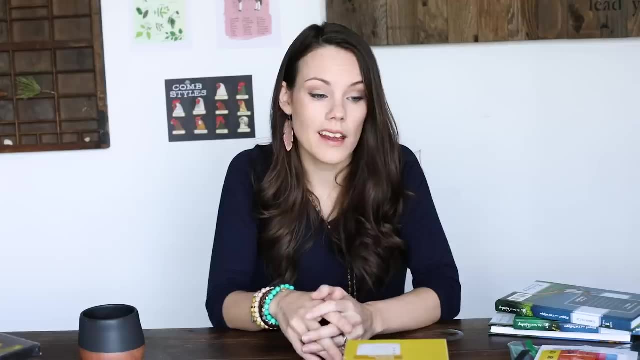 for a reading program. If you are looking for a phonics based program for reading to really give your kids mastery and a strong start In reading, this is going to be a really good fit for you. If you are looking for something that is, 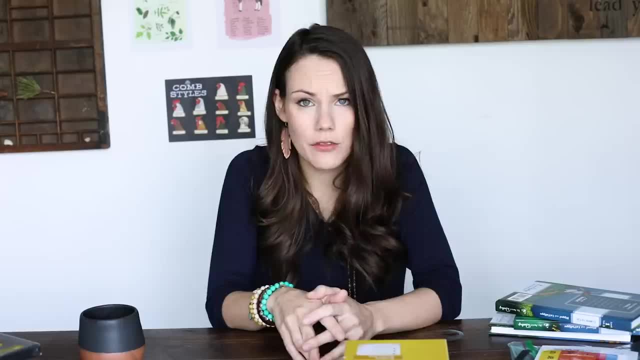 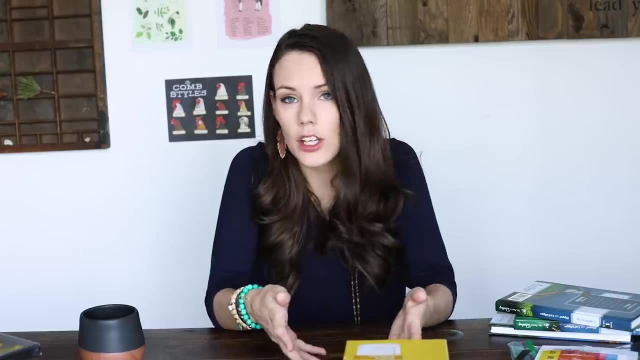 great for kinesthetic or visual learners. this is going to be great for you. It works also really well with auditory. Really, it targets all of the learning styles because you know they're going to be hearing you teach and hearing those sounds, And so it works well for really all learning. 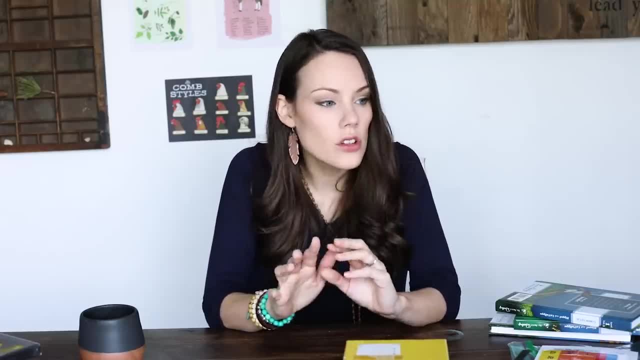 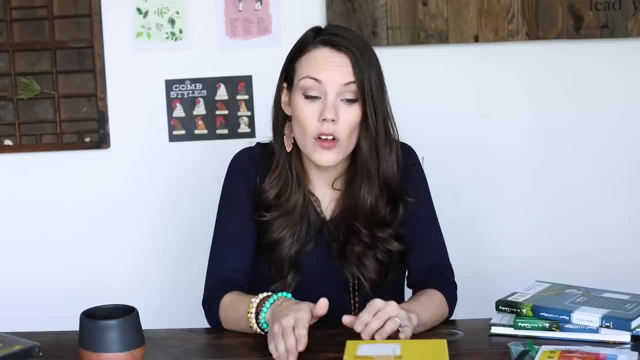 styles, but specifically if you have a kinesthetic learner. there's a lot of programs that aren't geared for kinesthetic learners, So I think that's a huge plus. It's something to keep in mind. It also has been proven time and time again to be incredibly. 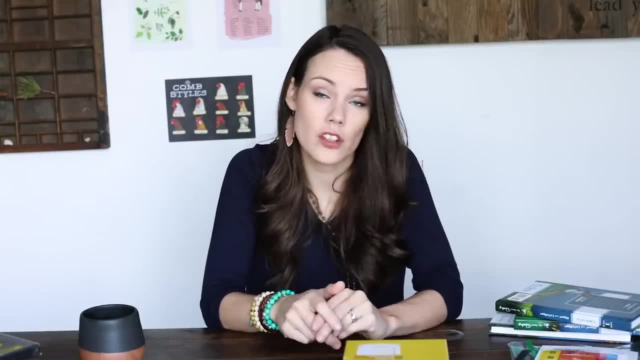 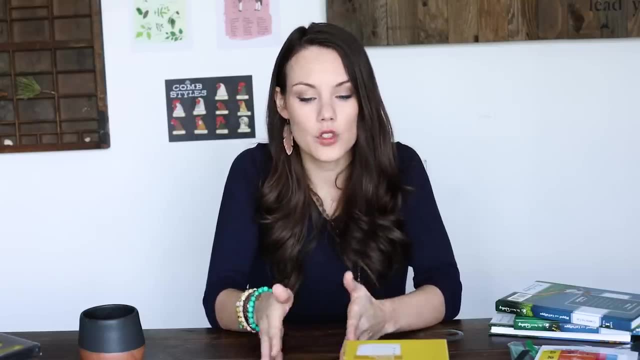 successful for kids with dyslexia or any sort of learning disabilities or challenges. So that's another thing to keep in mind if you've got a struggling learner, that this program can really help them see, visualize and build those words, And it's just proven to be hugely successful. 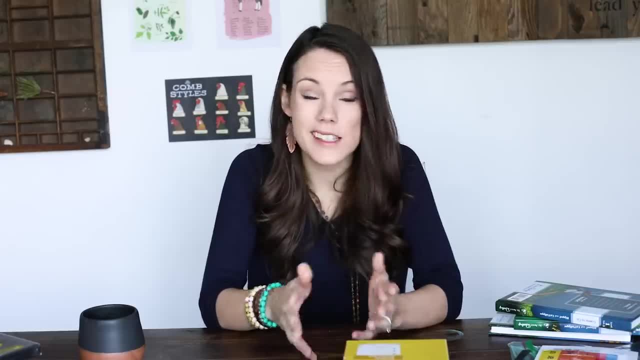 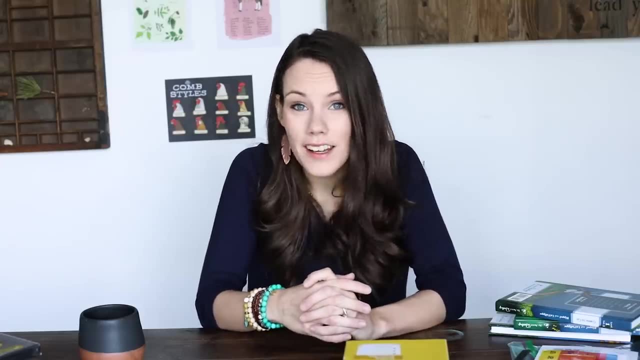 So those are all you know major pros, I think, of this program. It's secular, so it's you know it's going to work for a secular or Christian, depending on what you're looking for. The stories are funny, engaging and you know great quality. So all of those things are huge pros with this. 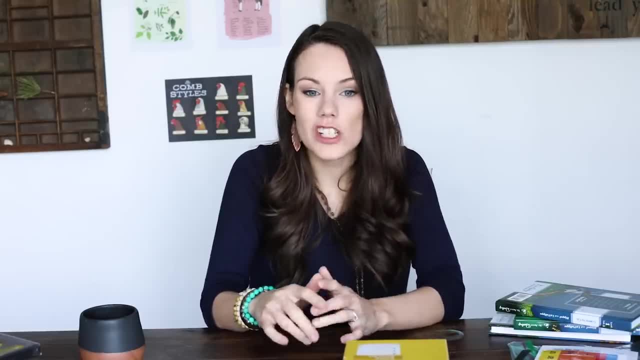 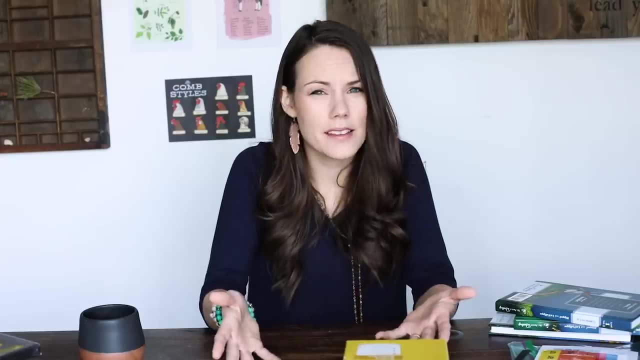 program. Who this might not work for is anybody who just does not have the time. It's teacher-led. You're going to have to sit down with your child and you're going to have to teach it Again. keep in mind that anytime you teach a child to read, it doesn't matter what program. 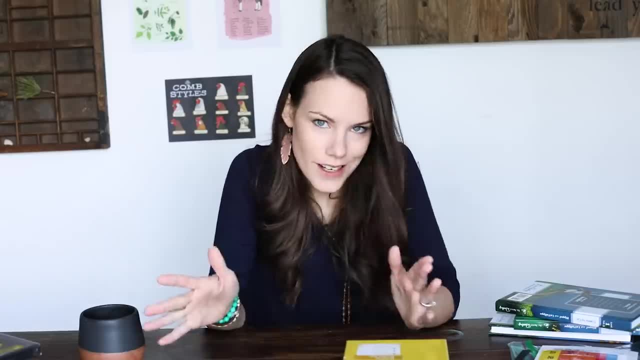 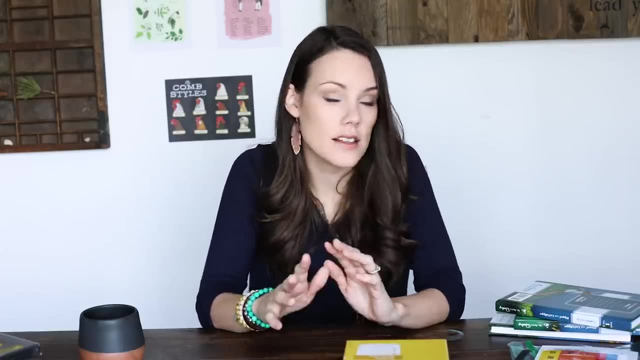 you use in the whole entire world. you have to teach them, So, unfortunately, that is just part of teaching your child to read. However, that being said, you know there's online resources, there's apps, there's different resources you can use that are a little bit. 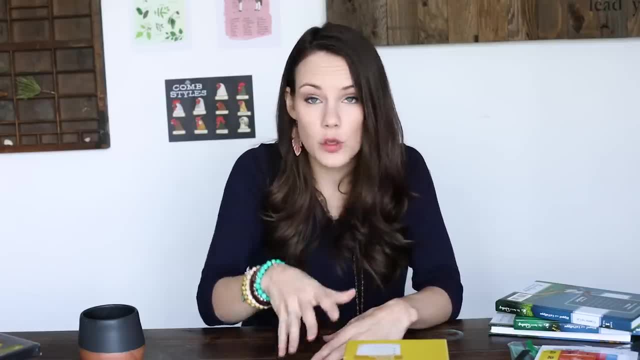 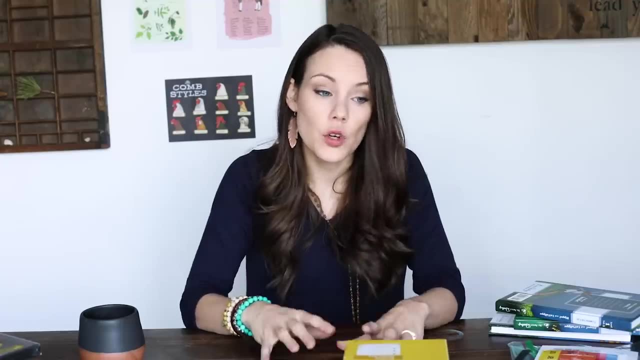 take that pressure off you as a teacher. So if you are working, like I said, if you're super busy, you've got kids all different age levels and you do not have the time to really invest in teaching your child to read, then you might need to look for something. 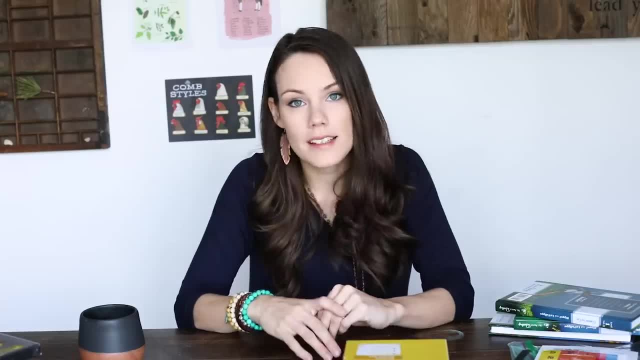 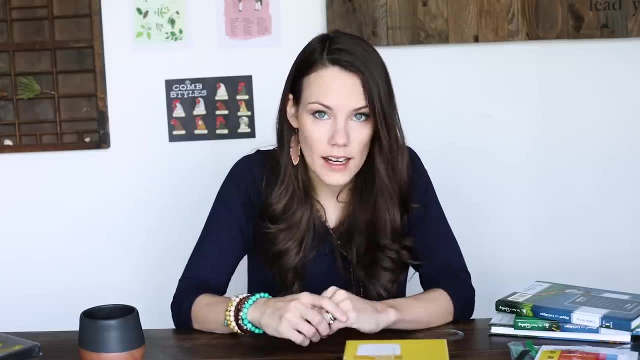 that is a little bit more independent. So just keep that in mind. This is teacher-led. You're going to need to sit with your child and it encourages read-alouds and it's going to encourage you to read aloud with your child for 20 minutes a day. So for us, that's no. 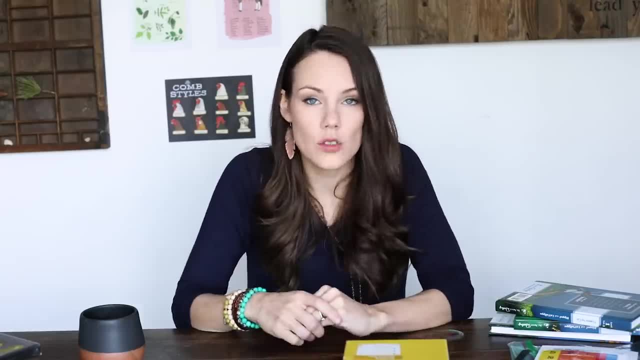 problem. We do read-alouds all the time, And so they're all really, really helpful. So that's what we're going to talk about today. So thank you so much for joining us for this video. We'll see you in the next one. 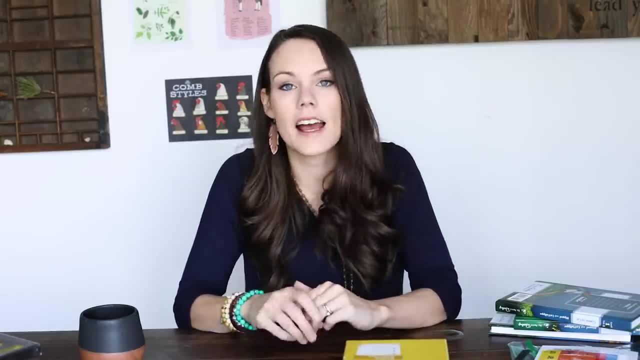 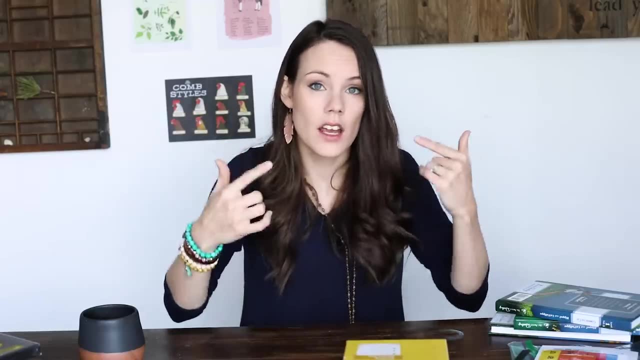 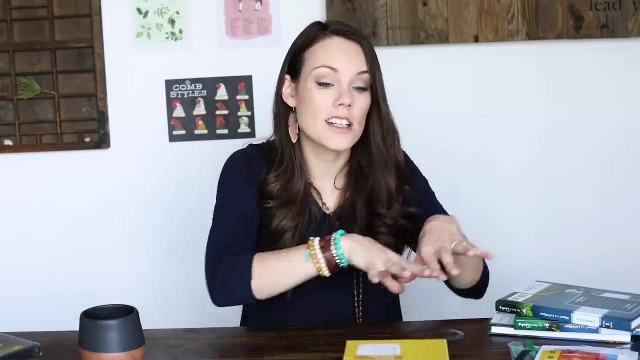 Bye-bye. So that's who I think is going to work well for and who it won't. Price-wise to get yourself started is a little bit more pricey It's. I don't even know the exact price, but I will. 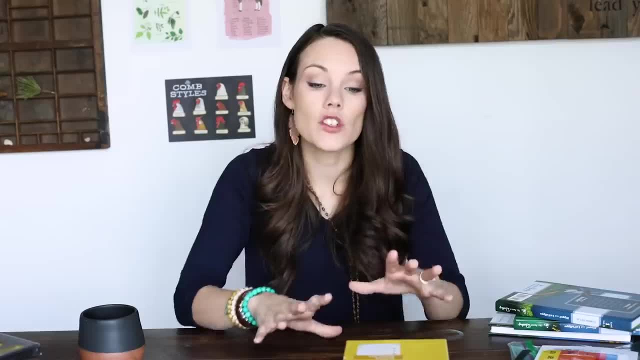 link it below, but it is a little bit more pricey to get started. However, once you have your cards, once you have your books, once you have your books, once you have your books, you know your books, you know the books, you have your books and they're all going. 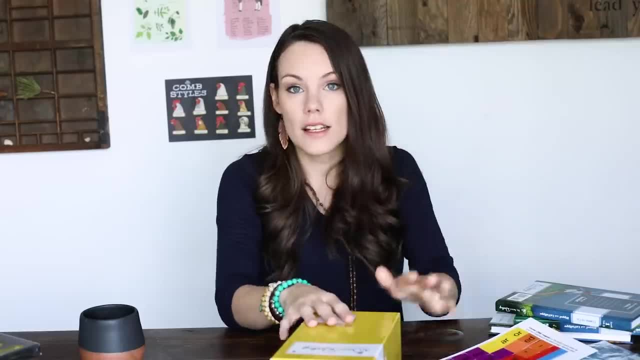 to work well. So that's one thing. So thank you so much for tuning in. See you next week. Bye-bye your, your these things. then it's a lot easier because now you're just getting your workbooks or teachers guides and your your books that you can again pass. 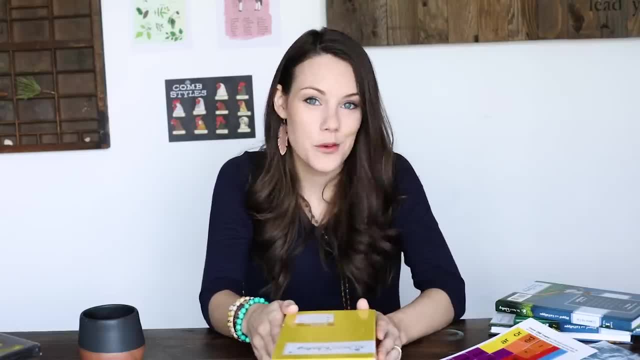 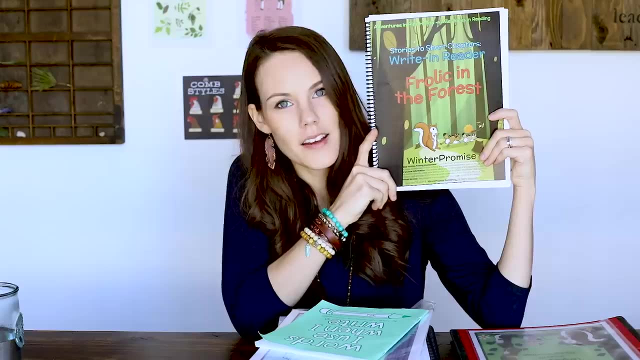 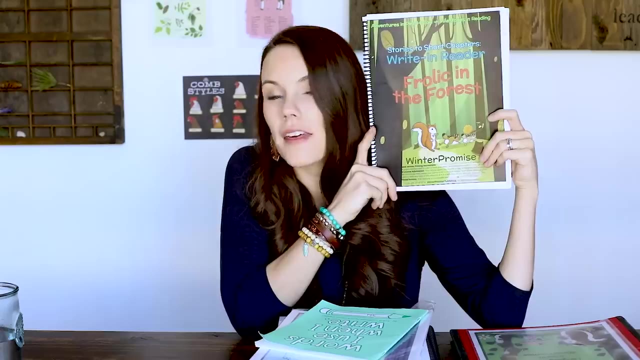 down to younger kids. so just all things to keep in mind when you're considering this program for your family. the next one that I'm going to show you is from winter promise. now, winter promise has similar to my father's world. they have not just their language arts, but they also have themes, and their themes would 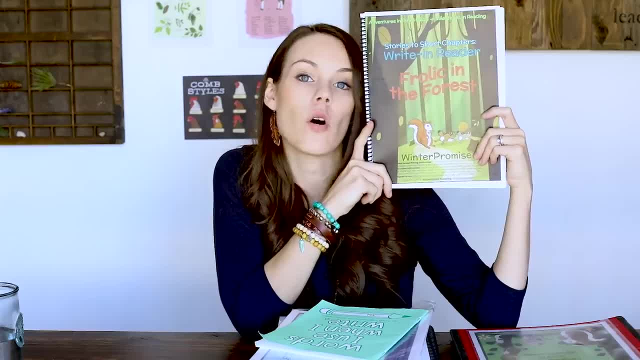 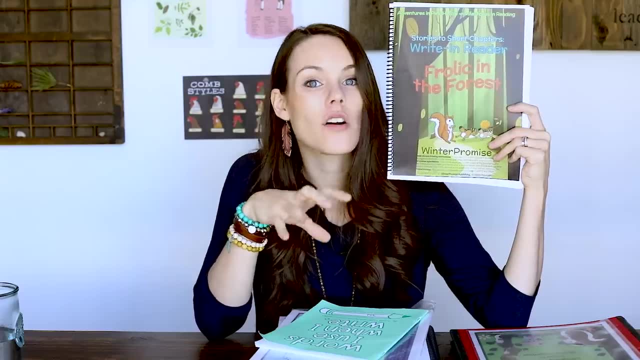 incorporate your science or your history or your Bible and all of those other things, and then you would add in your language arts and your math. now their language arts are different, however, because they are their own resources. these are not ones that have been adapted. these are or just pulling from. 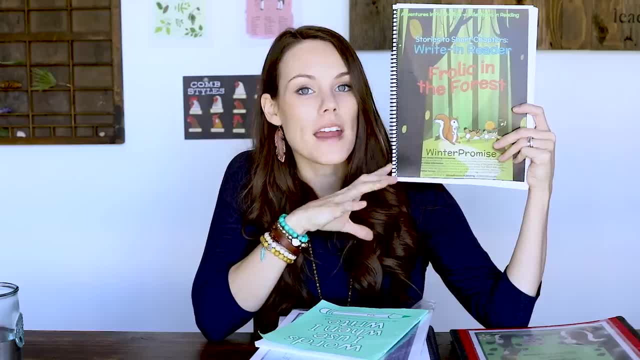 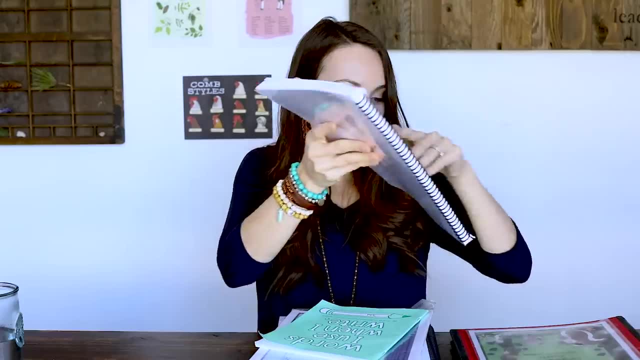 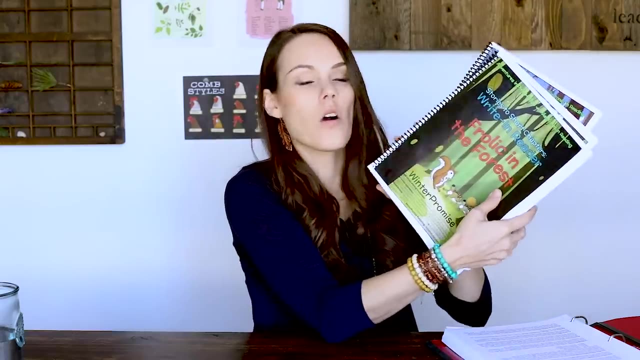 other resources. these are actually their own resources, so they have created different series. where it is written by them, it's very, very unique. you So I'm going to be showing you inside stories to short chapters and the approach of it. okay, so the first thing you're going to see is there is four of 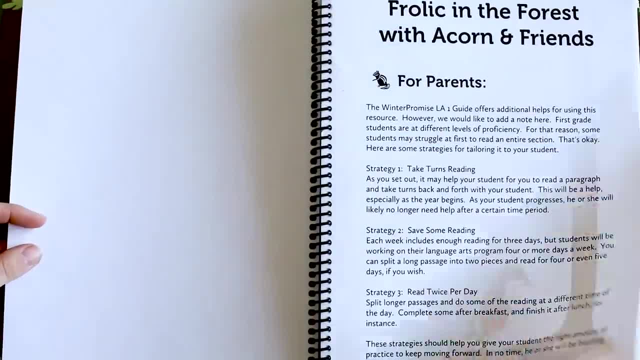 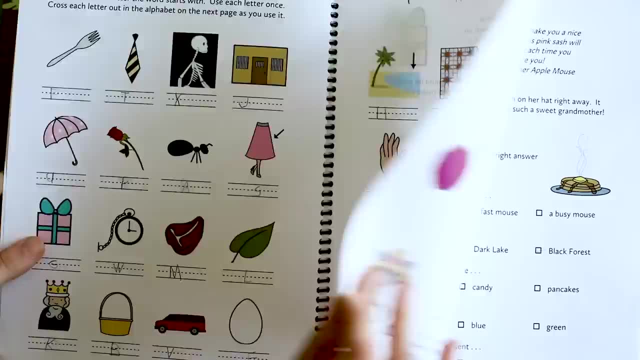 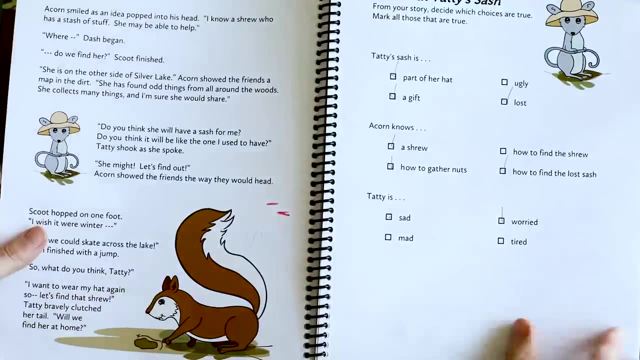 these stories to short chapters right in readers. so inside here they're going to be doing their reading and they're going to be doing any writing, any copy work that they're doing throughout their their year. so the reading in the beginning is going to be challenging and so you're going to have to do a little. 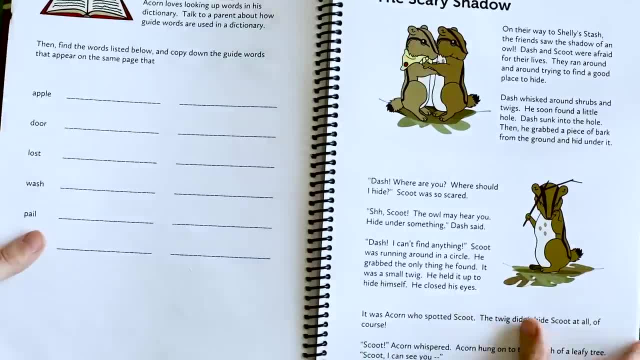 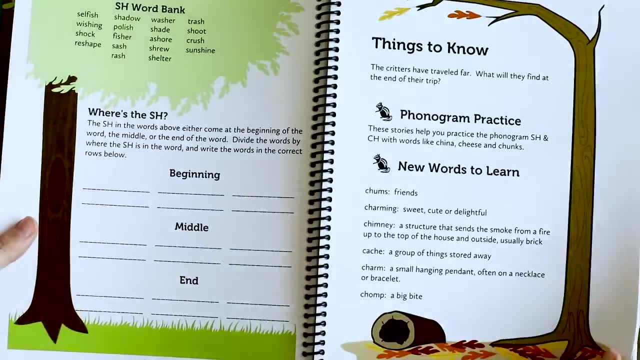 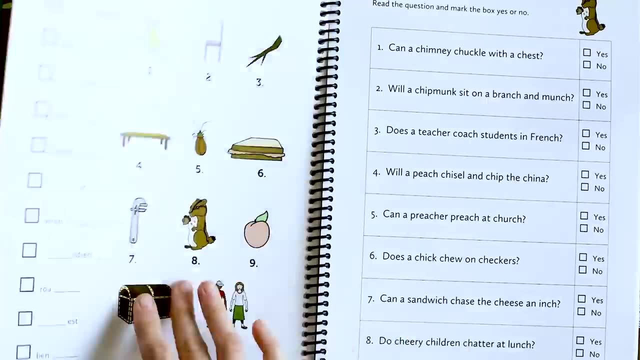 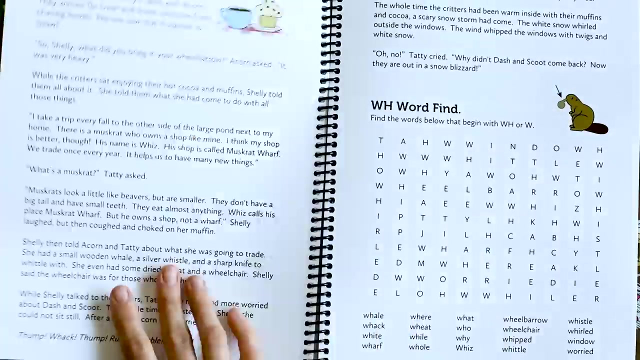 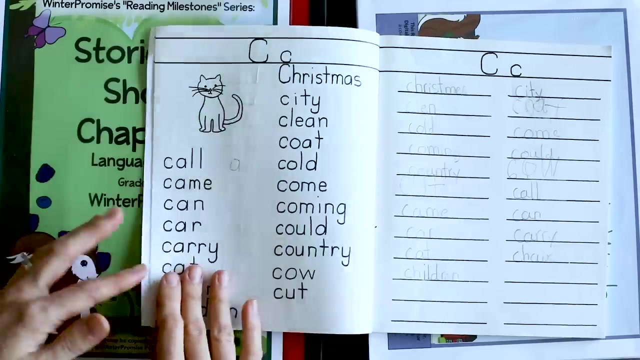 bit of it with them, but it is a very, you know, bright and fun. it's very bright and fun program, and so you can see the way it is laid out here. okay, the next thing that is included is words I use when I write. this is something that they're going to be working on in their writing, so this is: 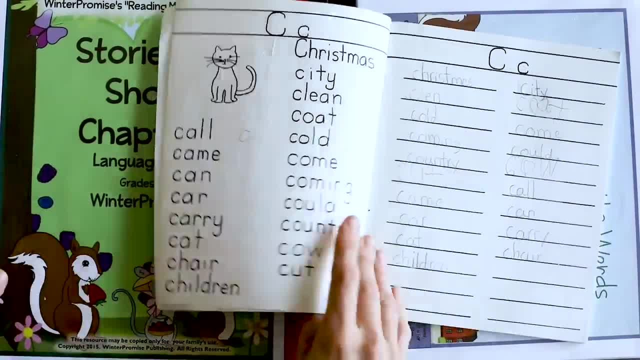 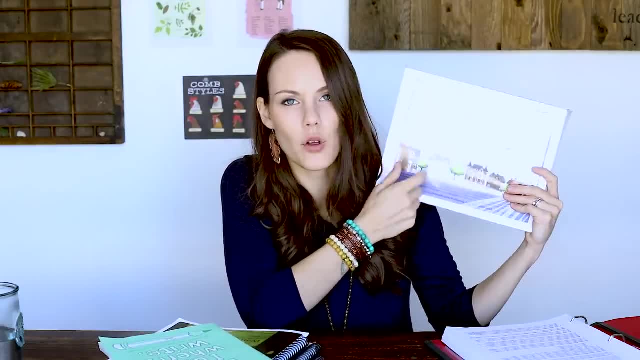 building kind of their own little dictionary and working on spelling. They're also going to have a handwriting set that has their handwriting pages in it. This is one I have from a younger level but I wanted to make sure I showed you that there is a handwriting set included. 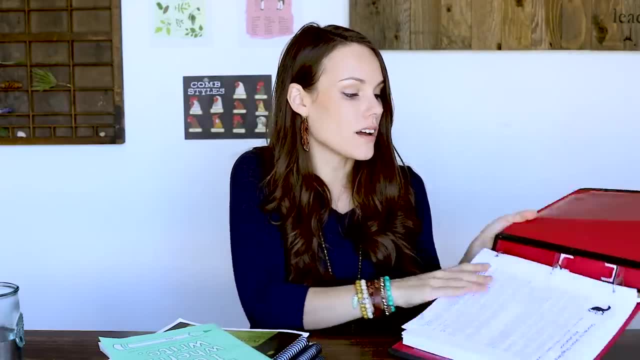 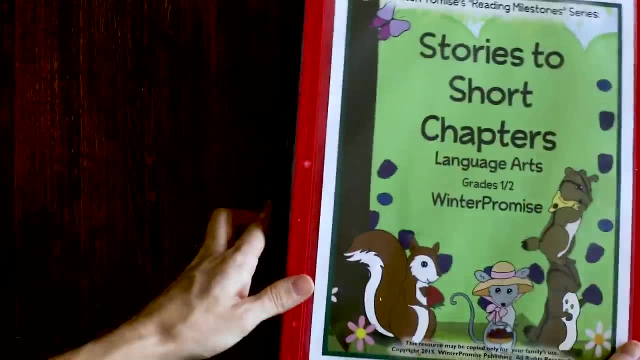 with it And then you have your actual guide, which is sent from the company, which I put into a binder here. So it tells you how to use the program and it has a very easy schedule that you can follow, and it is laid out on a four day schedule. 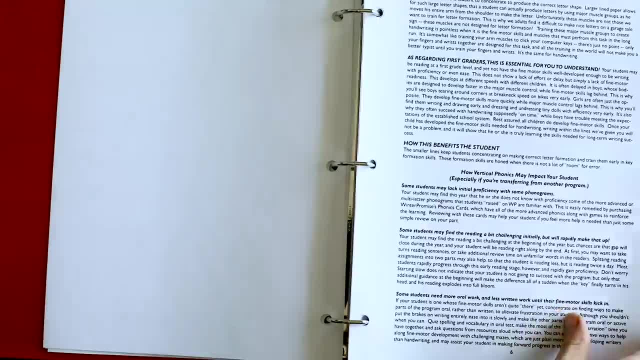 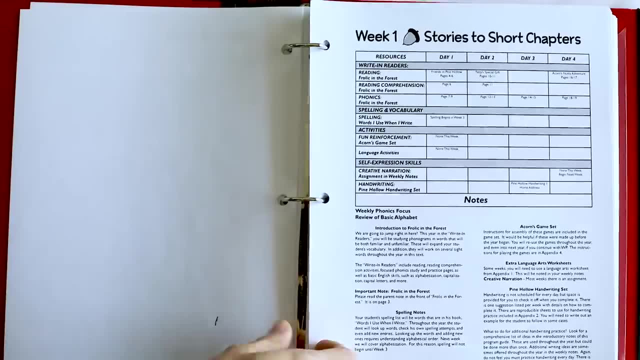 So you can see that here and you can see it is telling you exactly what resources you're using and what you need to be doing. It also comes with a game set that I do not have here to show you, but they're going to be working on a game throughout the year and uh. 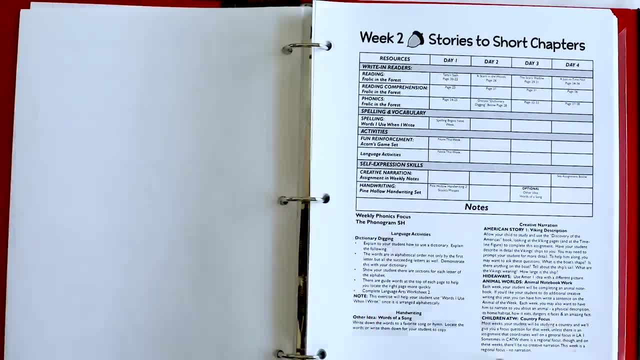 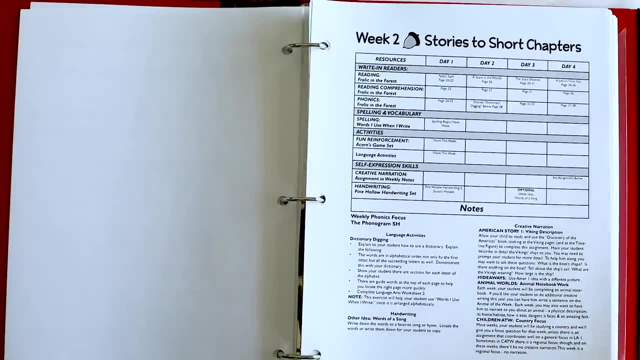 and doing different: reading, comprehension, phonics, handwriting, all of that different kind of thing. So it also will show you how you can adapt it with any of their themes, because you could choose different themes and you know depending on which one you were using. 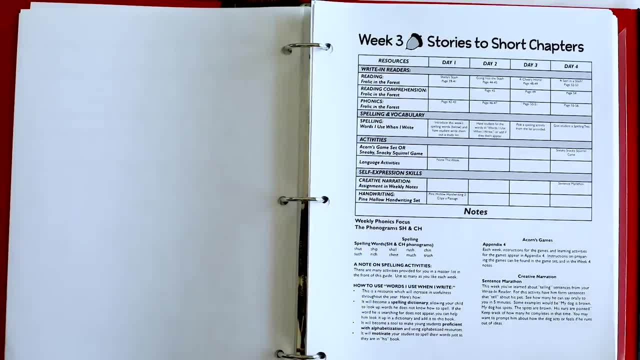 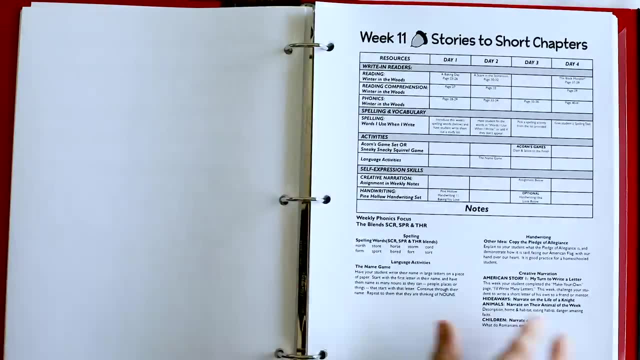 it would tell you what you would be doing for that And how that would integrate with this as well, And then any of the other. there's also some extra language activity worksheets that are in the back of the program. So that is Winter Promise. 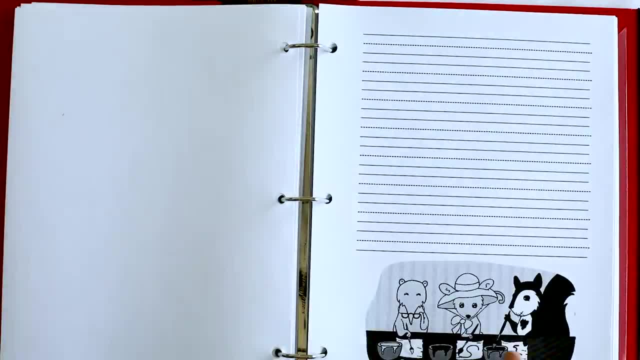 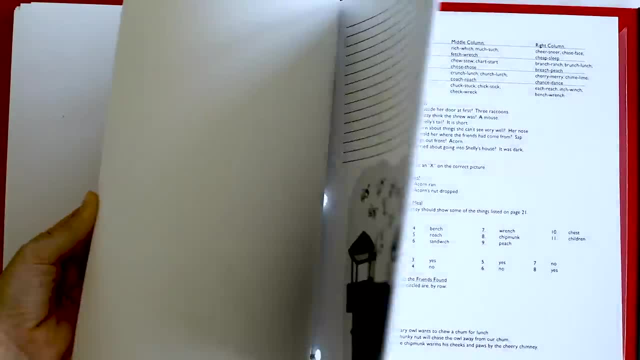 It is definitely on the higher end for language art, So that's something to keep in mind. It is Christian based. Winter Promise is Christian based. for sure, though their language arts itself it is not really so integrated that I don't think that that could be a huge. 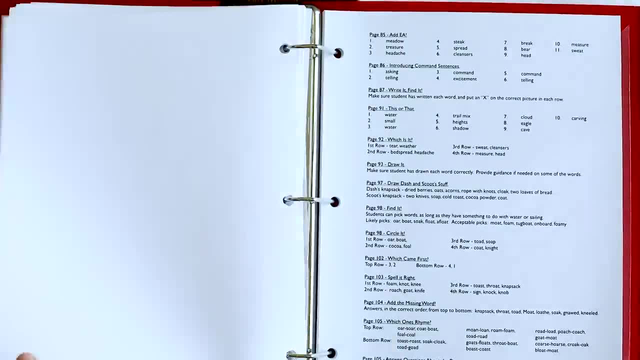 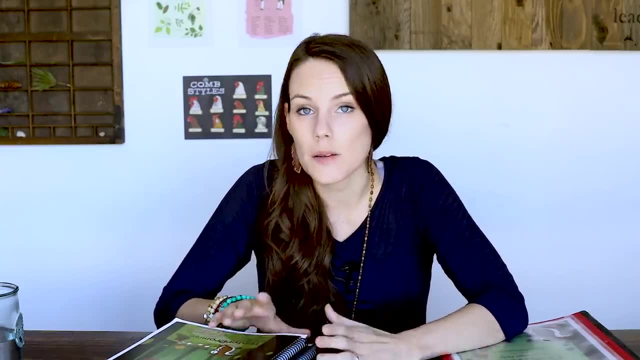 problem depending on you know what you feel about that as a secular homeschooler on. they have their, their reading. It's definitely it's more teacher intensive. It's something you need to sit and do with your child. It also can be a little bit overwhelming. 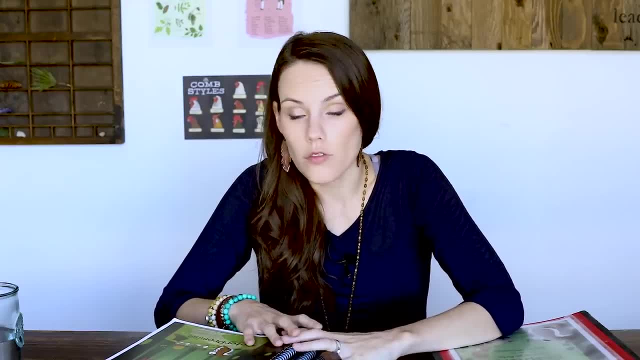 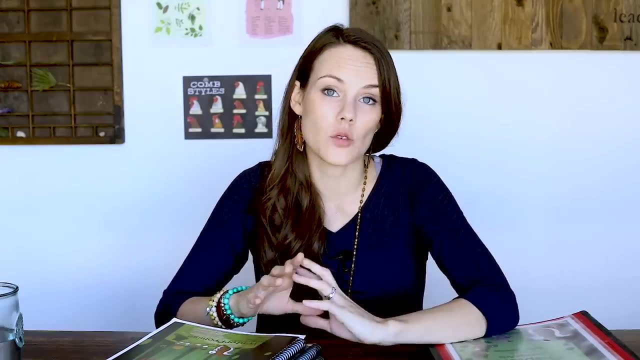 you know doing the amount of reading that is required for this, So I recommend breaking it up. If you're doing it with your child. in that way, you there's lots of adaptations, a way that you can use this that you can. 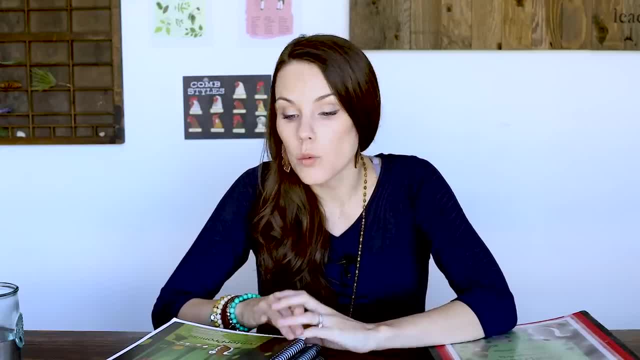 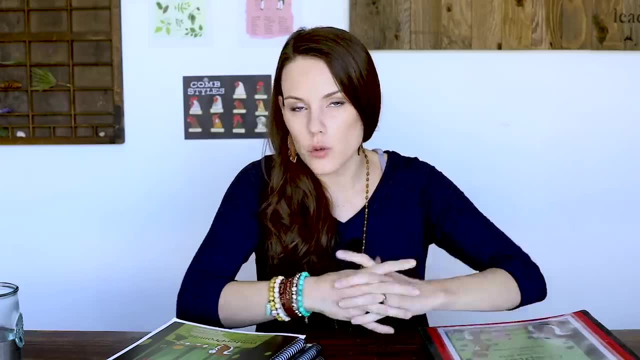 um, adapt it to work with your family. You would need one for each of your kids, depending on their various levels, And it is probably it's got some Charlotte Mason flair to it, but I would say that it is definitely more traditional in its approach. 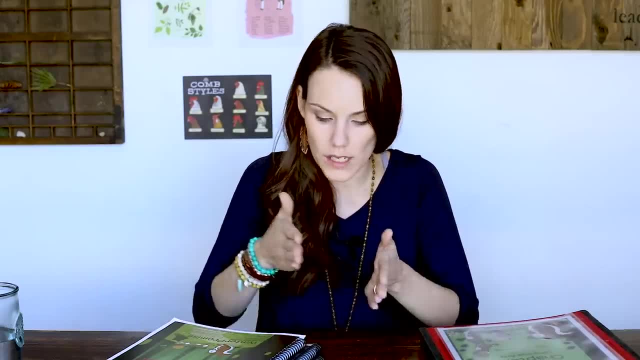 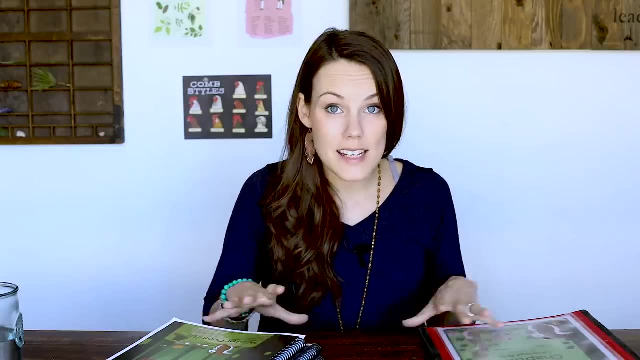 So if you are looking for something that is simple for you to follow and just read and do and follow the teacher guide, then this could be a really good fit for you. If you're looking for something that is either less intensive, this probably isn't it. 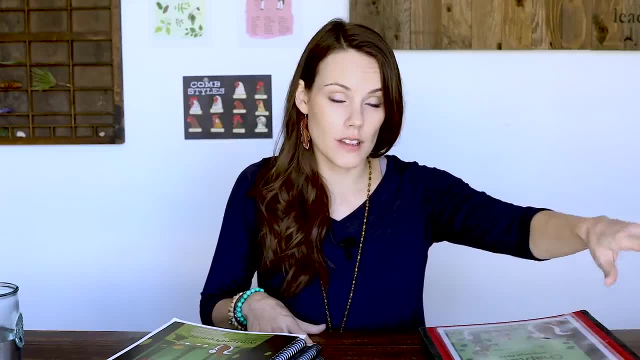 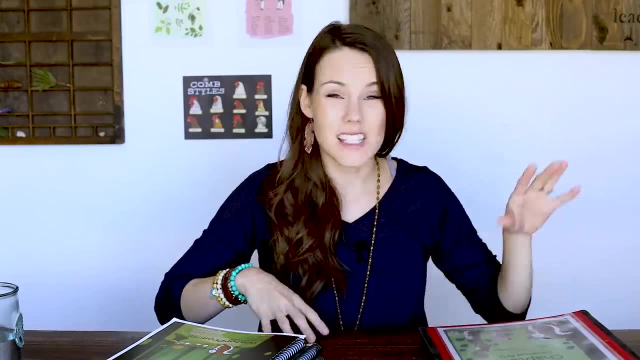 Less intensive is going to be a language of lessons for living education. If you're looking for something that is more independent, this isn't going to be it. You're going to want to find something like Christian light education that they can just do on their own. 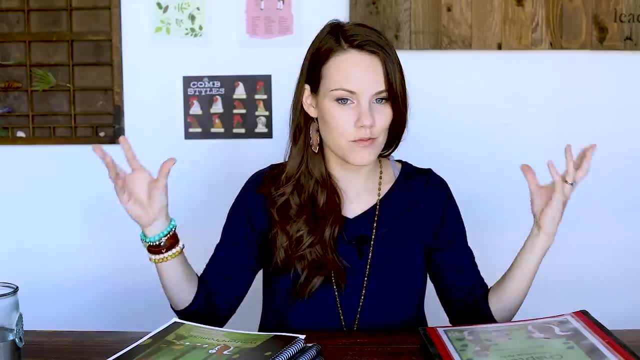 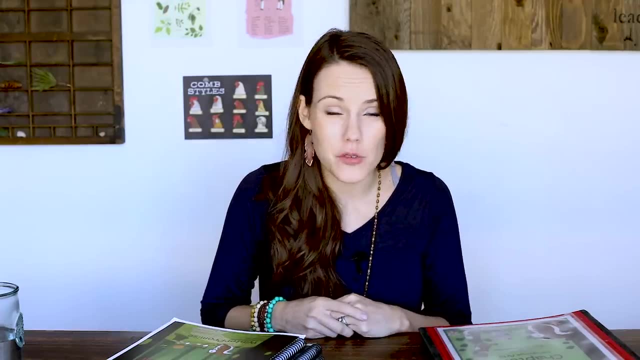 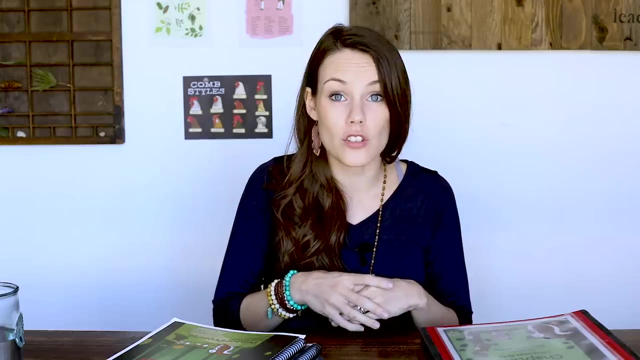 If you're looking for something that is just that, that education, that is just a feast of education, that Charlotte Mason philosophy, then you might want to look at something like my father's world, or you might want to, you know, look at some of these other ones, like brave writer, that are going to really be out of the box and are going to show you language arts in this. 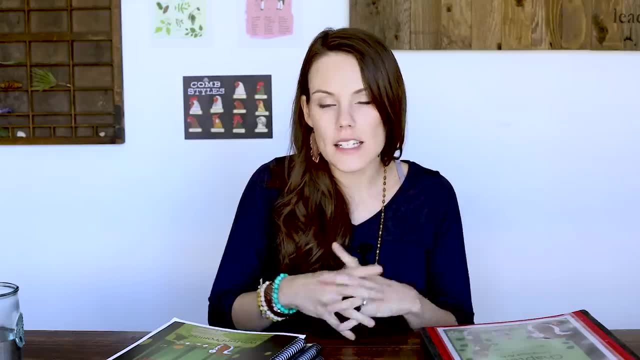 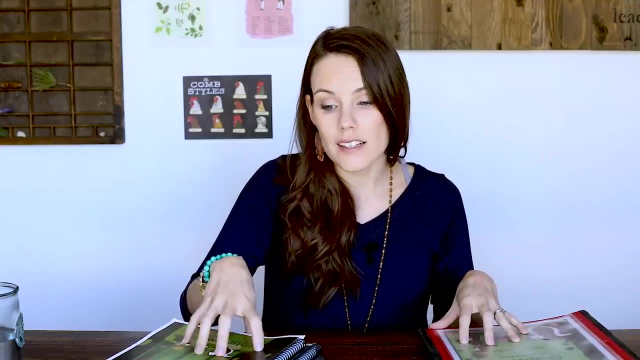 just just broad range, just different things to keep in mind. It's going to depend on you, on what you want as a family, on your own dynamics and your own goals. You need to keep in mind that this is more teacher intensive and more time intensive. 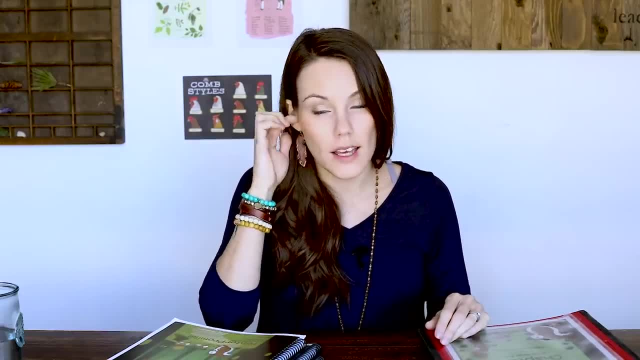 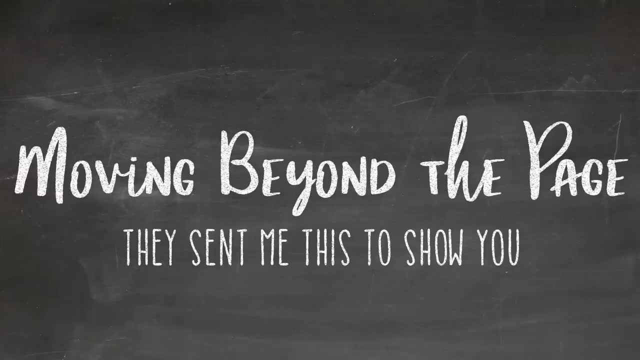 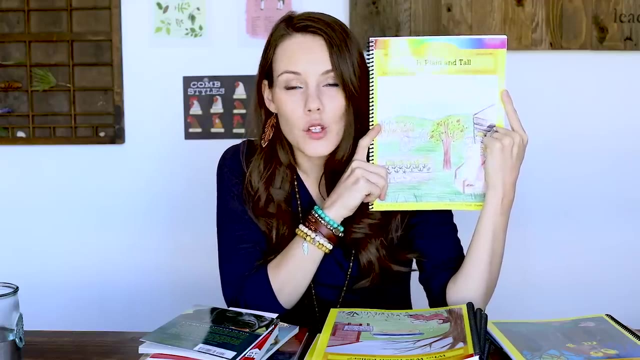 So just different things that you want to think about when you're considering language arts programs. The next one I'm going to show you is moving beyond the page. Now, moving beyond the page is incredibly unique, where I've shown you some that are Charlotte Mason inspired and some that are more traditional. 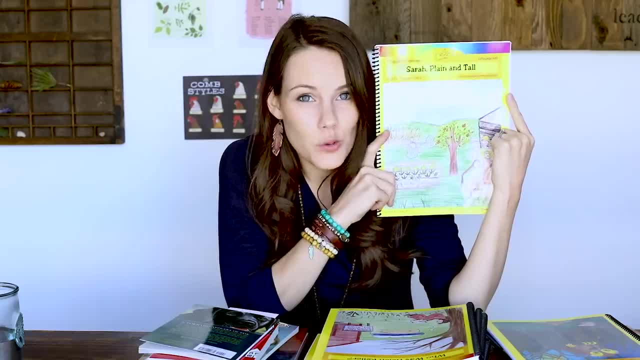 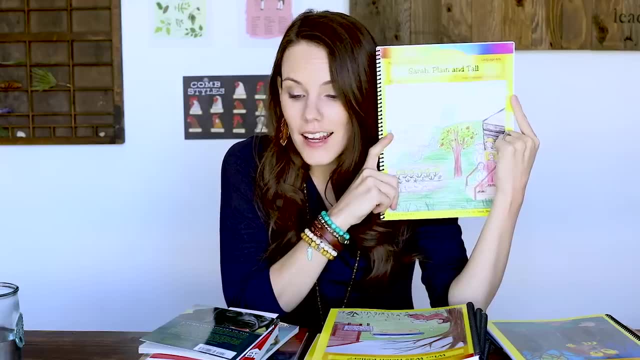 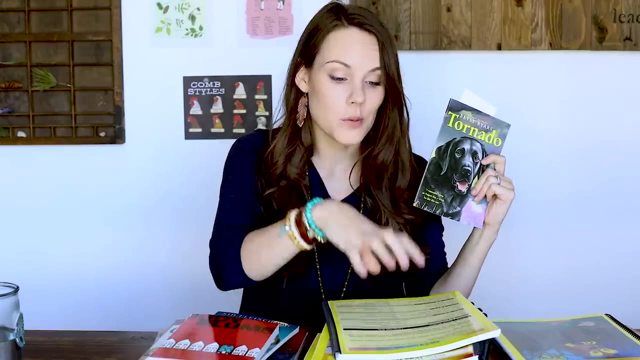 This is definitely unit study approach, which is incredibly unique. It is project based, which works fantastic for kinesthetic learners. It is hands-on, It's interesting and it is literature based, So they are going to be reading a book and then do it at that price point. You have to. you have to understand that there is so much included when you are, you are going to have to actually read through and you're going to have to prepare and you're going to have to learn. You're going to have to prepare and you're going to have to talk and explain and teach to your child. Week 36,. you're introducing the words. same thing They are doing. I can read it wordless. This is what the teaching looks like: Giving directions, dictionaries, a rubric. They're going to dictate a story And then here is their week 36,.